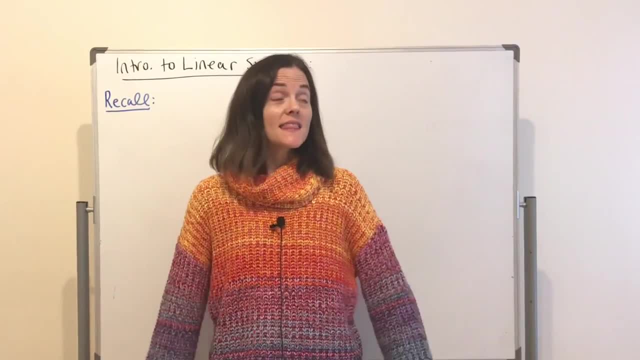 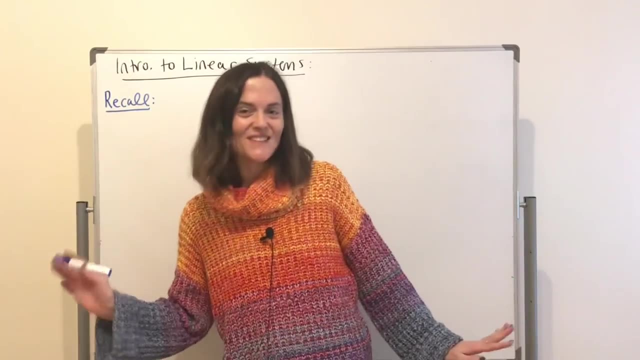 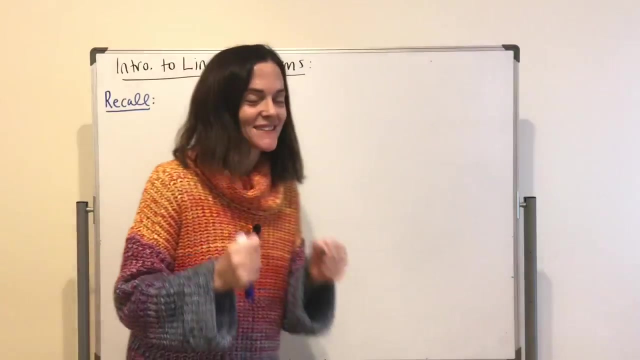 Welcome to Linear Algebra. This first day might be reviewed for you, and if it is fine. If it's not, that's fine too. okay, But I'm going to begin with the beginning so that we get a firm understanding to move ahead with the semester. So, first of all, what's a linear equation? 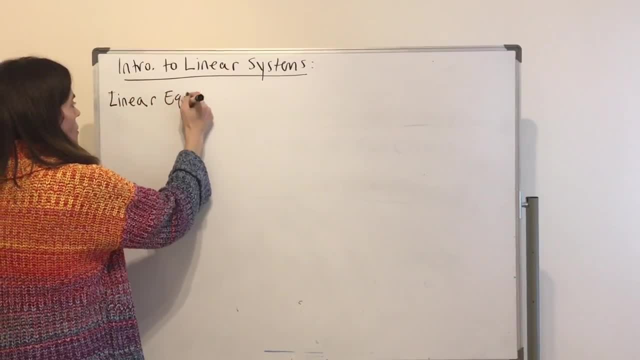 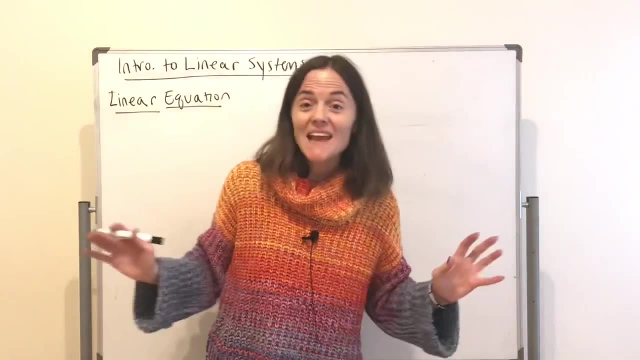 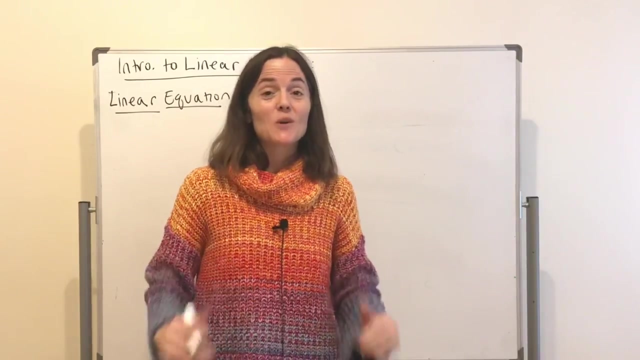 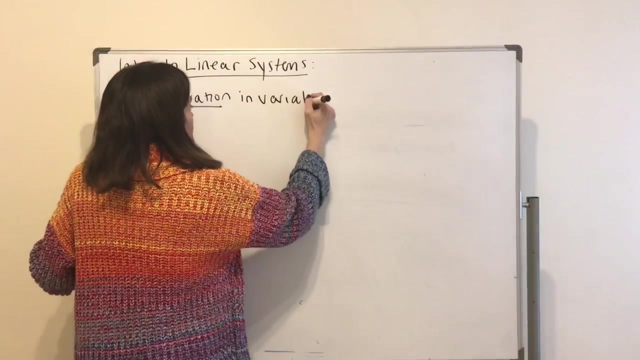 Well, generally, an equation and a function are two different things. An equation would be, for instance, setting a function equal to a number, or setting two functions equal. Those would be equations. A linear equation, let's say in the variables x1,, x2, x3, out to x. 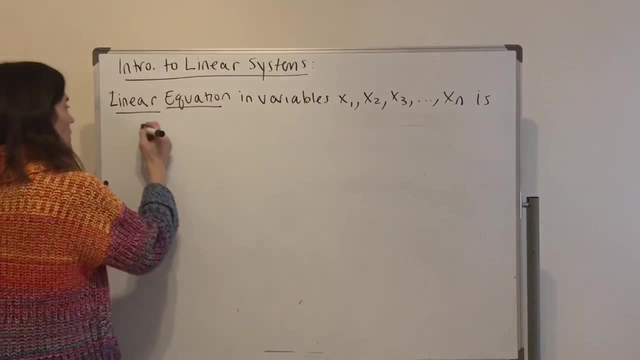 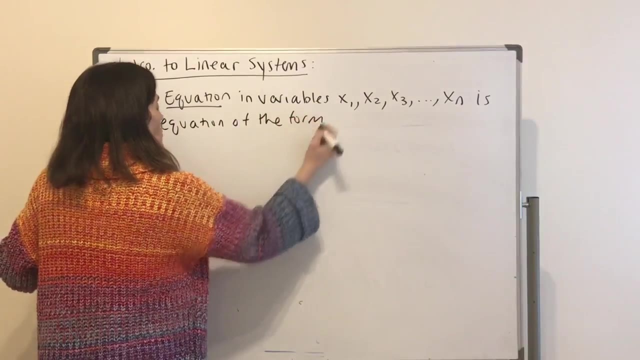 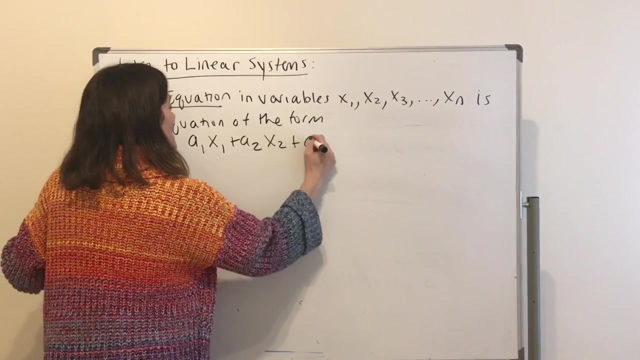 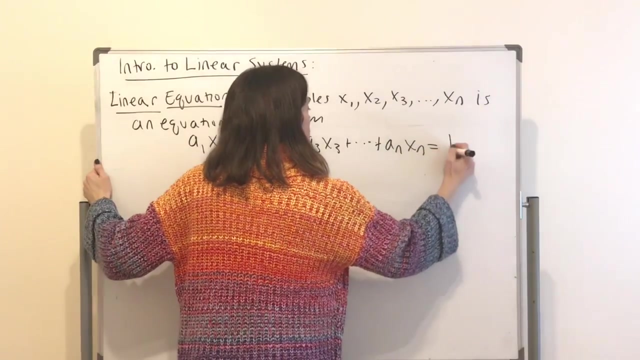 xn is an equation of the form. well, it looks like this: a1, x1 plus a2, x2 plus a3, x3, all the way out to an xn equals some b, okay, Where a1, x2 plus a3, x3, all the way out to 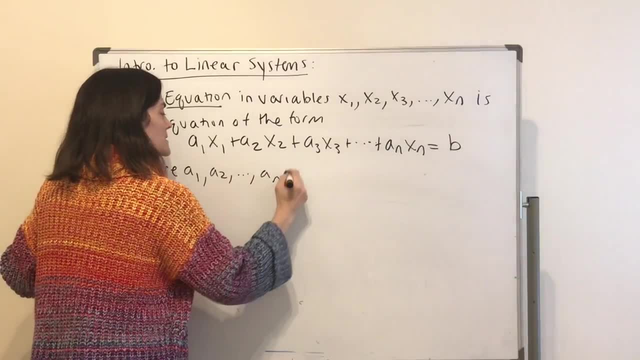 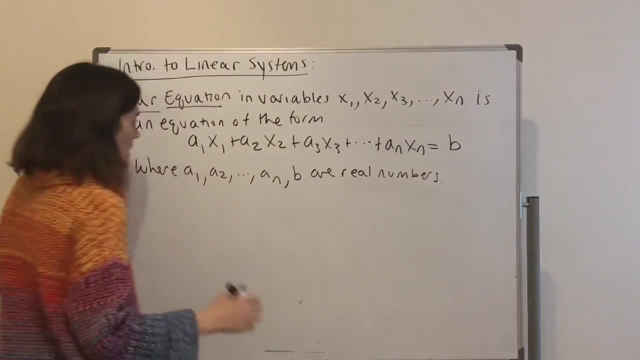 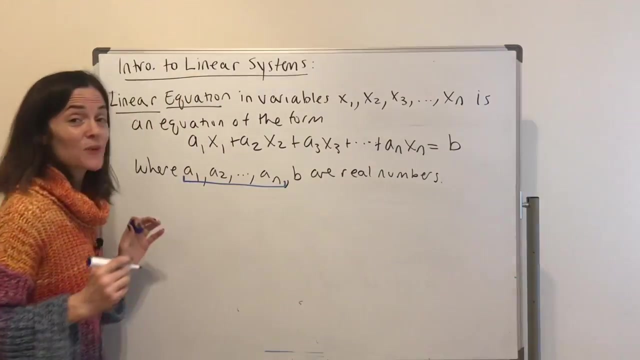 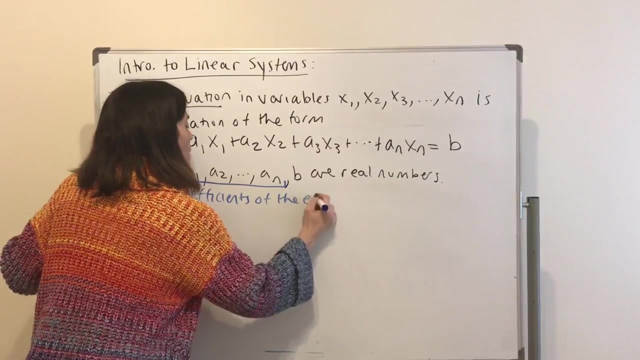 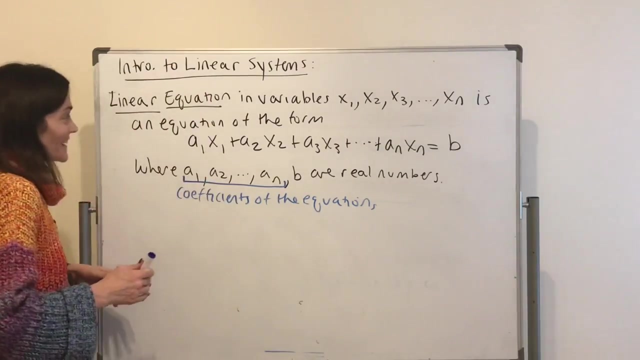 a1, a2, out to an and b are real numbers And these a1 through an are the coefficients of the equation And the variables. as I mentioned, they are written at the top. They are x1.. x1 to xn. Okay, this is a linear equation, If you see, if you see squares or if you saw. 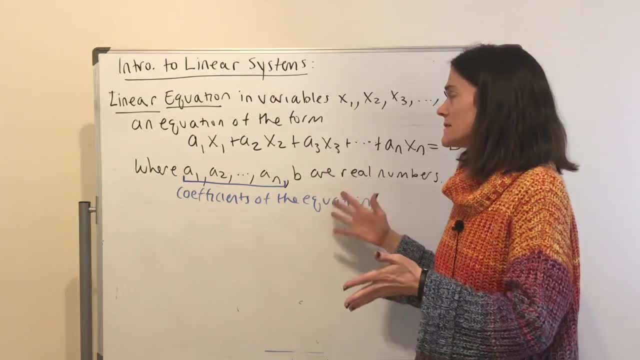 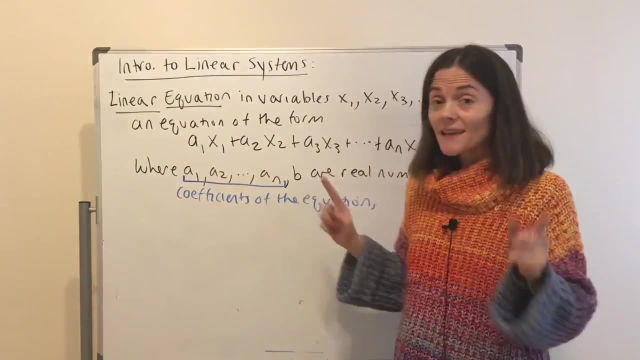 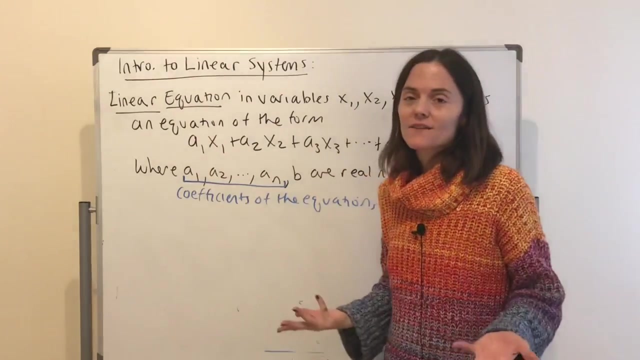 two things multiply together: if you had a term that was x1 times x3, not linear, or if you had the cosine of some term, not linear, okay, Linear means you have the variables with the power one and then times some coefficient in front. add it up like this: These are the 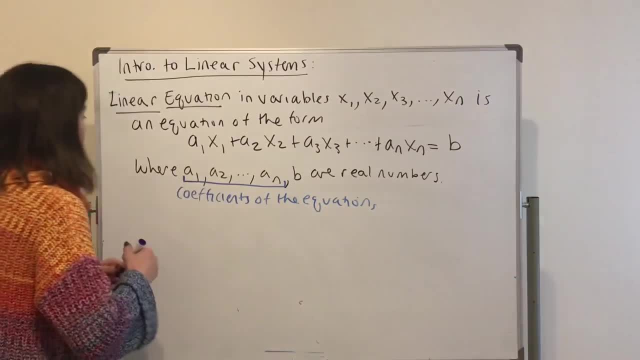 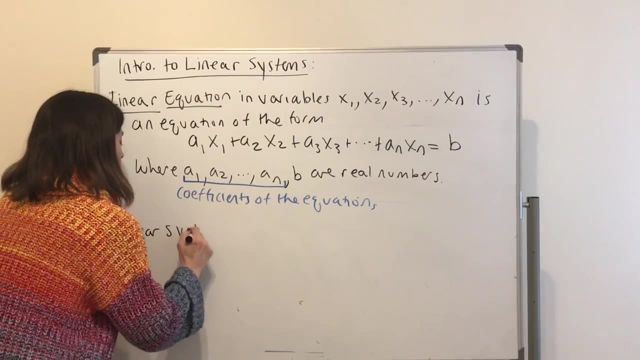 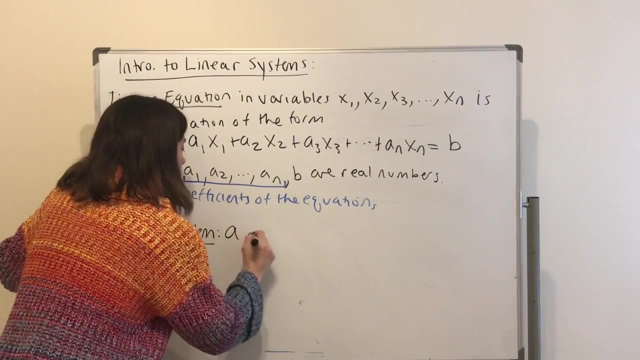 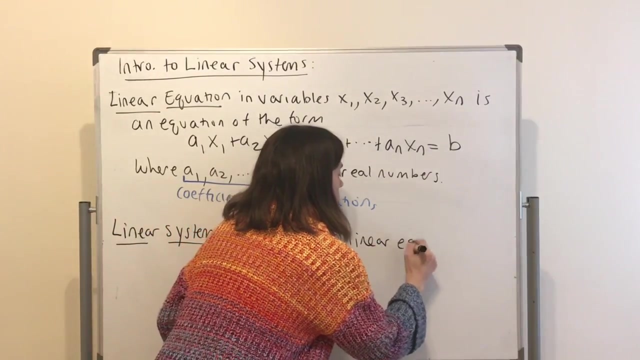 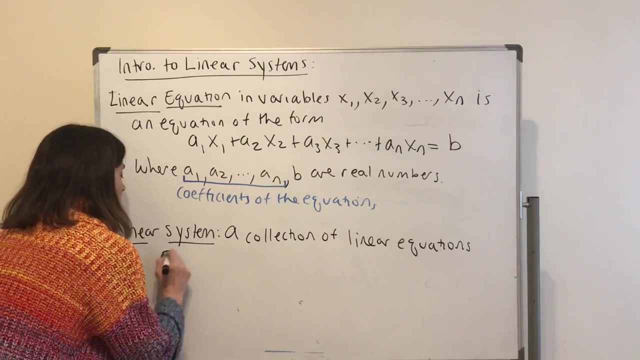 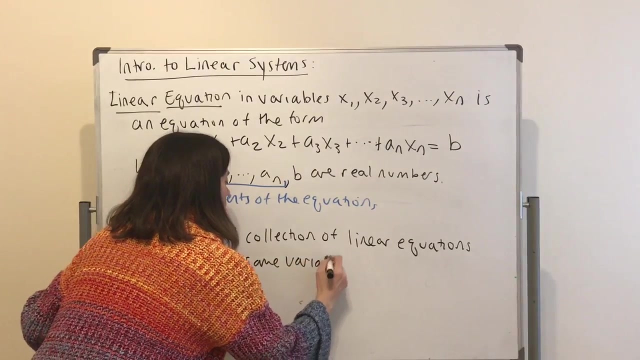 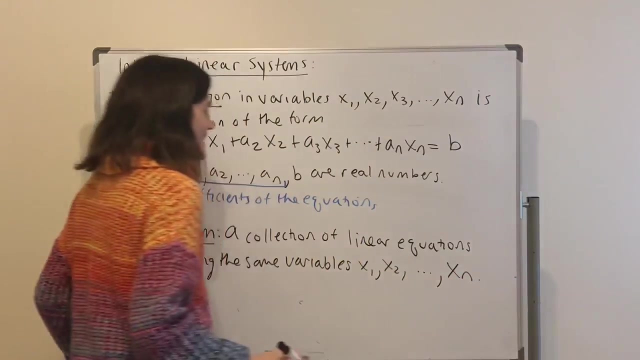 linear equations And then a linear system. this is a collection of linear equations that that have the same variables, And there's something interesting about this. if you sort of if you're out of the equation, you can do this before you solve the problem. 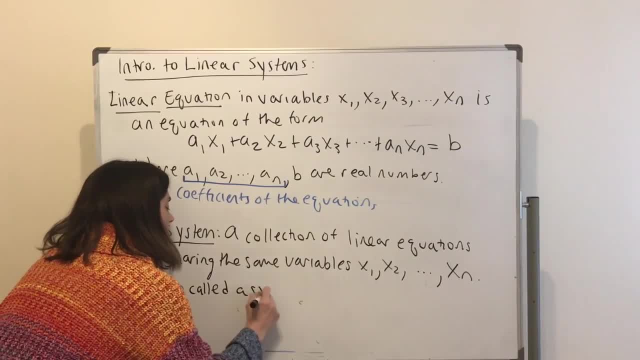 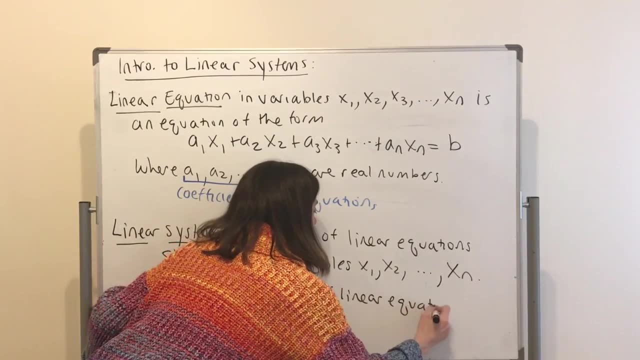 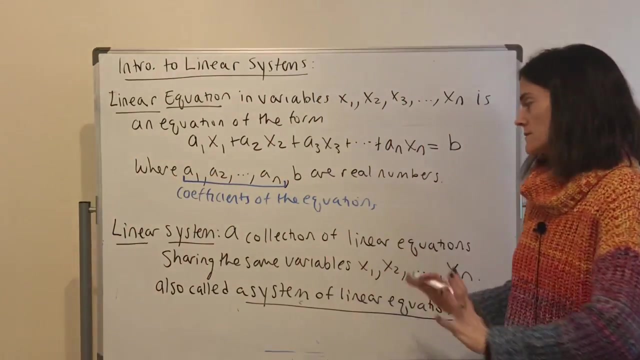 Assuming that the whole thing is linear. you can do this And you get the total 0. 0. 0. 0. 0. 0. 0.. and i will say right now this linear systems or system of linear equations, same thing. this: 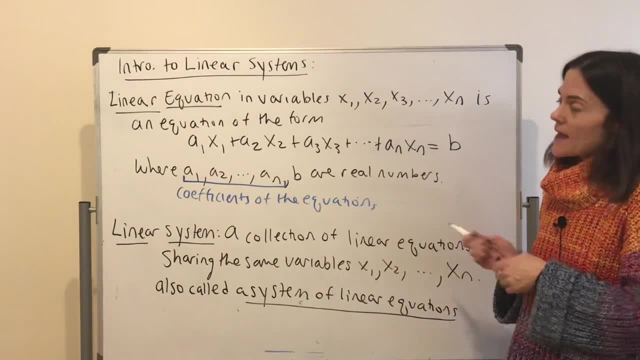 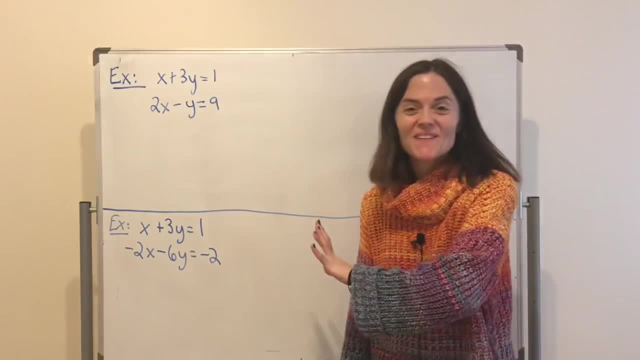 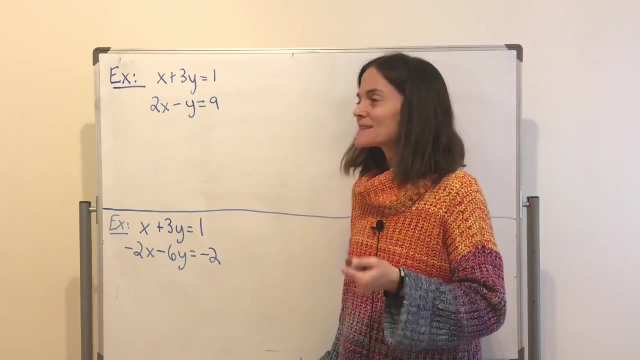 is the focus of this course. okay, well, let's do some examples. here are two linear systems. we will begin with um and they're both just with two variables, so i'm going to do three of them with two variables. then i will do some that have three variables. 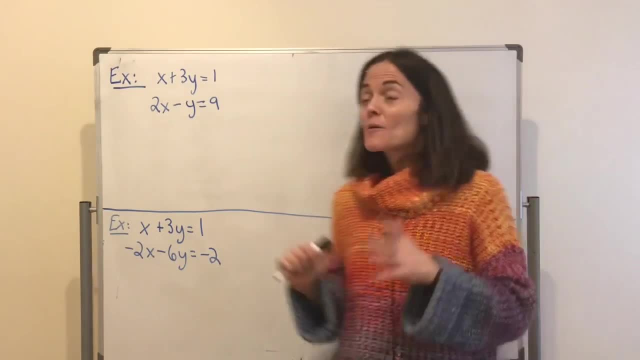 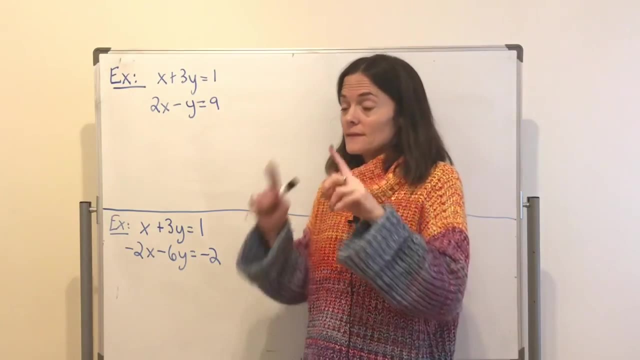 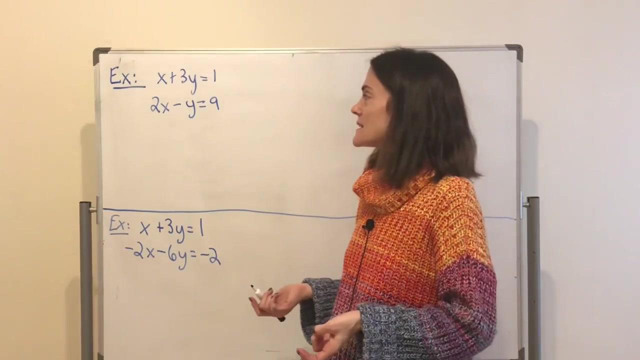 and uh, that's going to be the plan. okay, well, how would we find a solution? so a solution to something like this would be: uh, let's say, x comma y that satisfies both of these, or or maybe there's several x comma y that satisfies both of these. 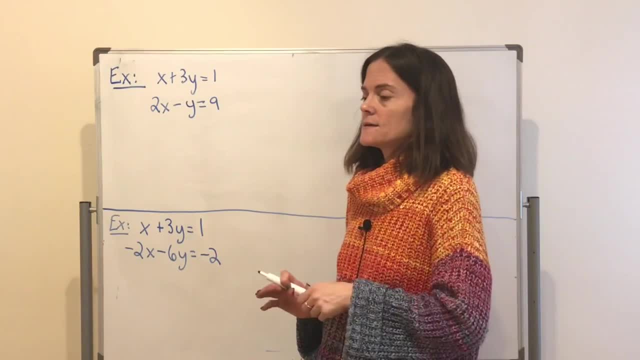 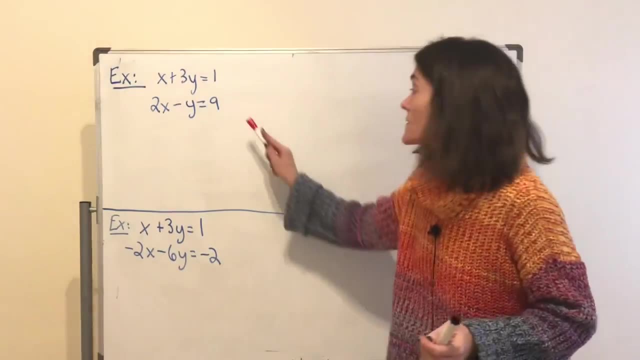 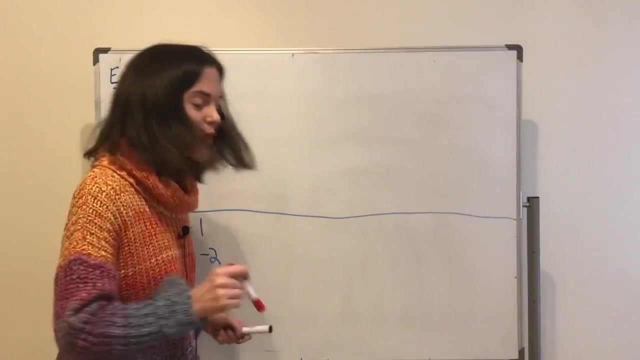 and how could we find this in a way that is um like methodical, because you will have even seen stuff like this in previous classes and you just sort of do your best, right, but we will find a methodical way to solve so that we could in theory have a seven by seven. we have seven equations, seven unknowns. 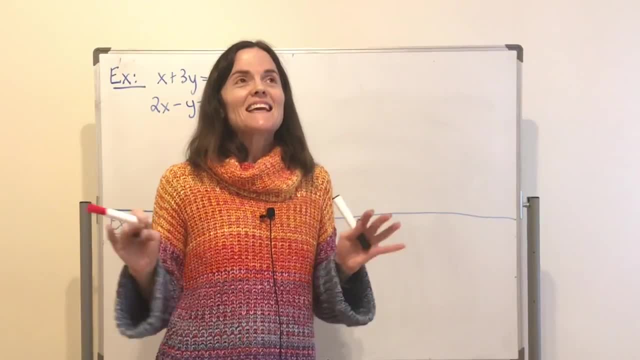 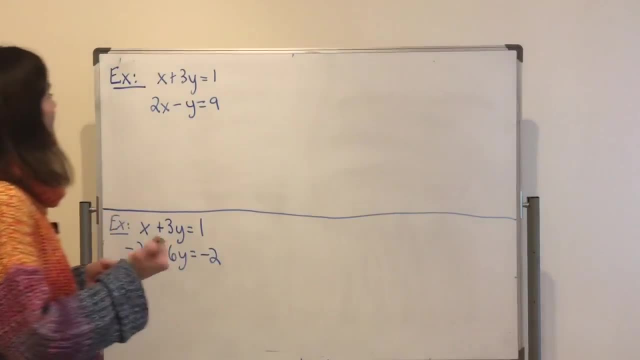 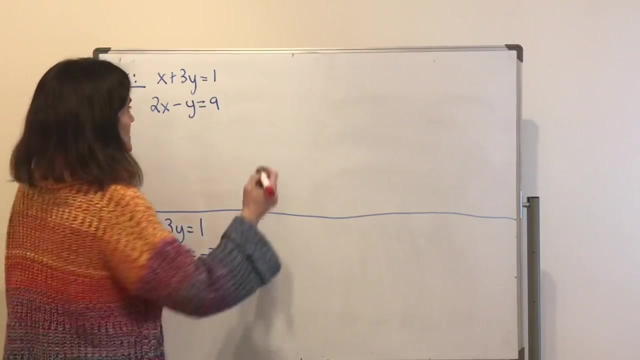 and we could go through our methodical order of doing things: find the solution if there is one, or the multiple solutions if there happen to be multiple. okay, so what could we do here, for example? well, let's take- and you will see my notation as we do- 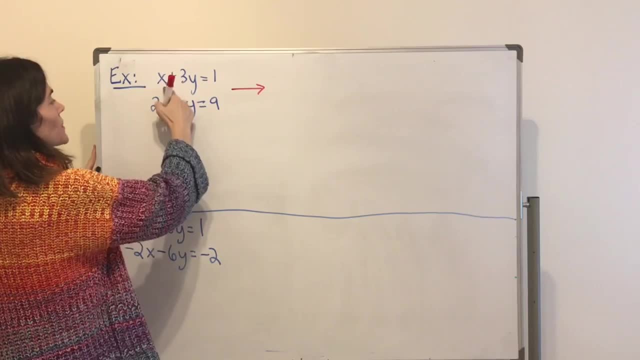 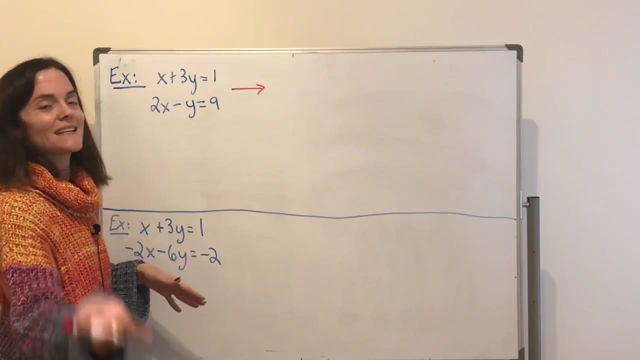 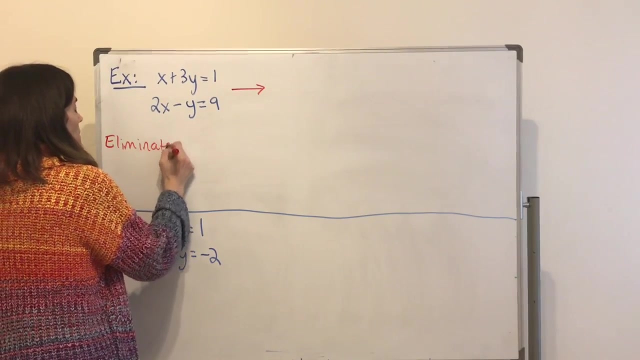 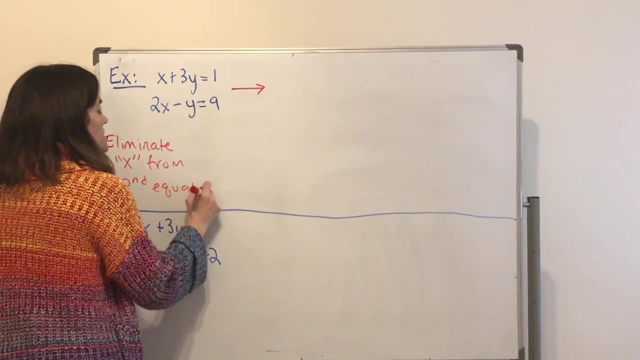 we are going to take this system and i'm going to multiply. one thing we can do with a big linear system is you can multiply one equation by a constant. add it to another. so what i'd like to do here is eliminate the x from the second equation. you notice, if i do this, i will be. 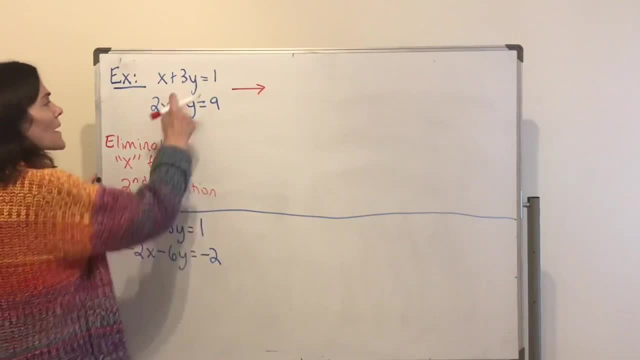 able to solve for y and then, once i have y, well, you can go through my notation and see which is y, and then you can go through the other equations and put it in the� back up here and find x. this is the goal, okay, and i mentioned- you've probably done this before. 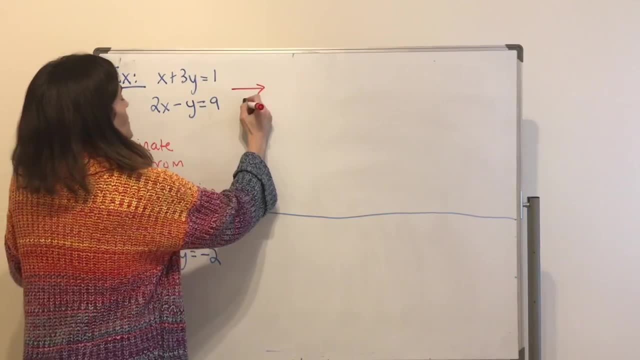 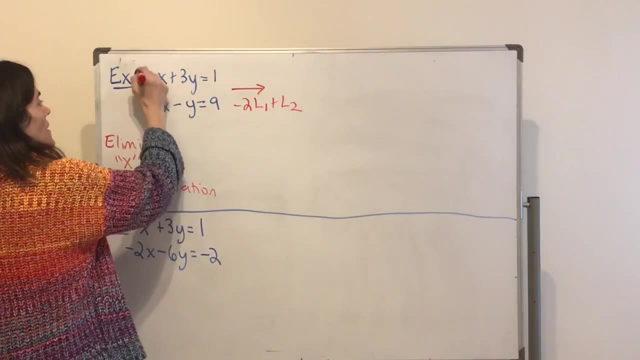 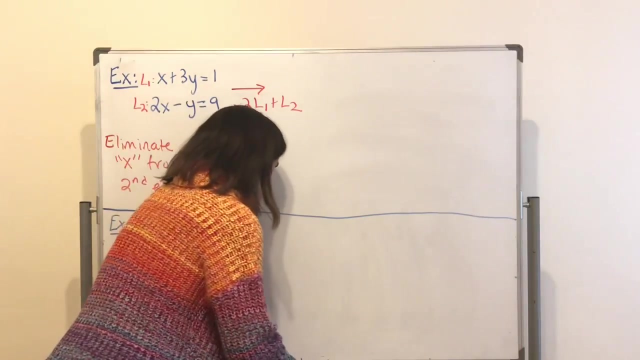 okay, well, i'm going to multiply. so i'm going to take negative two times the first line and add it to the second line. so here my notation here. this is line one. this is line two, like this: okay, well, what happens when i do this? i have not altered line one, it's still x plus three. y is one line. 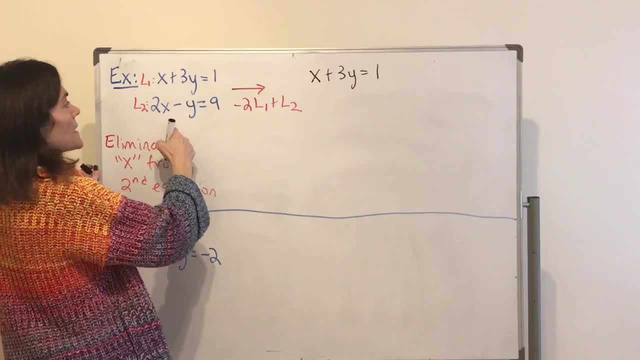 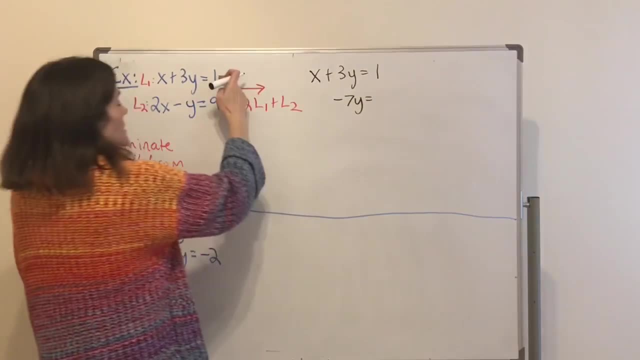 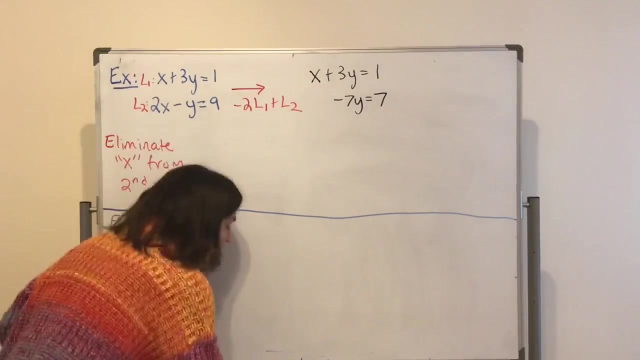 two. well, take negative two times this line, add it here. so the first equation is zero, and then i get negative seven. y is negative two times this plus this, you get seven. now what's another thing you can do? of course, in your mind you're thinking: okay, i see it, y is. 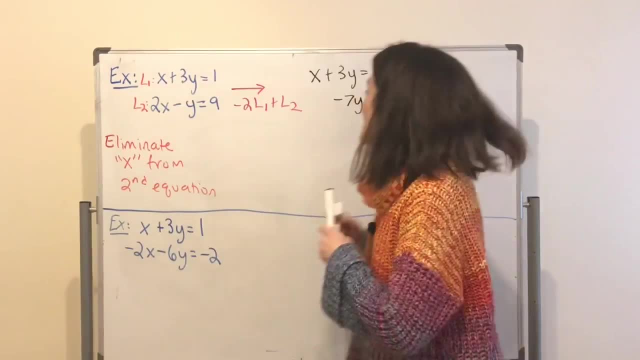 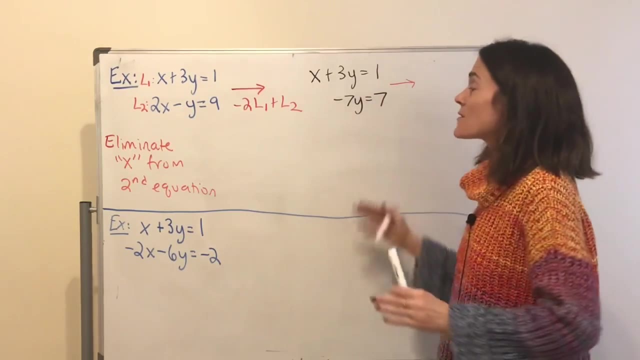 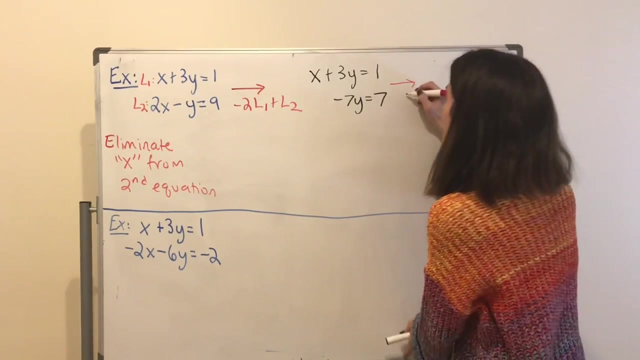 negative one, but i'm trying to teach the operations we can do. well, from here we can take. so one thing is you take a multiple of one line, add it to another. Another thing you could do is just multiply through by a whole line, by a constant. So I will take negative 1 7th times: L2.. Okay, 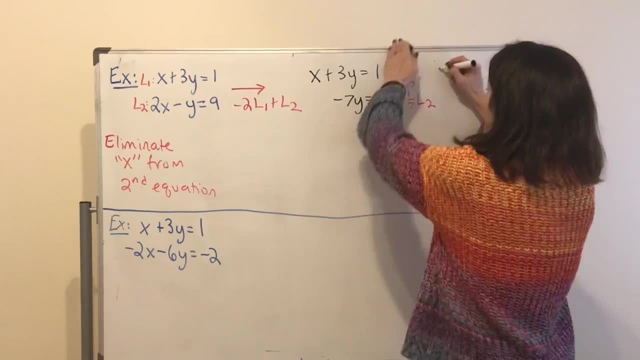 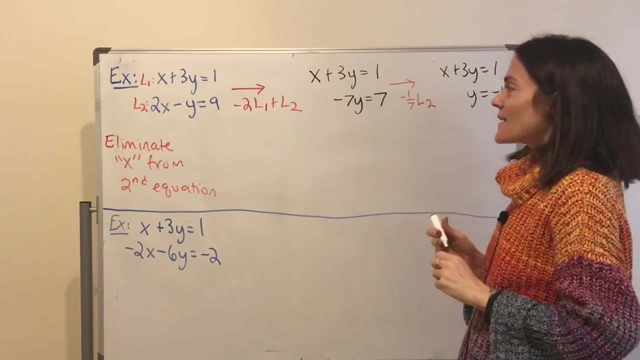 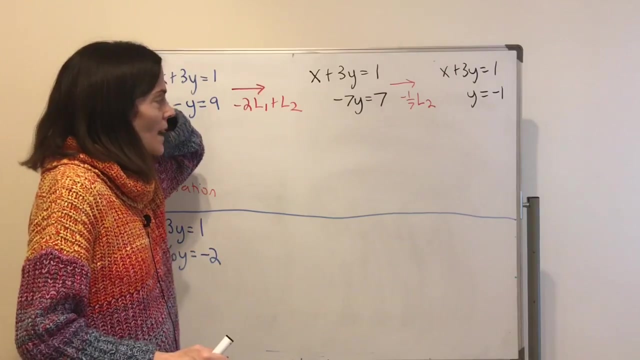 this is what I'm doing here. Then I get x plus 3y is 1 and I get y is negative 1.. Okay, so far, so good. And you notice, by eliminating the x, this is our goal- We have. okay, solve for y. 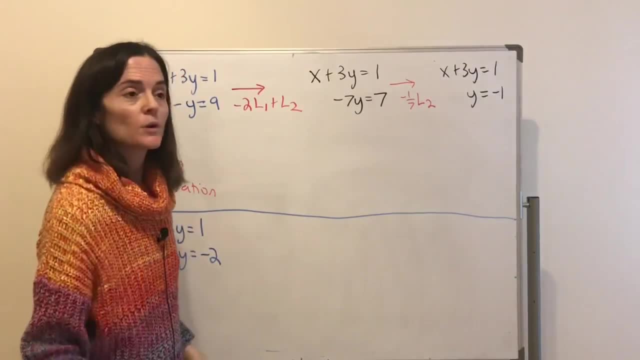 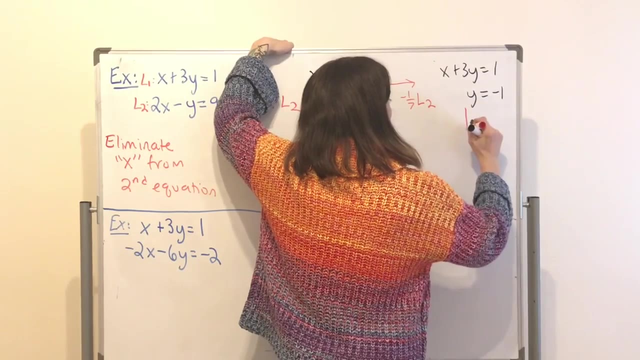 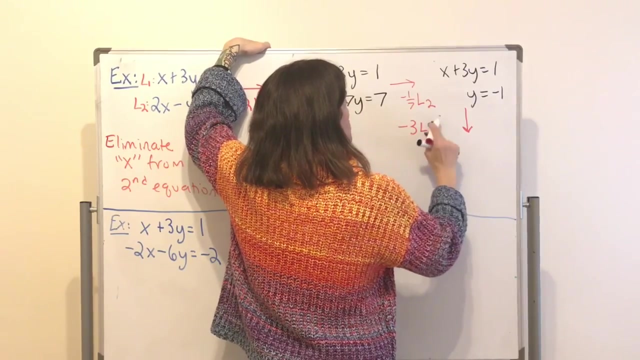 I could do the exact same type of operations. Take a multiple of one line, add it to another. In this situation, I would be taking- I will move down here- I would be taking um minus 3, L1, 2, excuse me, add it to L1.. Right So. 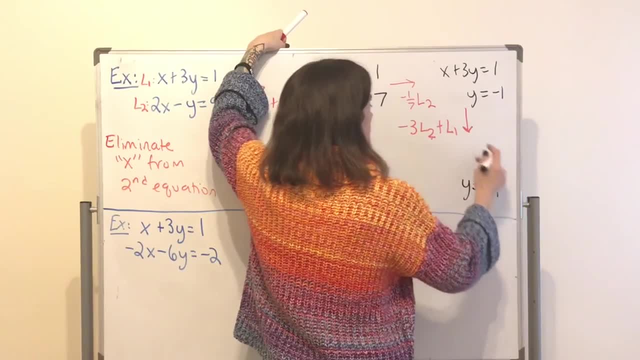 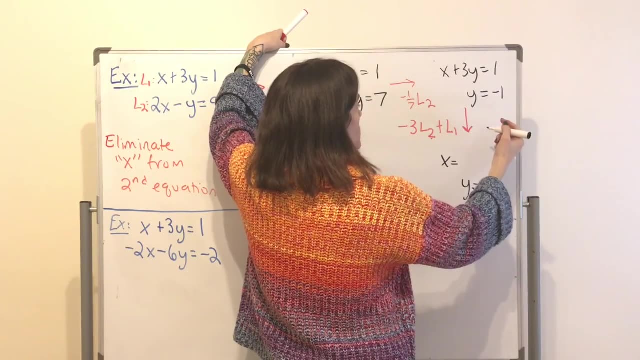 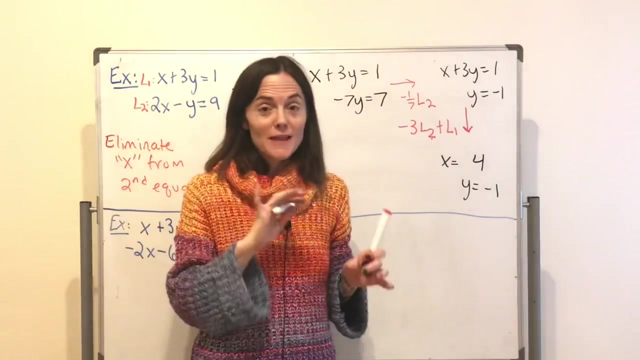 what happened was that this line 2 remained this, And then, when I take minus 3 here, we got x equals these two will cancel, And then we get 4.. Okay, So the only thing I've done, I've multiplied through by a line, by a constant, taken a multiple of one line. 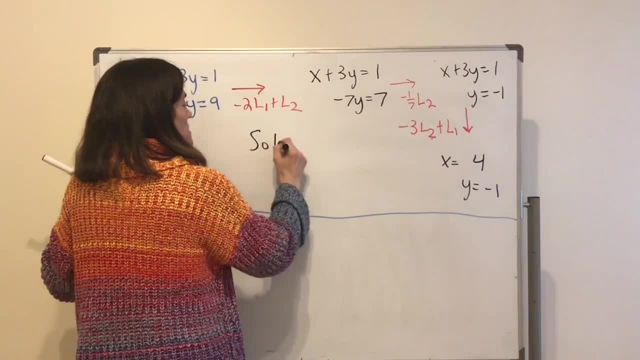 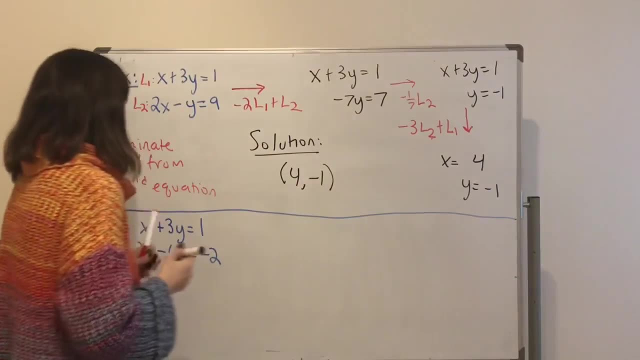 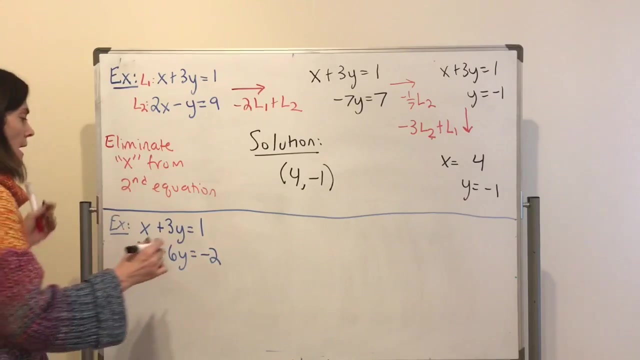 added it to another and I have the solution. So we have the solution here. It is 4.. Comma minus 1.. Okay, Well, let's do the same thing here In this example. again, it's a linear system. We have two variables. I'm going to do the exact same strategy. 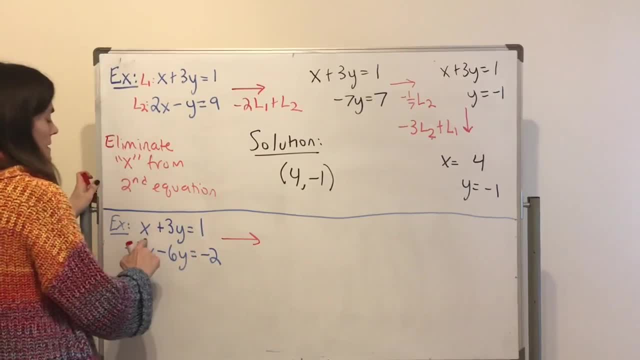 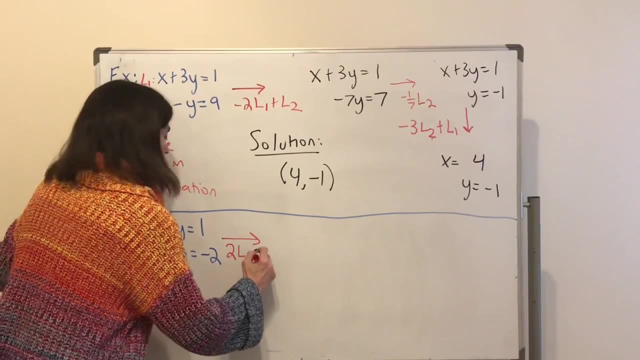 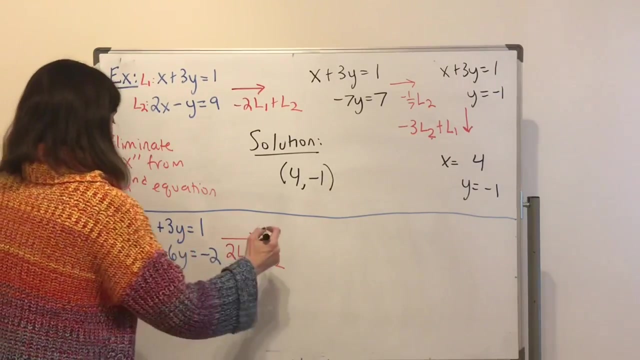 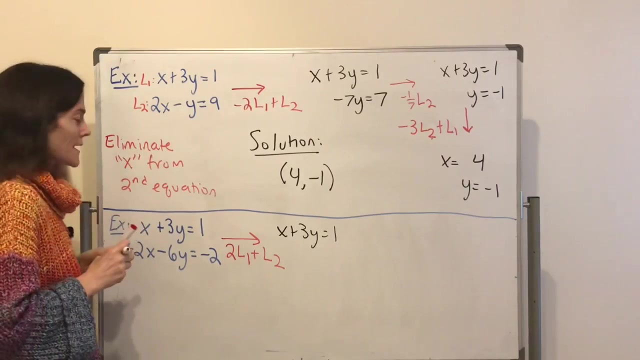 where I take. let's see, I want to eliminate the x. Okay, So I'm going to take two times line 1, add it to line 2.. My line 1 remains the same. It is x plus 3y is 1.. Well, you notice my line 1 was the same in both of these. It's fine. 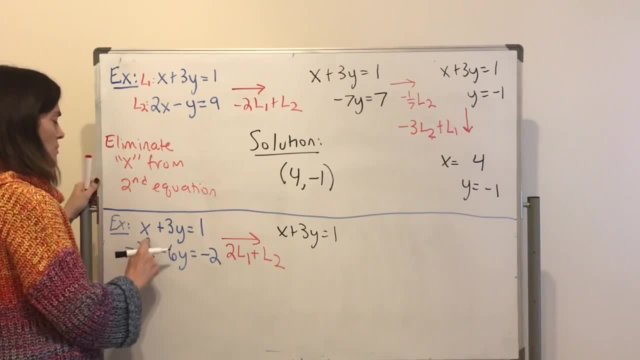 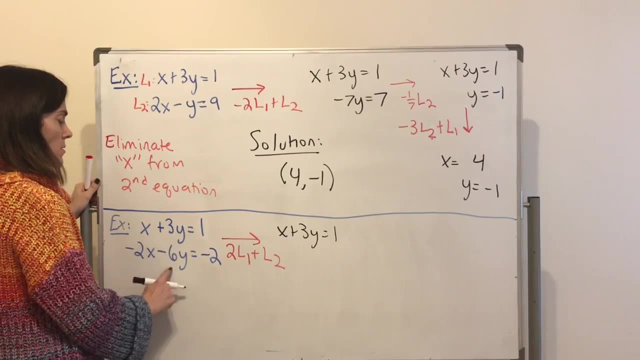 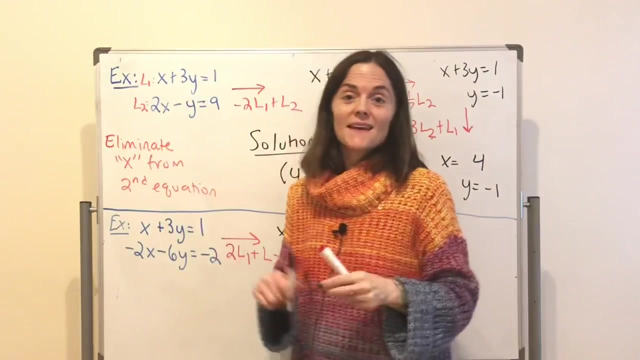 They're still two different examples. Now, what happens when you take two times this and add it to this? Um well, I get 0, 0, 0. So I get 0 equals 0. Well, okay, What you see here is in this example. 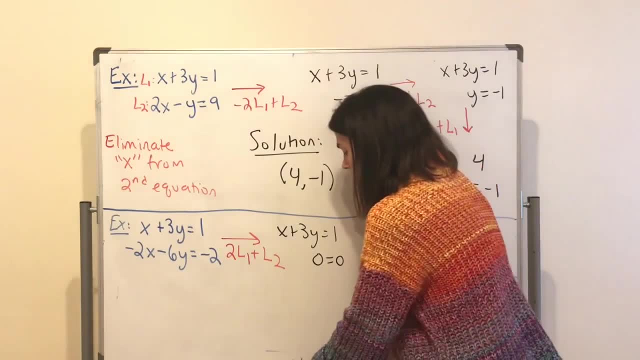 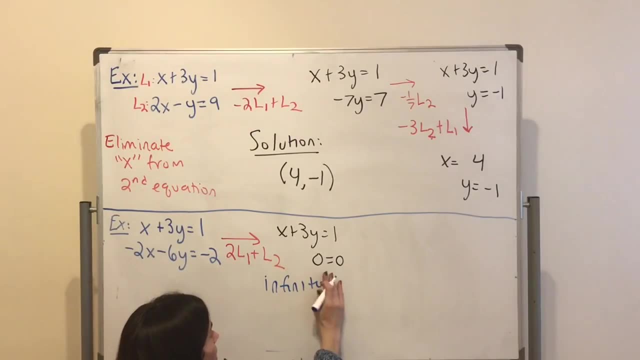 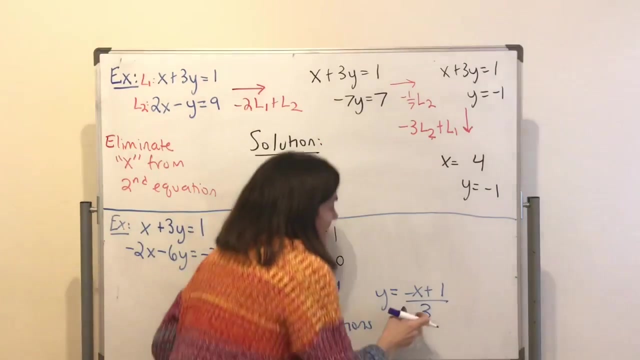 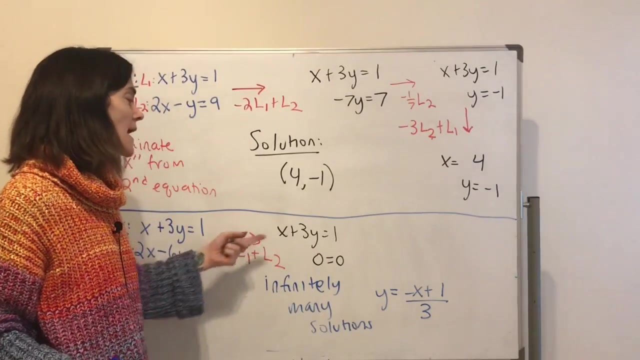 we have infinitely many solutions. Maybe I'll write this below: We have infinitely, infinitely many solutions. In fact, our solutions. you see, this is a line with slope negative, a third intercept, a third like this, And every single point on this line is a solution to. 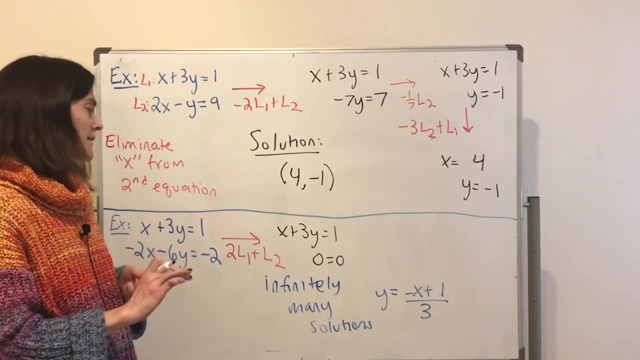 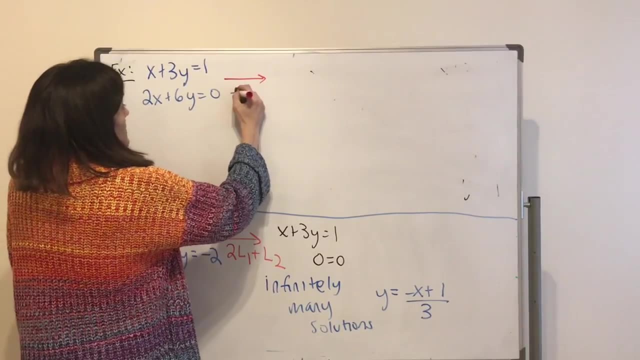 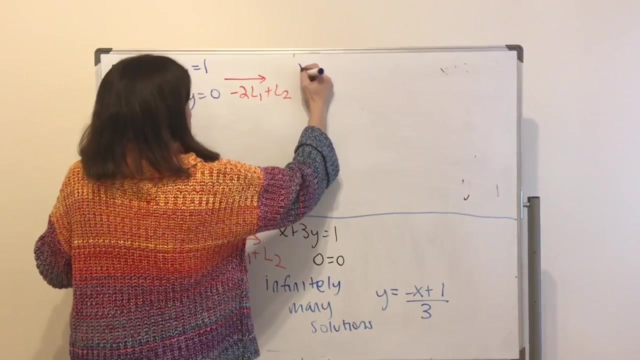 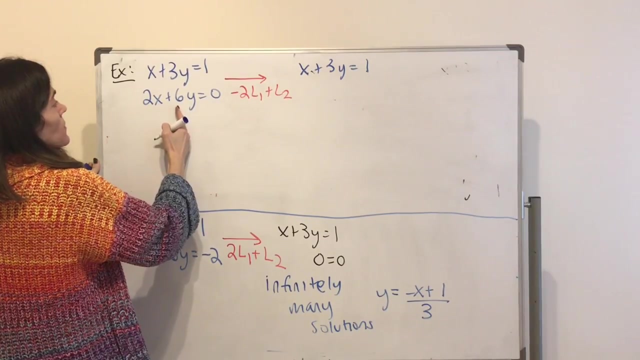 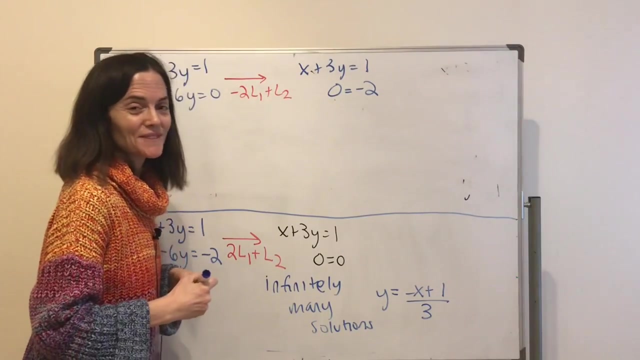 this linear system. We have infinitely many. Okay, Well, let's do one more quickly. Okay, Here we go. We're going to take minus two L1, add it to L2.. What happens? Line 1 remains the same, But then here, 0, this adds 0.. 0 is negative 2.. That's never true, Right? 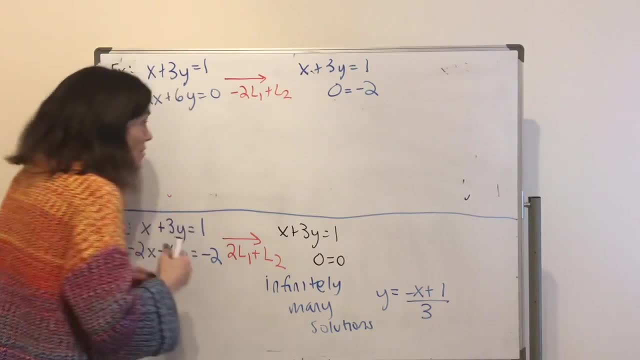 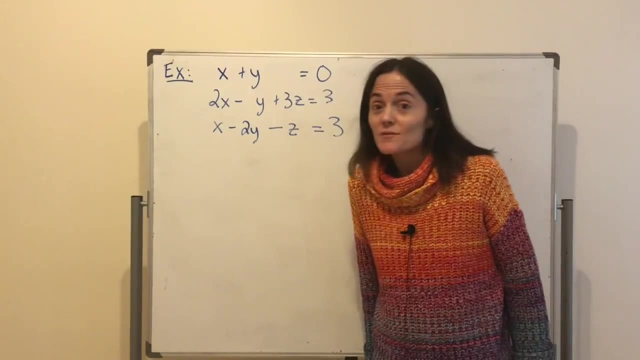 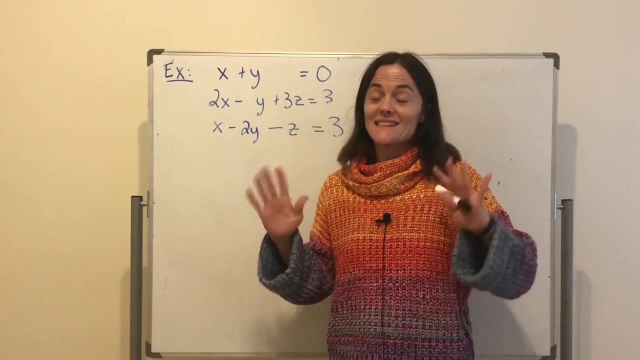 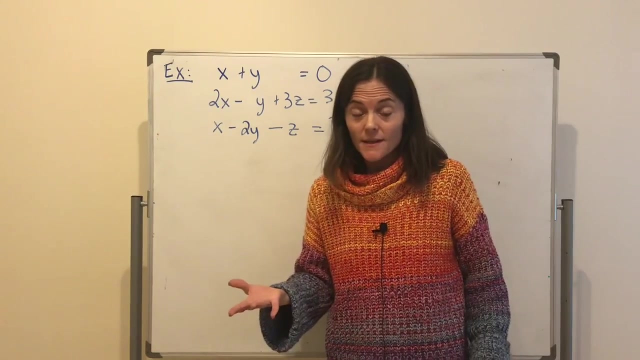 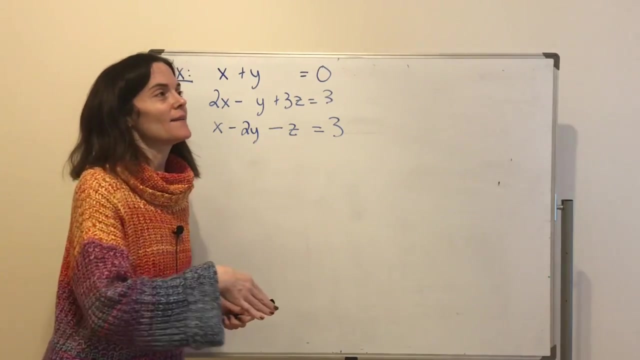 Never. What this says is: we have no solutions. now we have three equations, three unknowns, this linear system. one reason that i i went slowly per se through two equations and two unknowns was to get, as i mentioned, this method down. so, for example, what are we going to do? well, i'm going to multiply. um, let's say, add a multiple. 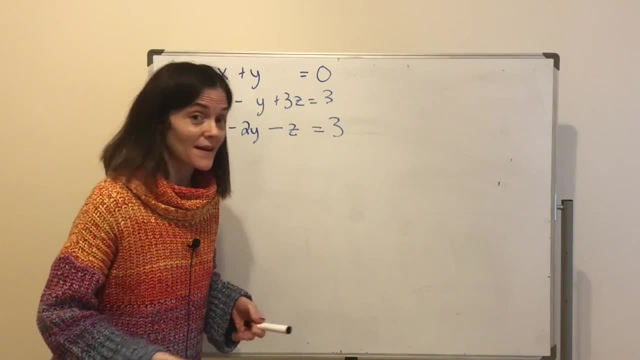 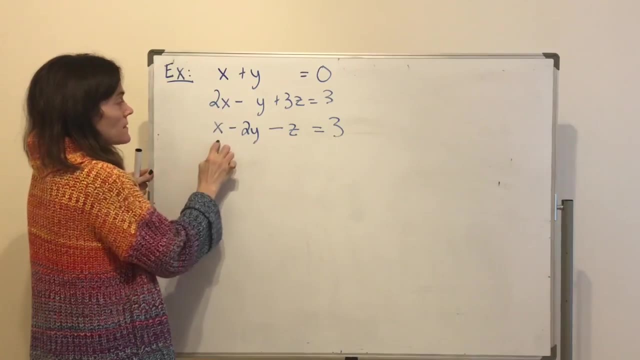 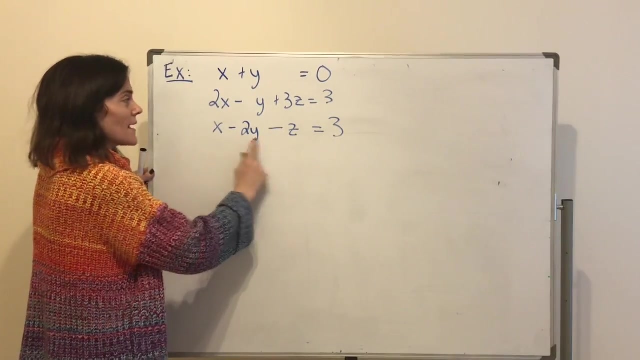 of one row to another or multiply one row through by a constant. but my strategy will be: first i'm going to eliminate the x's in this row in this row, okay, and then i'll subsequently eliminate the y. here i will solve for z and then i can sort of backtrack, solve for y. 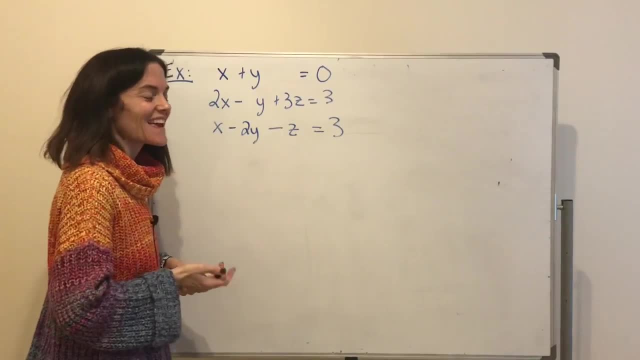 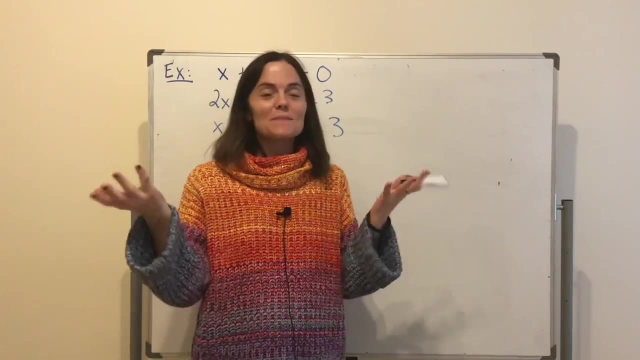 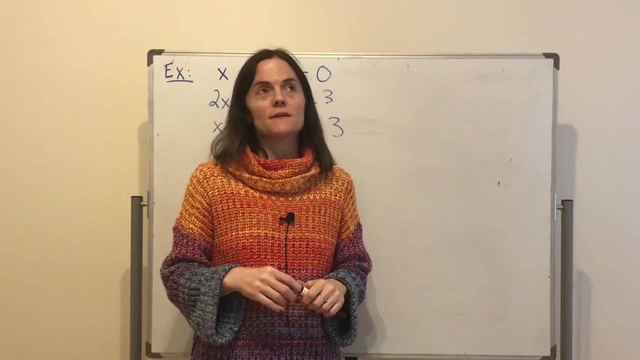 solve for x like this. we will see. okay, and this, this is a methodical way, as i would like to was saying, Of course, with two equations, two unknowns. sometimes you would just solve for y in terms of x, Stick it in the second equation, right, And that works until you start having. 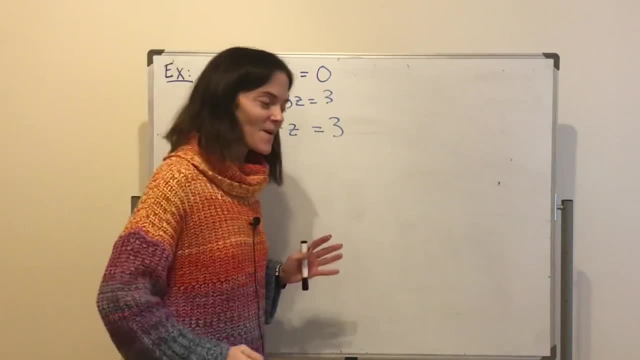 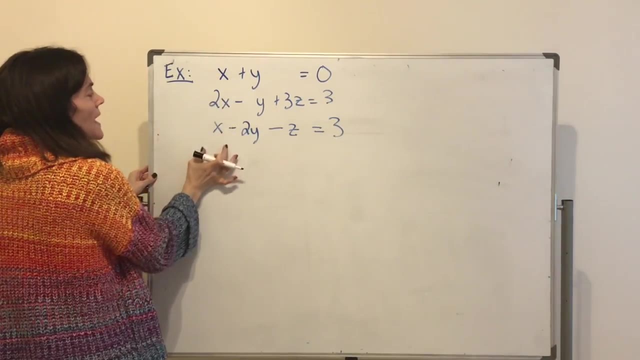 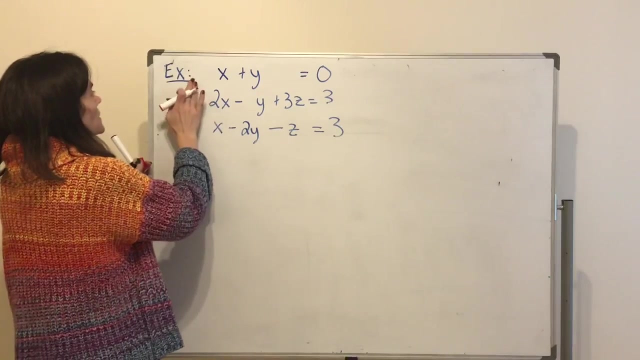 larger linear systems. So we are really focused on the steps. Okay so here, what I mentioned I would do: we will eliminate the x in the second and third line And, just like we started last time, when you sort of see the steps written out, let's see, this one will be L1, L2, L3.. Okay so, 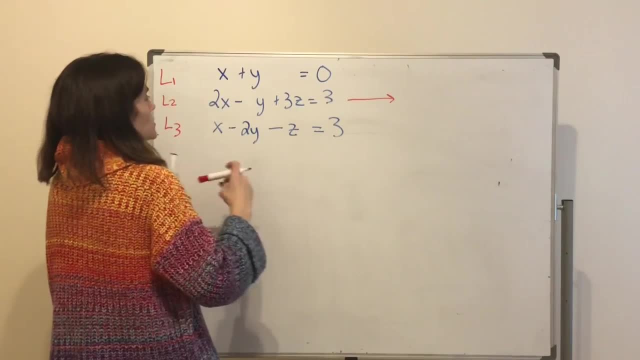 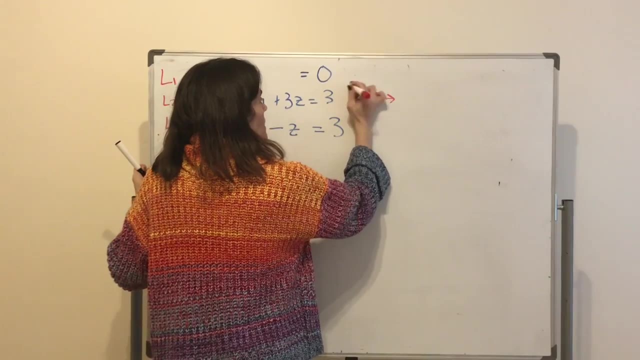 the first thing I'm going to do is I'm going to do two things at the same time. First, I'm going to take negative 2L1, add it to L2.. Negative 2L1 plus L2.. And I will take, look, just minus L1. 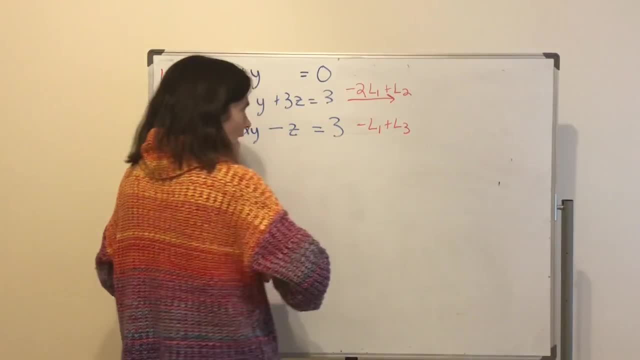 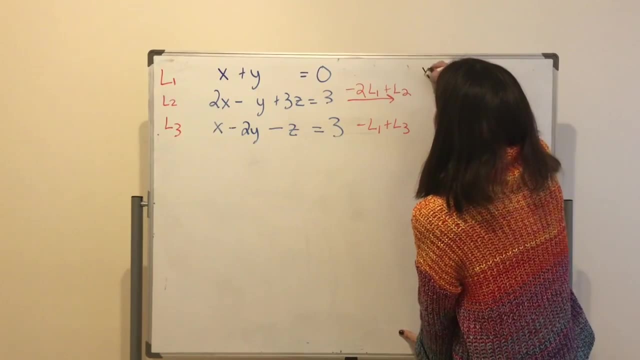 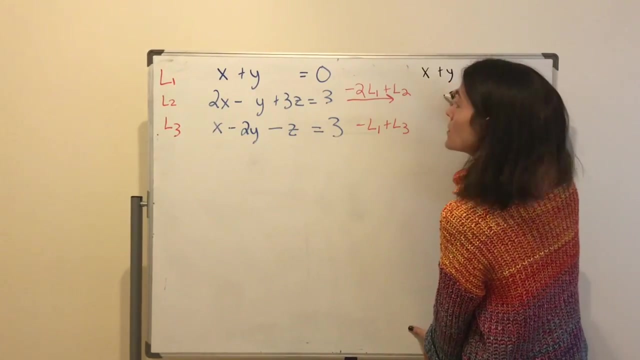 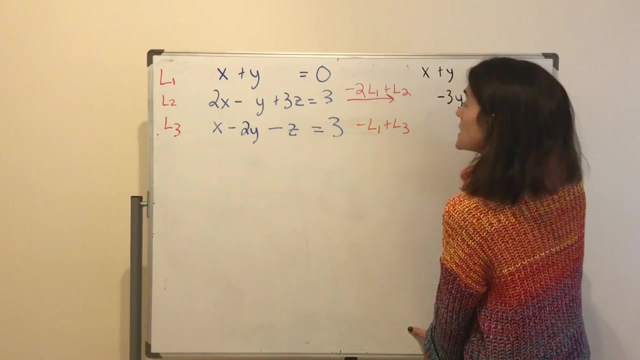 plus L3.. Okay, and then I will recopy What I get when I perform these operations. So I have: the first line is still x plus y is 0. And then here I'm going to get 0. And then I will have, let's see, minus 3y plus 3z is 3.. This is. 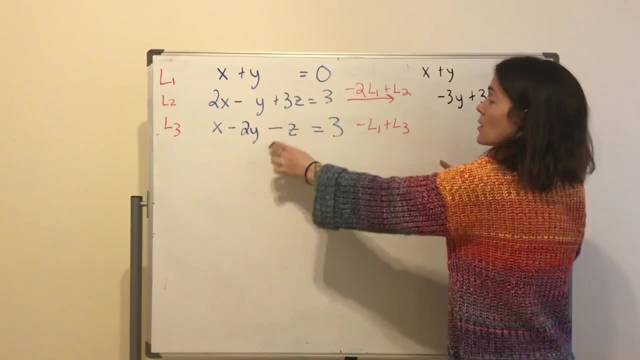 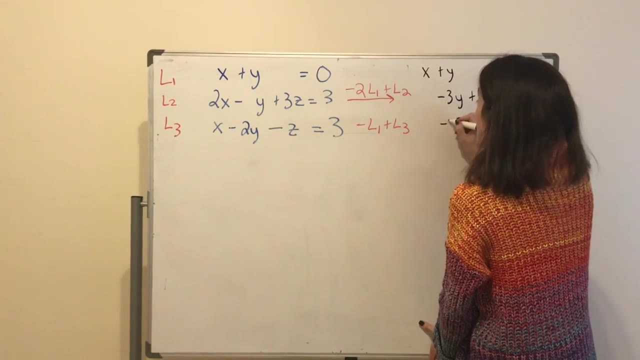 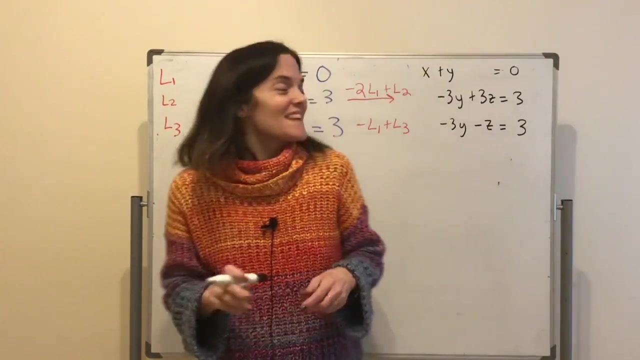 by doing this operation. And finally, when I take minus L1, plus L3, I'm adding it to here- I get 0.. Well, this is 0.. I get negative: 3y minus z is 3.. Okay, Now, as I mentioned, now I want to just 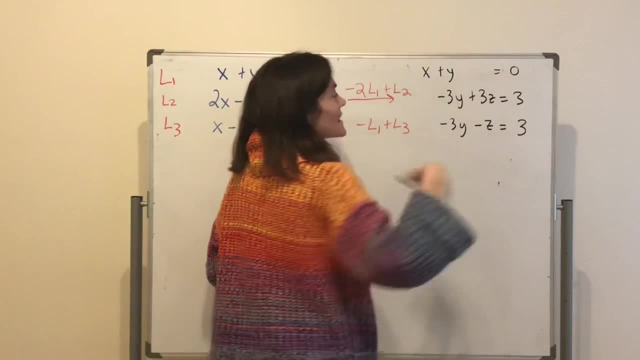 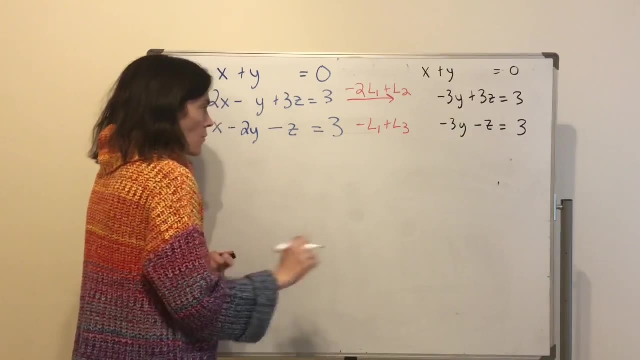 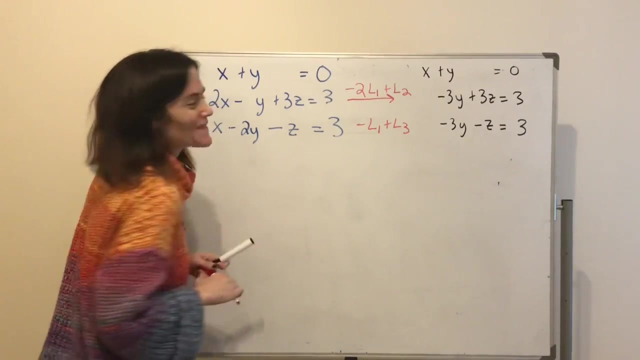 look here Now. well, this little piece, if you think about it, it's two equations, two unknowns. but I want to eliminate the y here, And so maybe, instead of going down, I will just move. It's difficult to do. 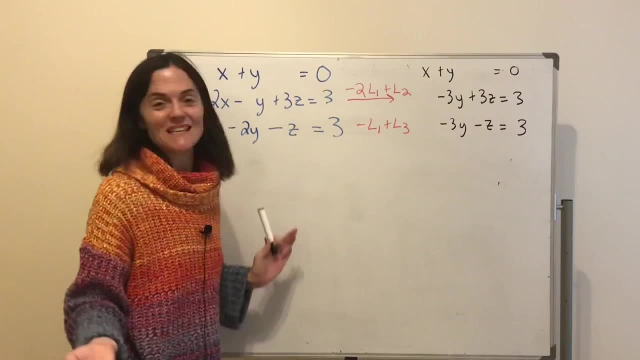 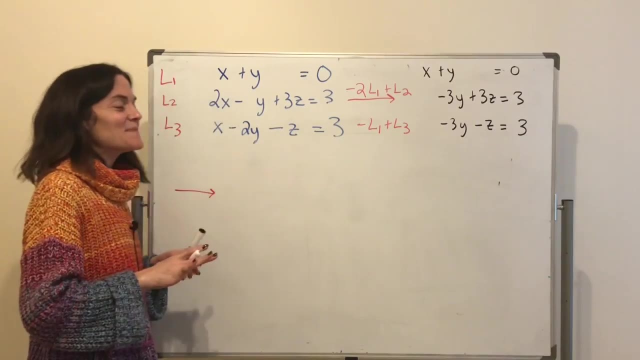 I can't do this on the board. I can't just keep going across forever, especially with this small board, But I'm going to come here. So when you read this, here's what I'll say, and I'll do this this semester, Because it's very likely I'm going to be recording on this small board in my home. 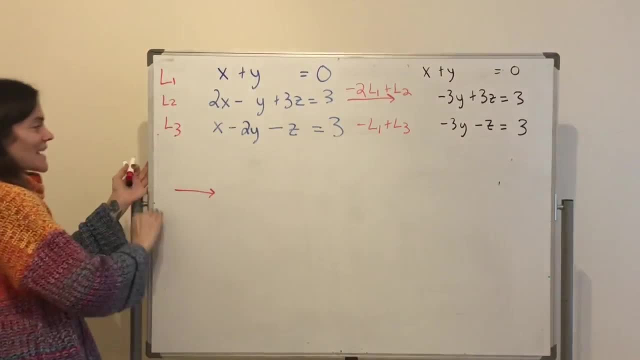 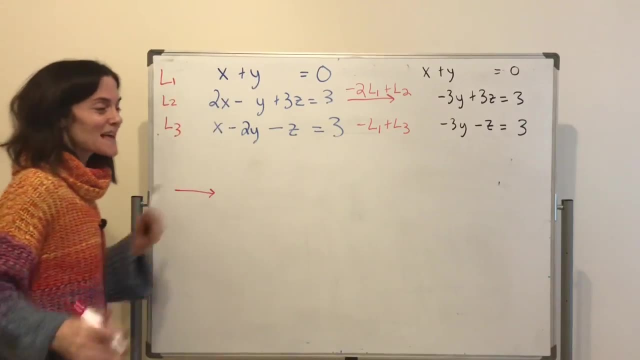 right, We're going to read this way, And then we're going to come to the next line and read this way, And then we're going to come to the next line and read this way. Okay, this is the order. we should read the problems as I'm working them Very nice. So what am I doing? 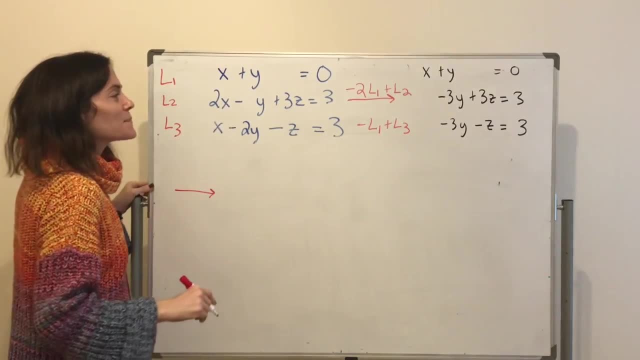 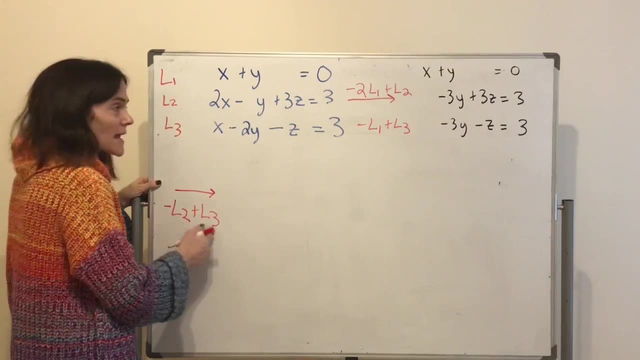 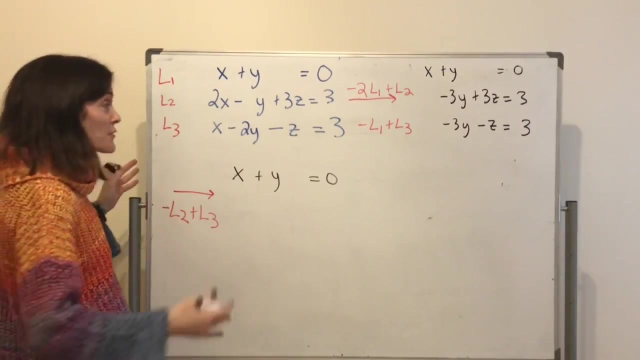 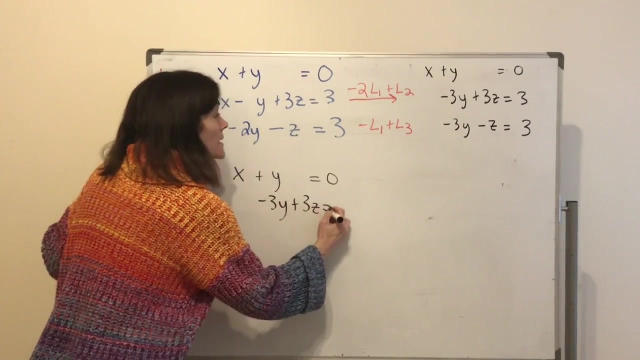 I'm looking at the black system up there And I'm just simply taking minus l2 plus l3.. So I'm adding or subtracting l2 from l3.. x plus y is zero. then we recopy the second line: minus three, y plus three, z is three, And then we 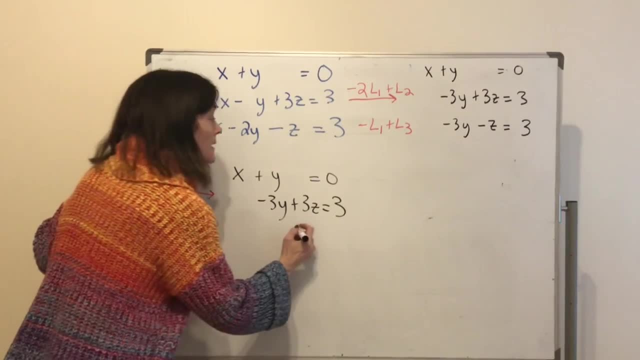 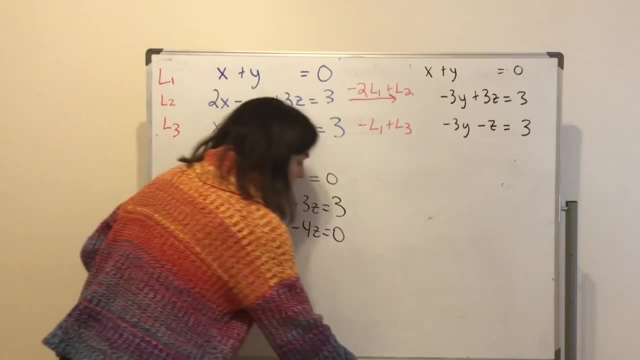 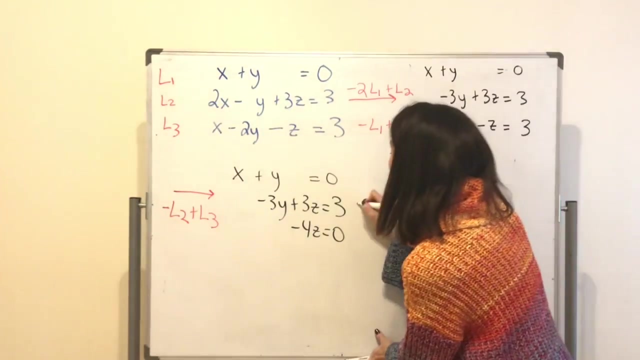 subtract line two from line three And we get, let's see, negative four. z equals zero. Okay, technically we could do the steps as we did when we had two equations in our linear system and two unknowns where. well, what can we do? 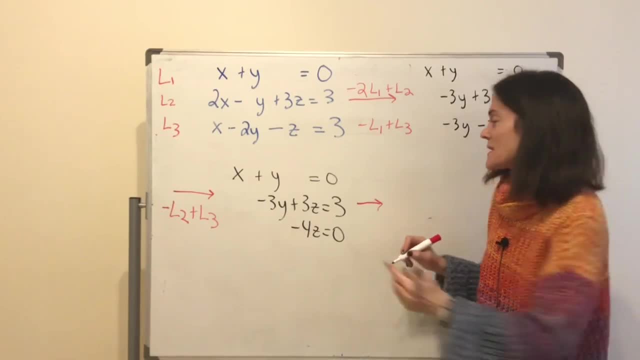 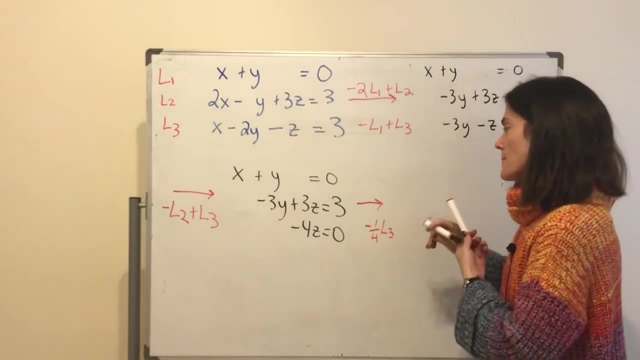 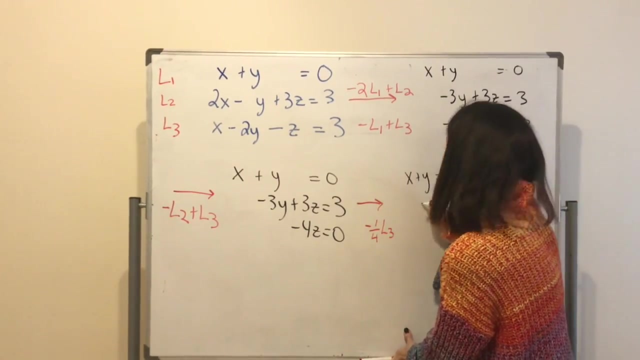 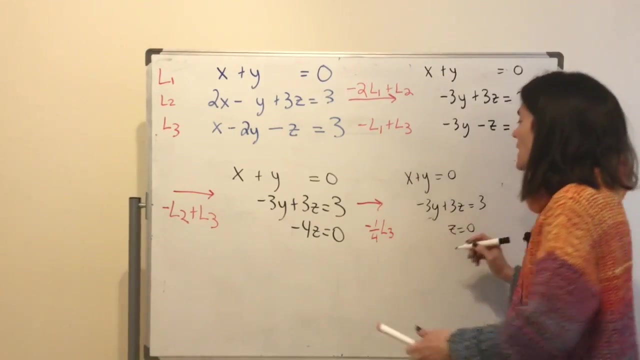 multiply a row by a constant. add a multiple of one row to another. So I would multiply, for instance, negative, a fourth l3.. And you see, we solve for z. This line is the same, this one is still this. we get: z is zero. And I could go through the steps. 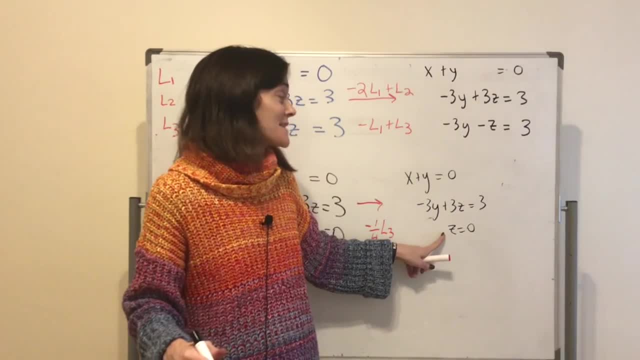 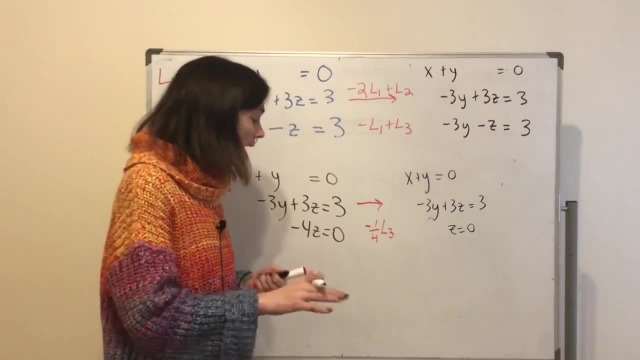 of multiplying. what would I multiply minus three times this row added here And then and sort of working our way back up, which I'll do in the next one. it'll be a little more complicated, But this is fairly easy to solve. You see, we see z is zero. 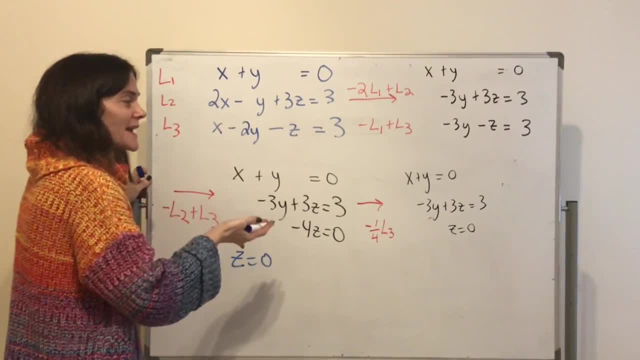 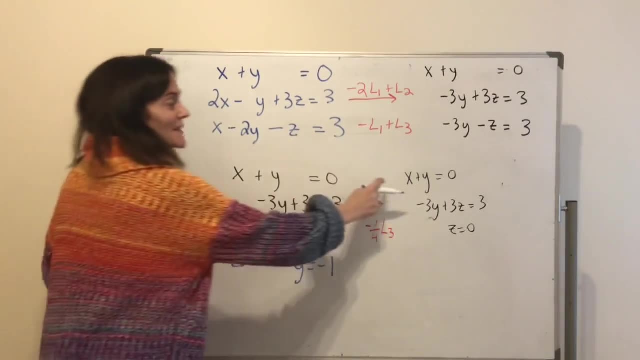 Once z is zero, step back to line number two, and we get that y is negative one. Once y is negative one, step back to line number one, and you get that x is one. So you see, here we have a unique. 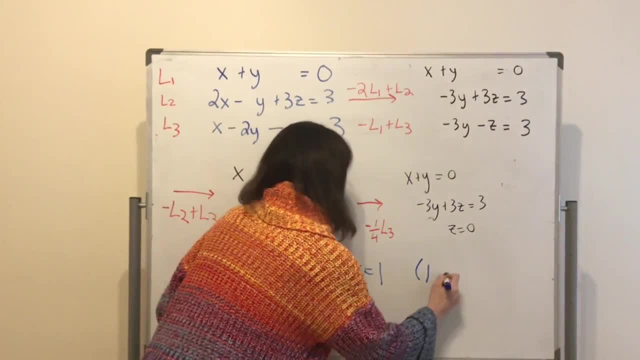 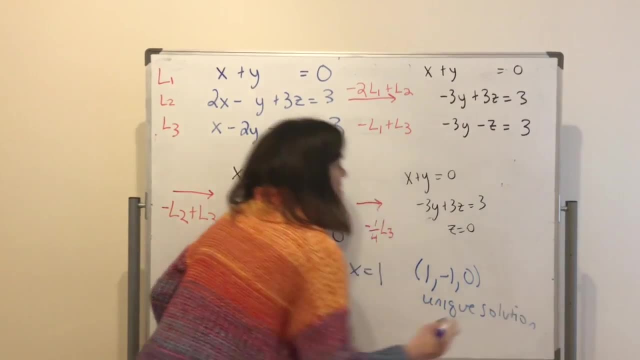 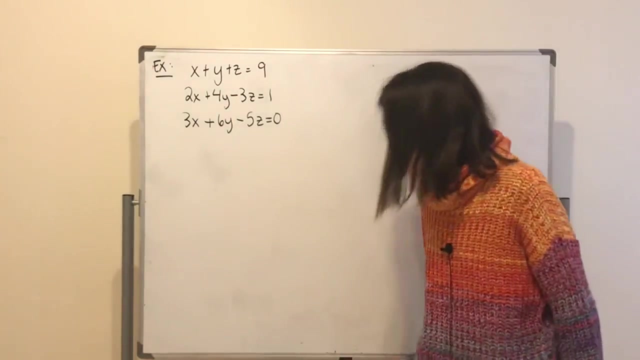 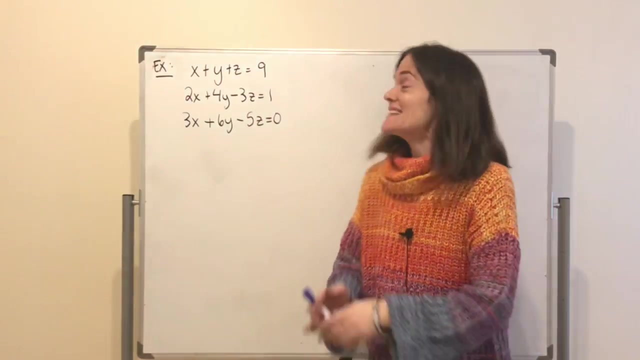 solution. It is the point one minus one zero. we have exactly one solution to this linear system. Let's very carefully do this second example, where we have a linear system with three unknowns and three equations And all I'm going to do is multiply a constant times one line, add it to. 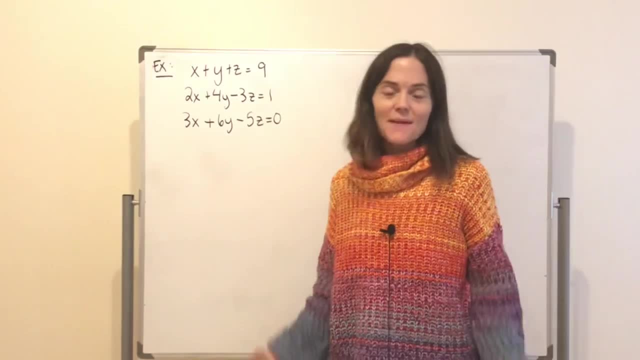 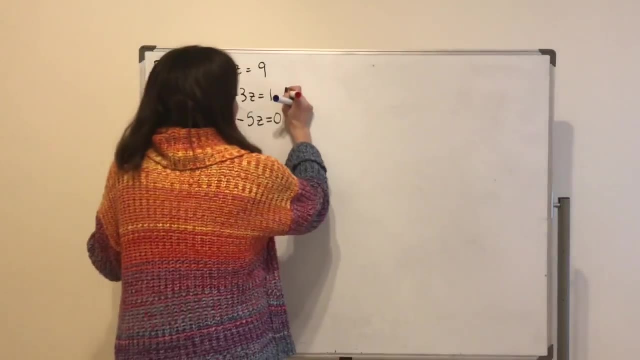 another, or multiply a constant times one line. This is all I will do, okay? So let's do this very carefully. Here we go. The first thing I'm going to do, just like in the last one, is I will eliminate both of these x's. 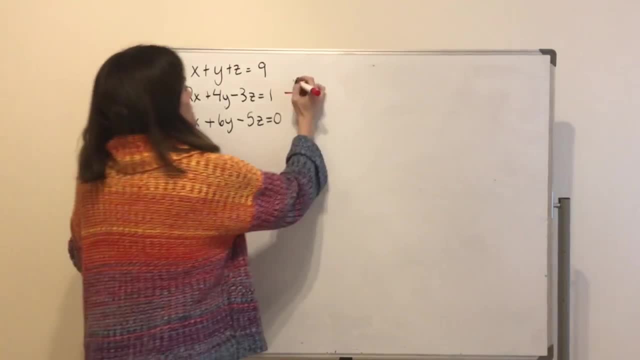 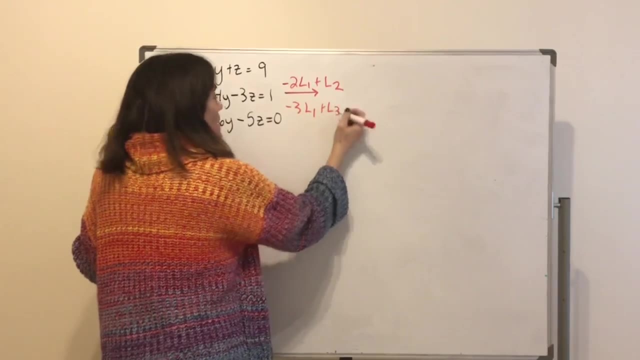 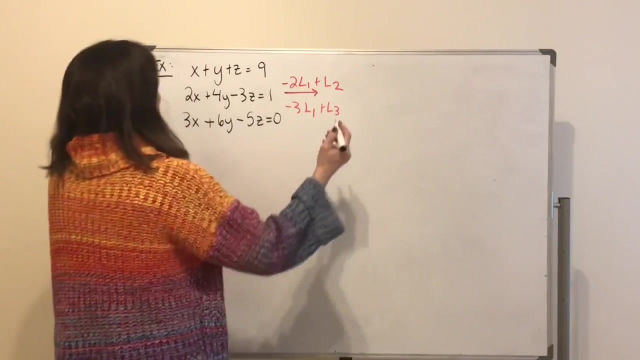 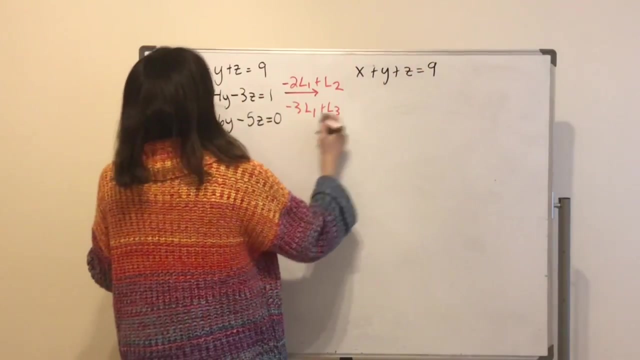 Line one plus line two, line one plus line three. So this involves minus two line one plus line two and minus three, line one plus line three. And let's re-copy the corresponding uh system. The first line has not changed. The second line is now: um well, the x is not there. and then here: 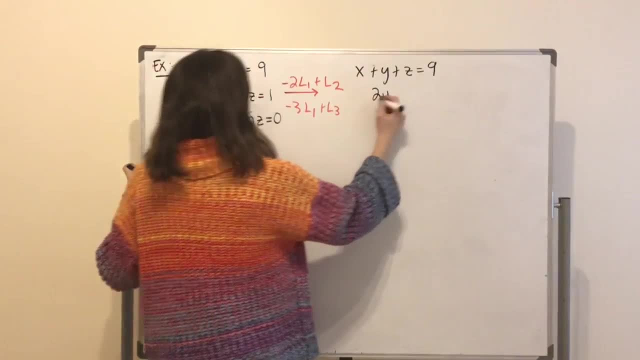 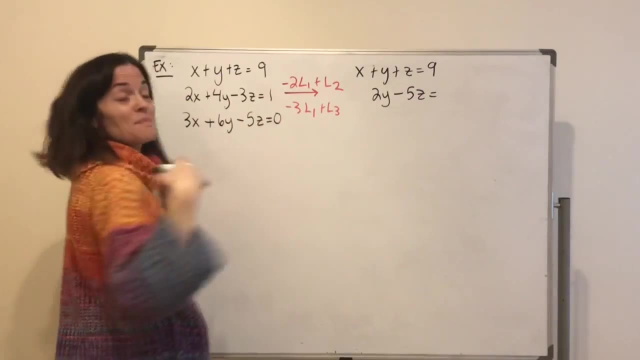 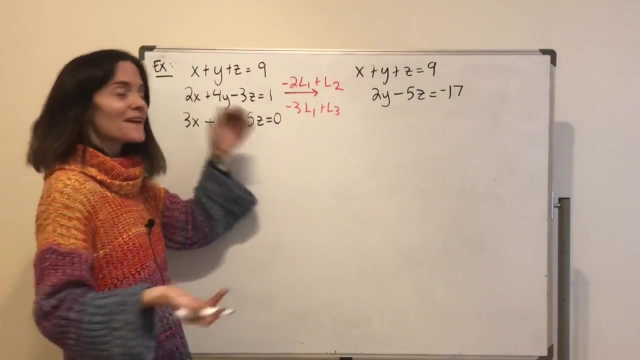 we have: four minus 2 gives me a 2y, And I have minus. 3 minus 2 gives me minus 5z. This will be 1 minus 18 negative 17.. Okay, Now we do this right. We get 3 minus 3. eliminated the x, We have 6 minus 3. 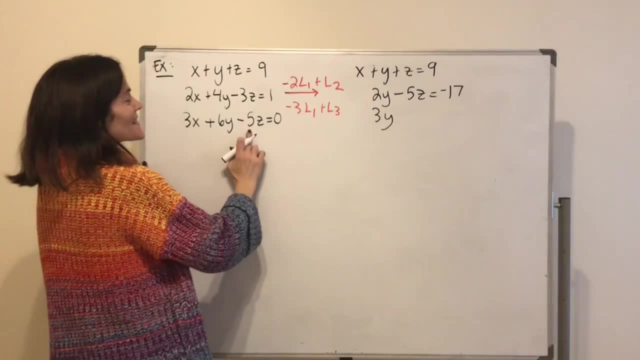 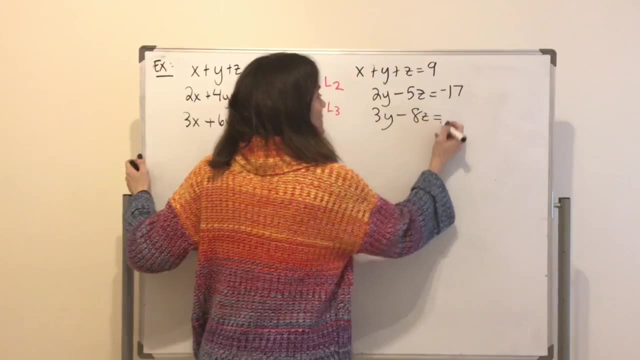 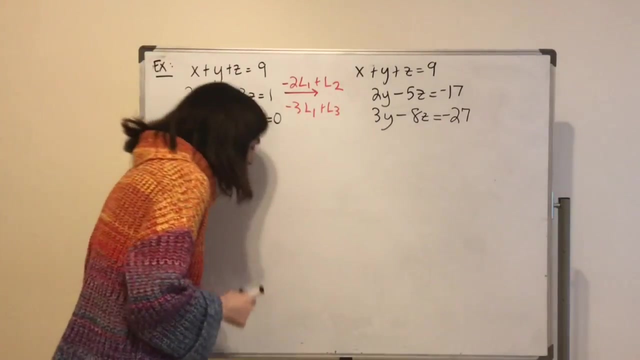 or 3y. We have minus 3, I mean, excuse me, minus 5 minus 3 negative 8z. And finally we have 0 minus 27 negative 27.. Okay, What comes next? Well, if you look at this, 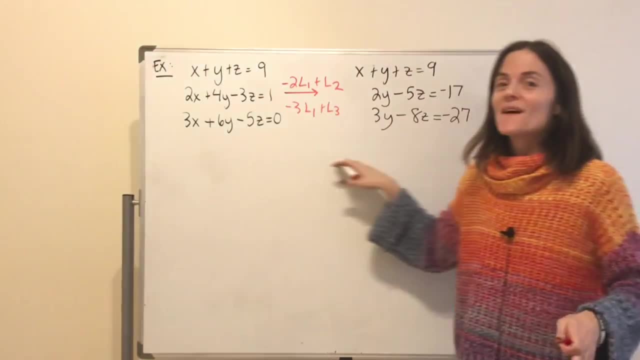 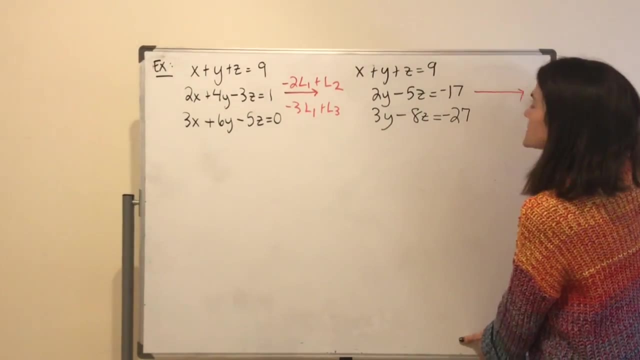 I'm going to put my arrow this way, but, as I mentioned, I will continue on the second line. This is how we have to read with my small board. Okay, So what's going to happen next? I want to eliminate this y. This coefficient is 2.. I will multiply. 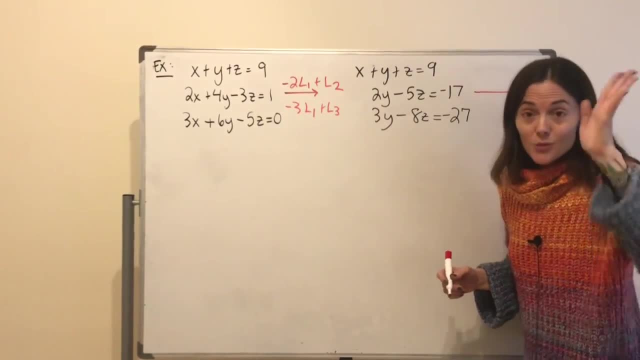 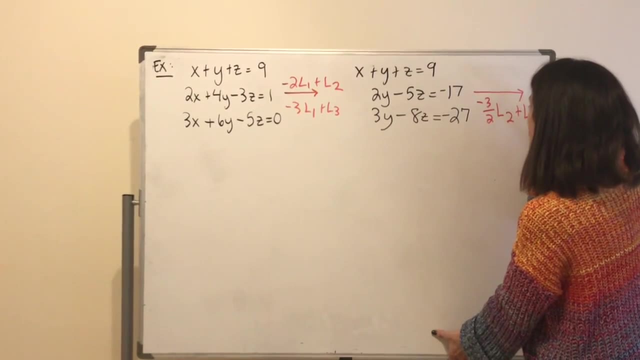 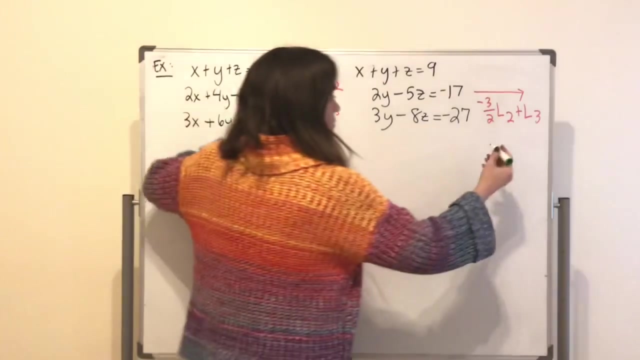 the second line by negative. let's see 3 over 2.. So negative, 3 over 2, l2.. Add that to l3. And here we go. Okay, Here is where maybe I will right here, right underneath this: 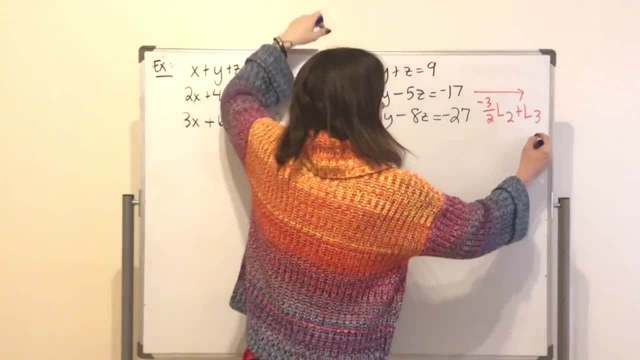 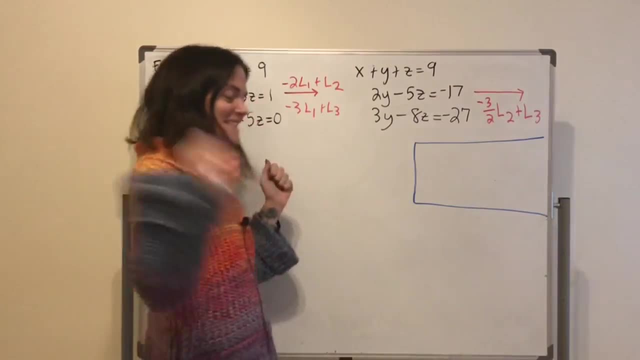 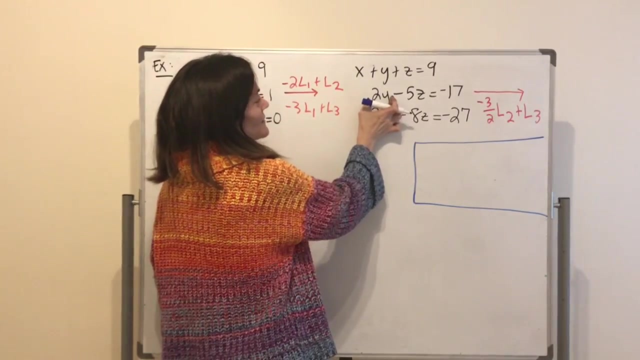 maybe in blue so we can read it. well, I will make a little fraction, Side work box. Fractions will take somebody down. if you're not careful, It's very easy to make a mistake with fractions. So okay, Well, this is fine. We get minus 3 plus 3.. There's. 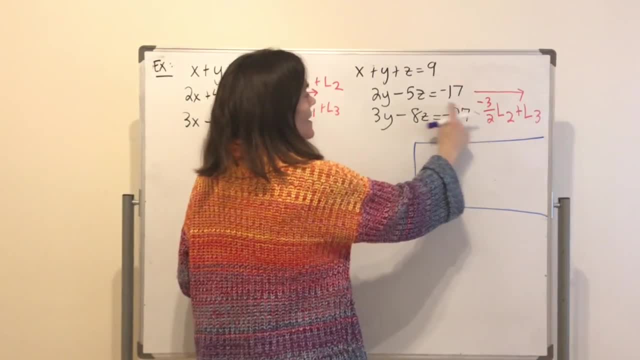 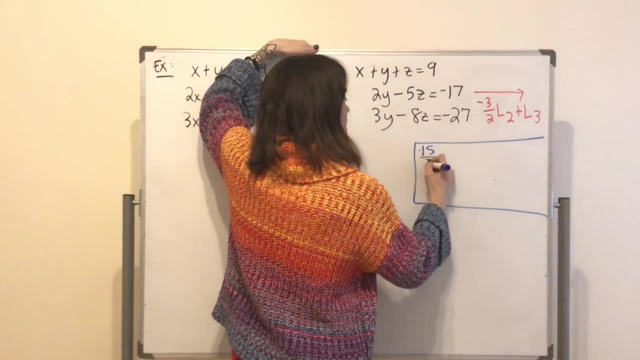 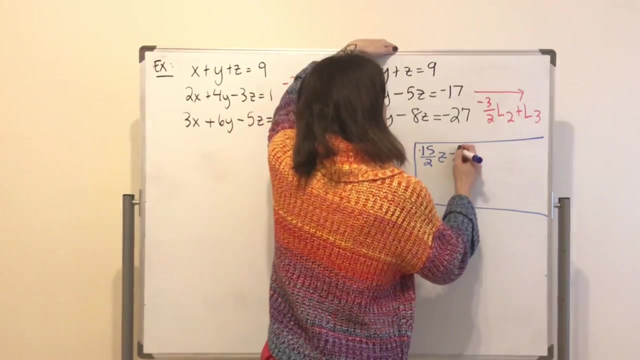 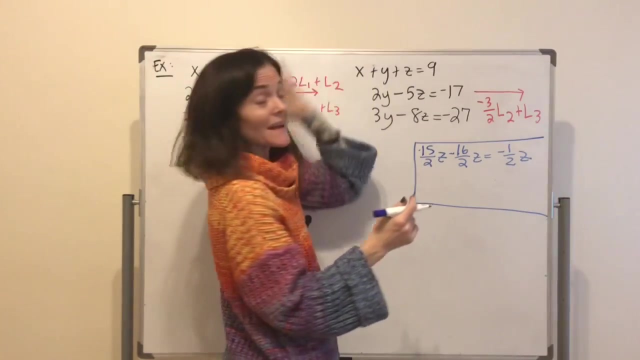 0y. But now, if we have minus 3 halves times minus 5, this will be a positive 15 halves z. And then, with this line, minus 8z is negative 16 halves. This is negative 1 half z. Okay, I'll write it in a moment, Right now. 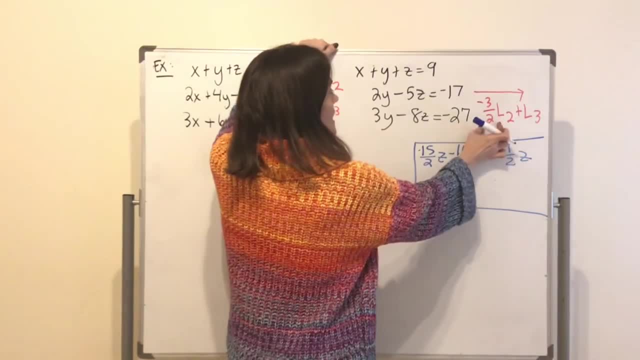 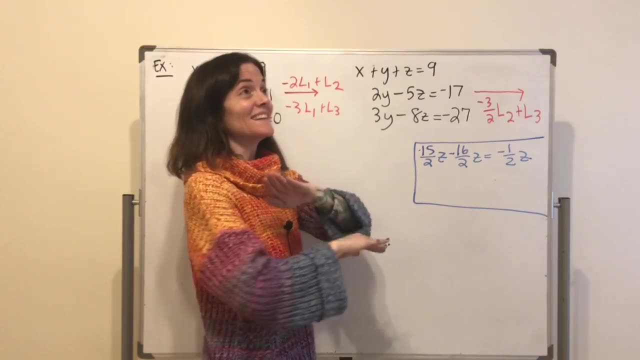 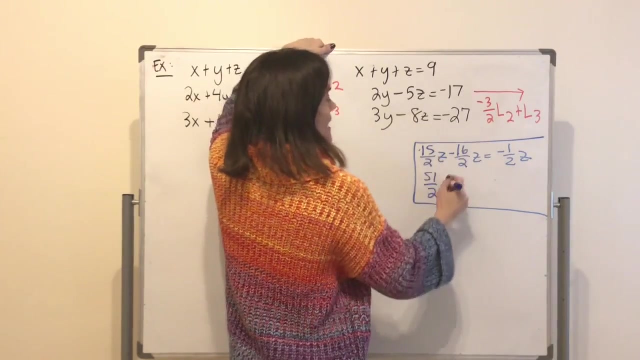 I'm just doing some fractions. Then if I take negative 3 halves times this number, I get: well, 17 times 3 is 51.. So it's a positive 51 over 2.. And I'm adding that to. 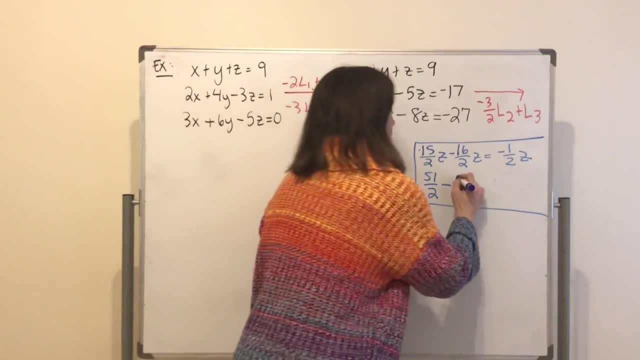 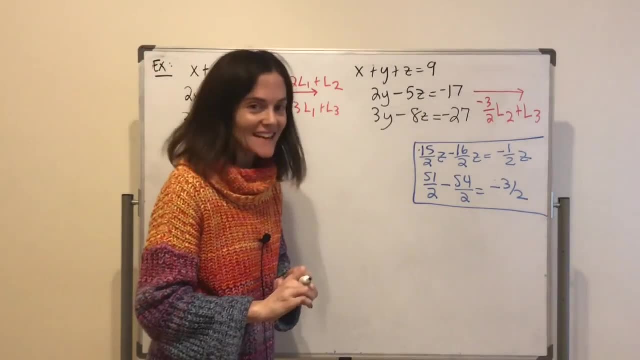 negative 27,, which is negative 54 over 2.. I get negative 3 halves. So this is just my side work with fractions. I will erase it when I need the space. Okay, So what's the result here? 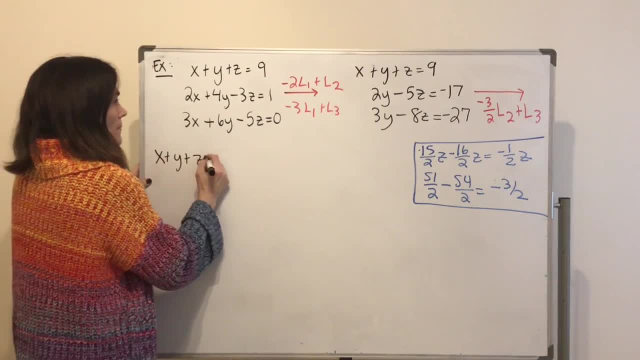 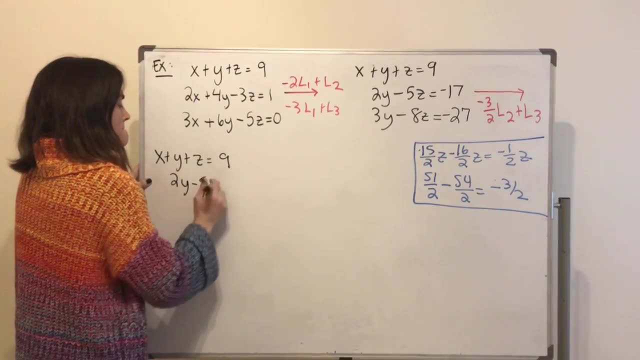 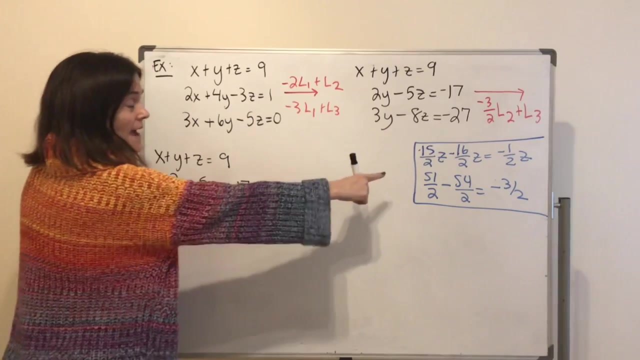 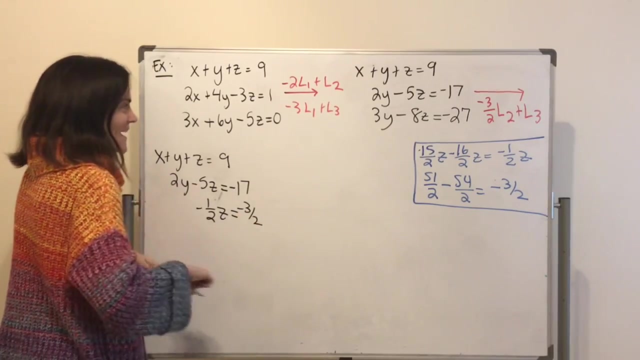 My first line remains the same. My second line I also have not changed: Oops, z, z. And then my third line has become: well, I have the terms here: Negative 1, half z, And this is negative 3 over 2.. Okay, And if all I do is multiply a constant times a line or add a constant? 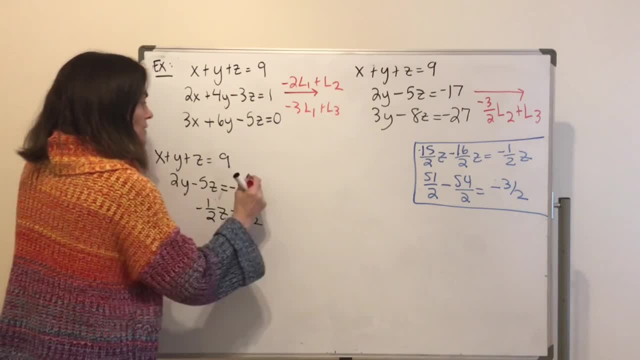 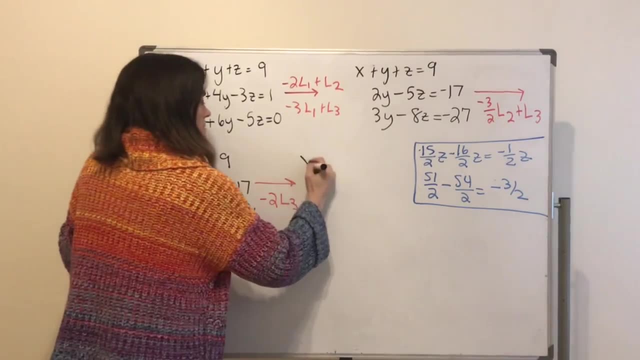 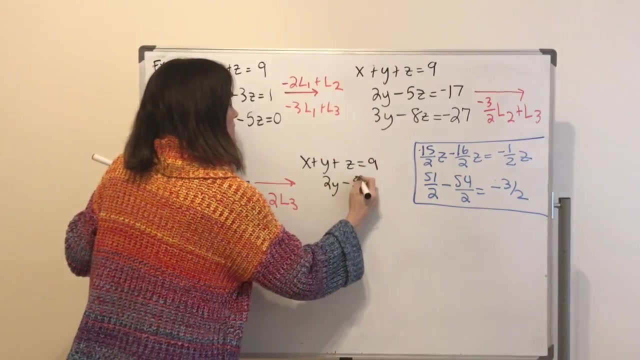 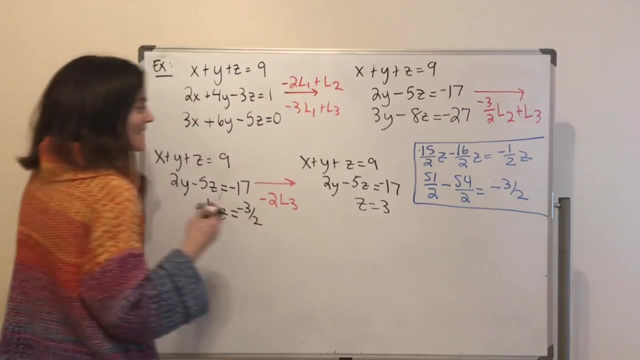 of one line to another. at this point I will multiply through. Line 3 will be multiplied by 2.. So I have x plus y Plus z is 9.. Here I have 2y minus 5z is negative 17.. And here I get that z is 3.. Okay, But as I 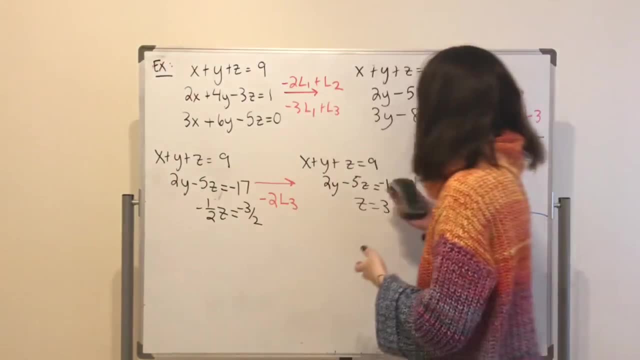 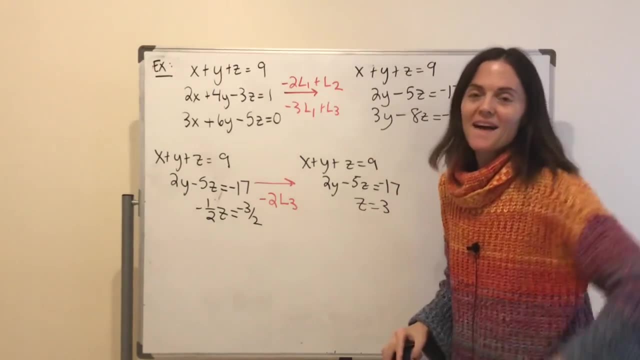 mentioned at the start of this example. I will carefully now. well, here goes my side box, side work box. I will carefully go through this- where all I do is multiply, as I said, a constant by one line added to another, like this Or: 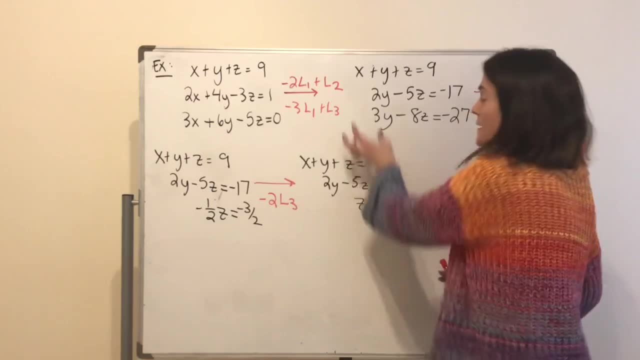 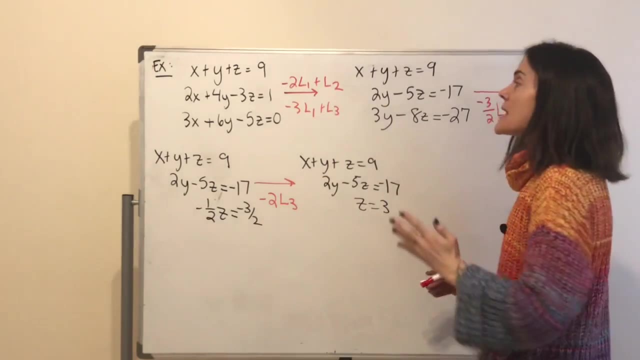 just a constant by one line. So when I'm working backwards, you see I have z, I can solve for y. Once I have y and z, I can solve for x. But what I'll do is it's the same idea. 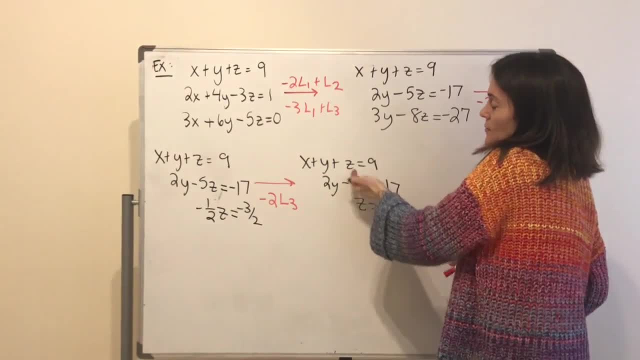 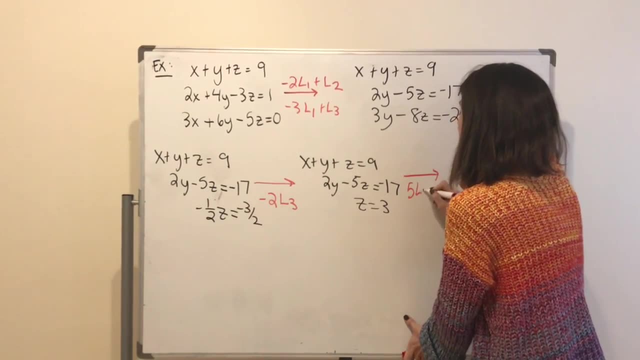 but now I'm going to work up and eliminate the z's in both of these lines. So what is that amount 2?? Well, I'm going to take 5 times line 3 and add it to line 2.. That will get rid of this z And. 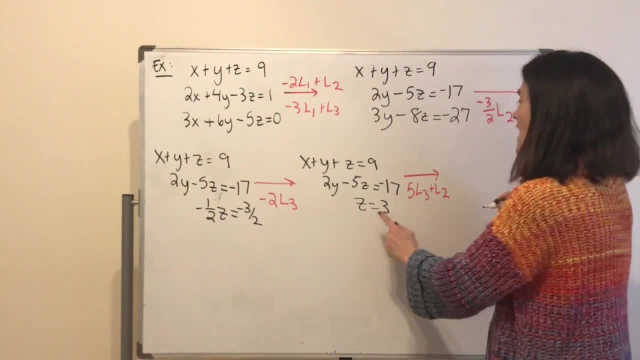 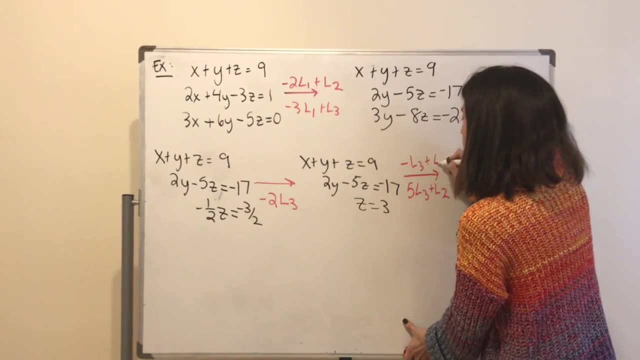 then, or this z2.. And then I'm going to add it to line 2.. And then I'm going to add it to line 2.. And then I will take minus line 3 and add it to line 1.. Add it to line 1.. Okay, So now let's. 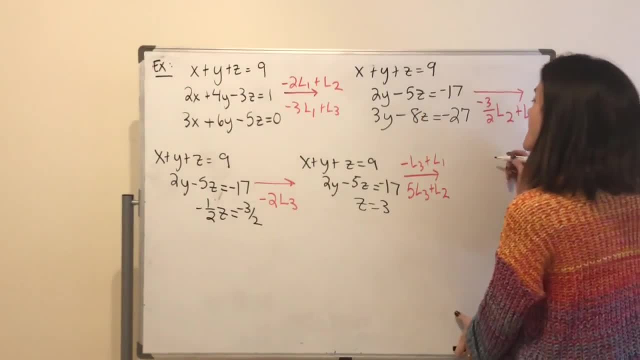 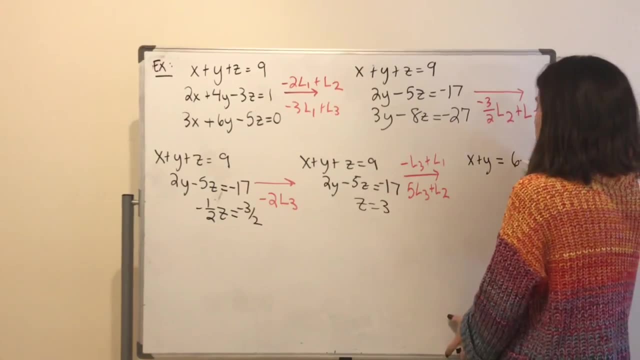 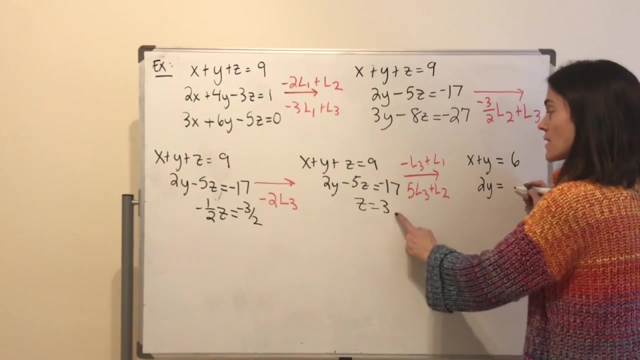 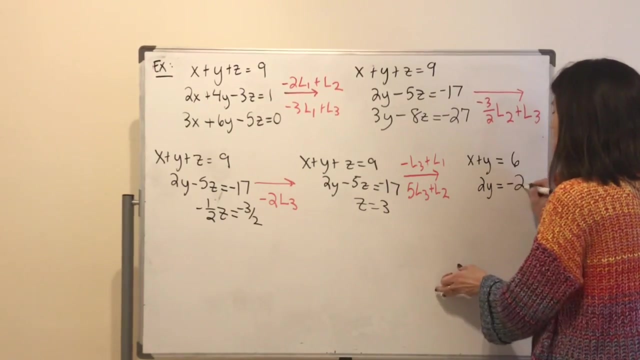 write what results We have: x plus y equals 6.. And then here we get: 2y equals. well, you take minus 5, or 5,, excuse me- positive 5 times. This is 15 minus 17 plus 15 minus 2.. Now you see. 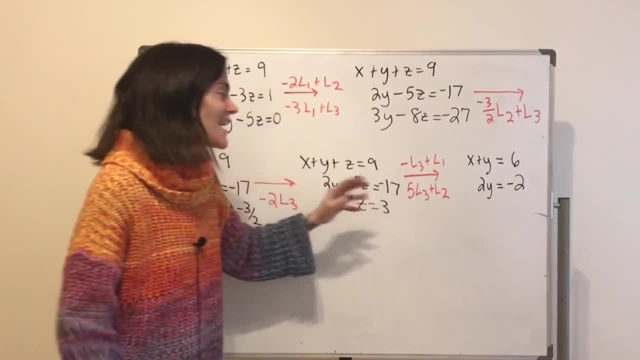 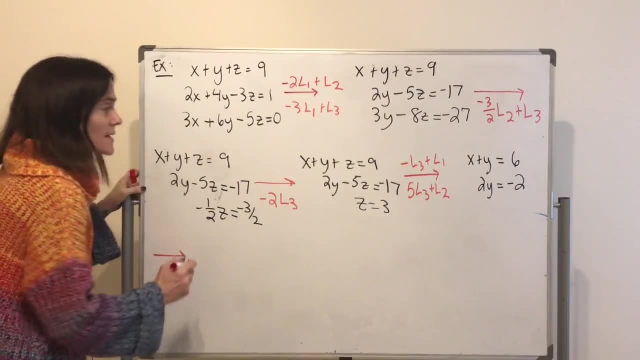 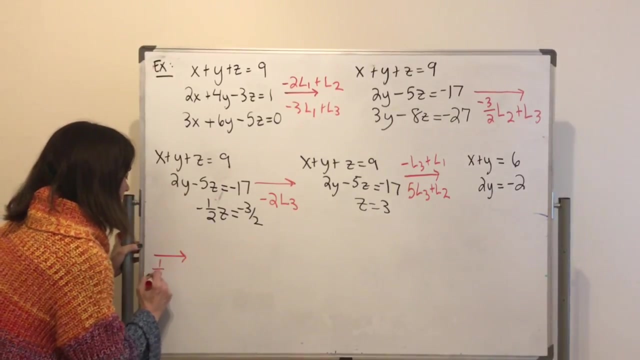 this is looking great. Now I'm going to continue this pattern, As I mentioned very carefully. the next thing I will do is multiply through line 2 by negative or positive 1 half, Excuse me, So I take 1 half line 2.. 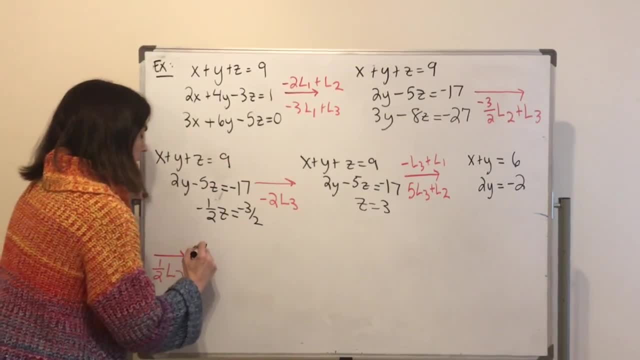 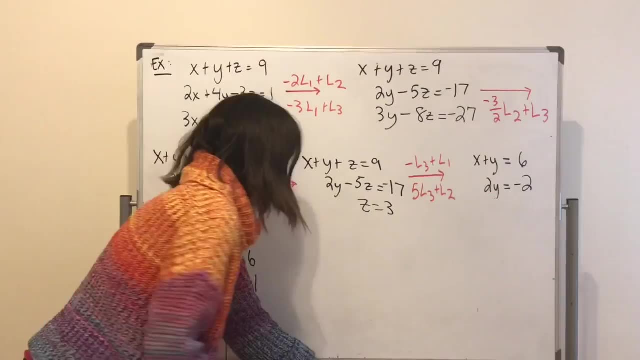 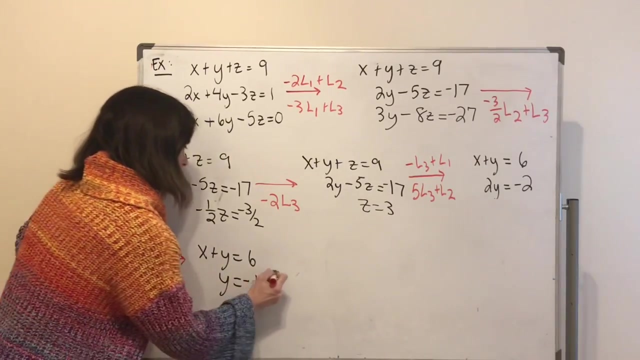 I've changed the name at the bottom: X plus 9.. I'm going to take my first line. I have not changed: X plus y is 6,, but I get y is negative 1.. And then this very last step. what is it that I want to do? 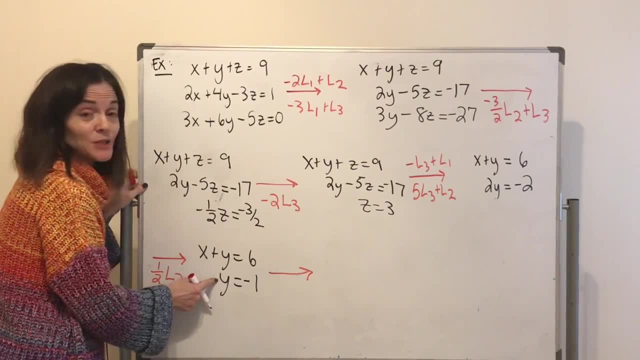 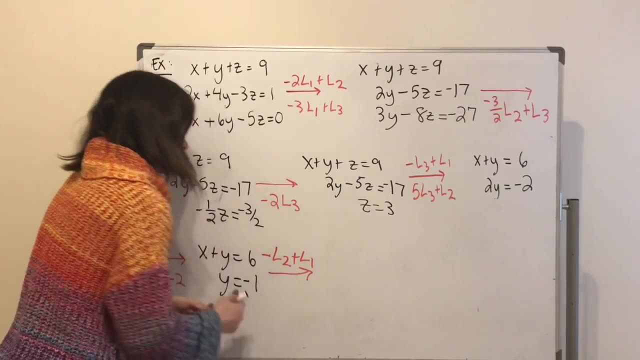 Well, I want to take uh minus line 2 and add it to line 1.. Okay, So here we go. This would do uh 27 modules intercalations. Here we go. This would give us x equals 7.. 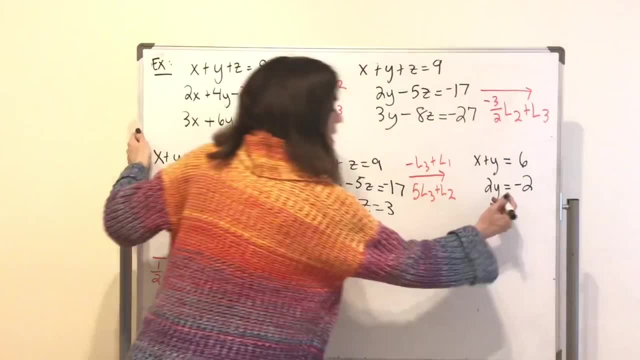 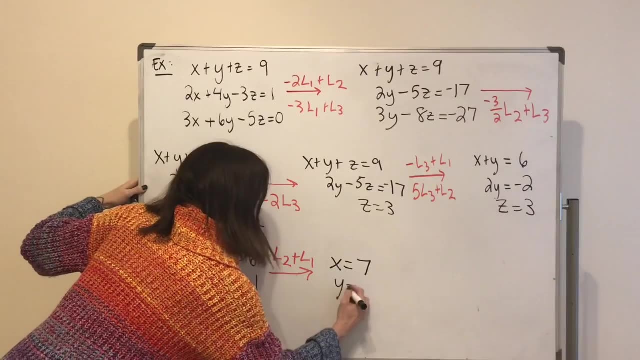 Now, technically, I didn't copy the whole system every time. We still have z equals 3 here, z equals 3 here, and we would have: y is minus 1 and z equals 3, right, I should have kept copying that each time, for example. 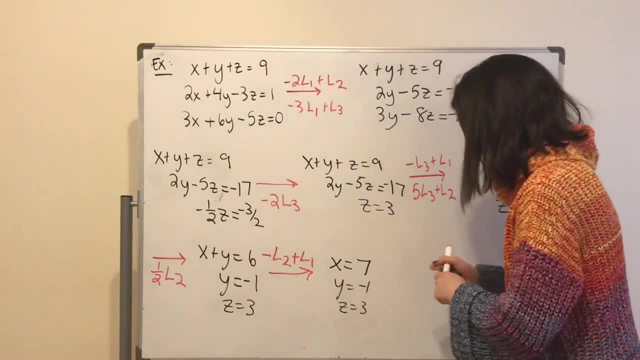 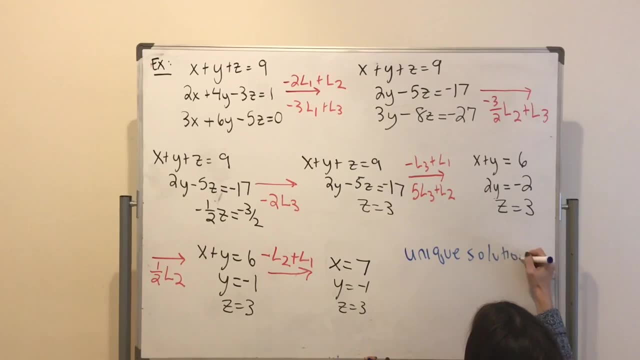 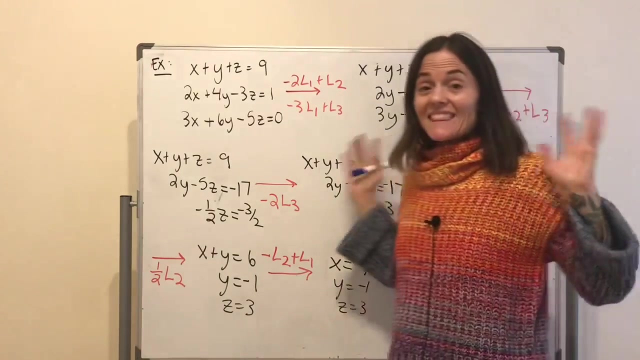 But now we have the unique solution. So the unique solution here was the only solution that we got was this: 0.7 comma minus 1, 3.. So we have one solution to this system. But one thing I like about the way that we did this: it was very methodical. 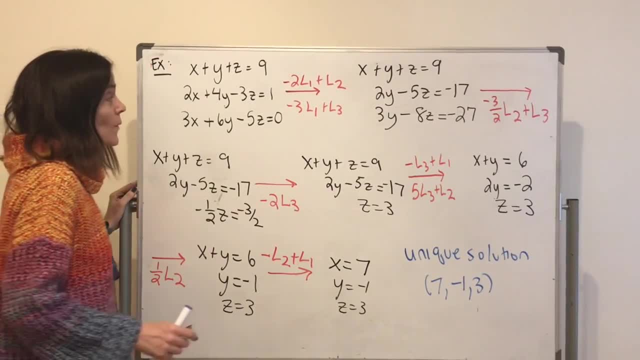 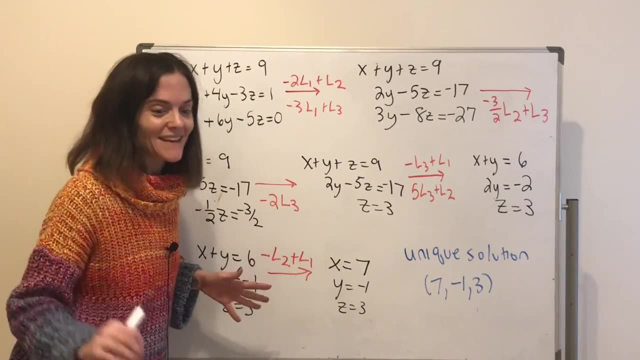 and this was my point- where we could have followed these same rules and done, say, a 30 by 30, where we have 30 linear equations and 30 unknowns. Well, not on this little bitty board, but in principle. 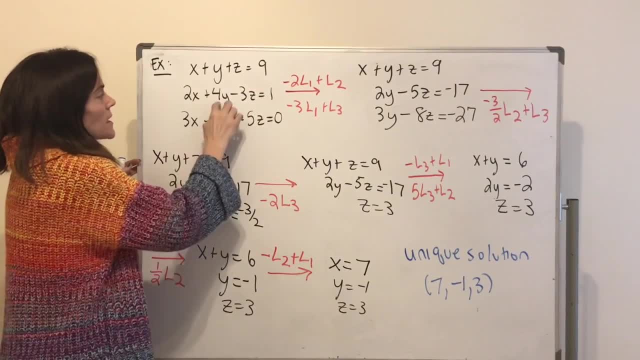 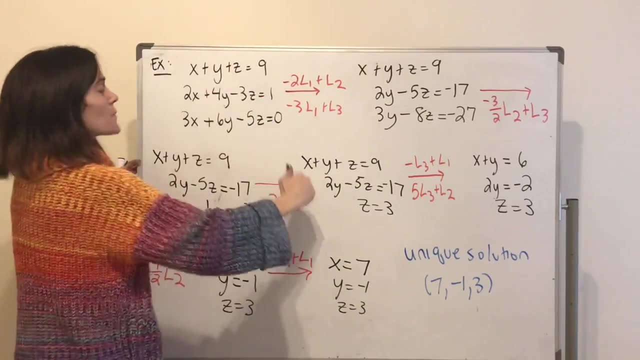 where you eliminate everything under here and then you keep the y eliminate under here. Then you would keep this one eliminate, keep this one eliminate until you get down to the bottom, and then you just work backwards. You eliminate above, eliminate above, eliminate above, like this: 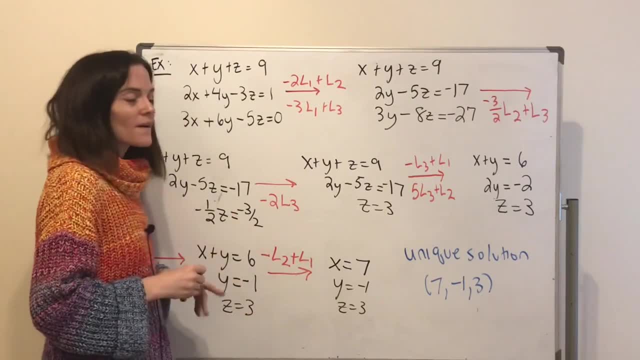 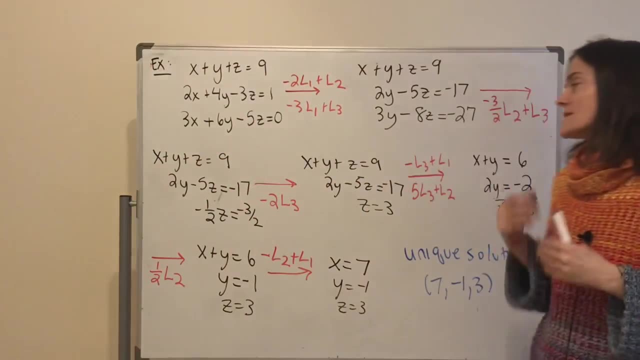 We are going to be using this a lot more, this type of elimination, throughout the semester. We will just get into the language of matrices, which I think makes it a little bit easier to use, Maybe a little bit easier than writing out the equations every time. 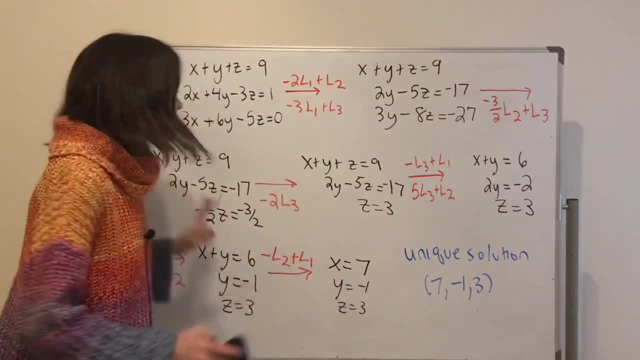 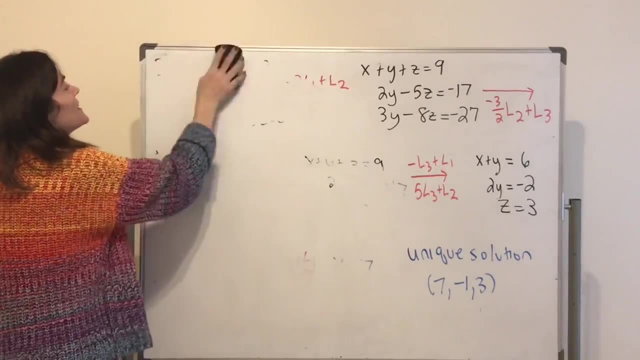 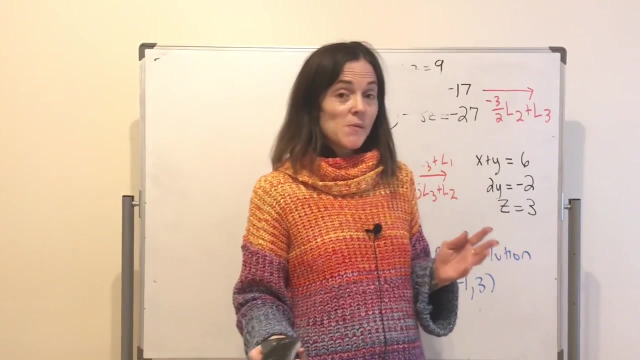 Okay, well, but before we do any of that, we're still in our introduction to linear systems discussion and section. I would like to do two more examples to see what other types of behavior can happen when you have, for instance, three equations, three unknowns, and then we will look at the pictures. 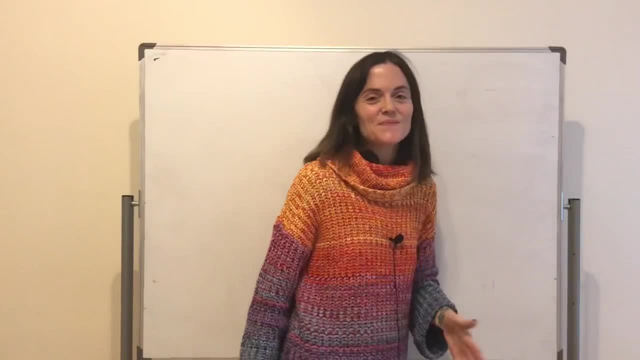 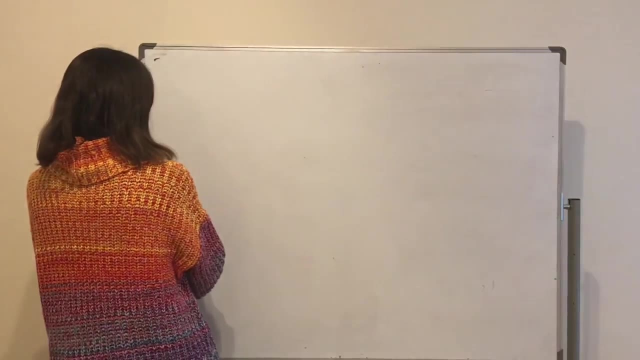 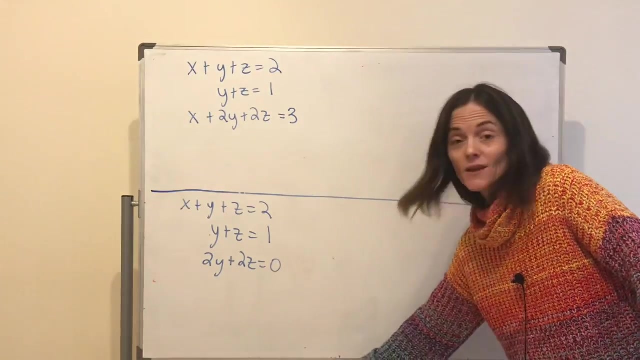 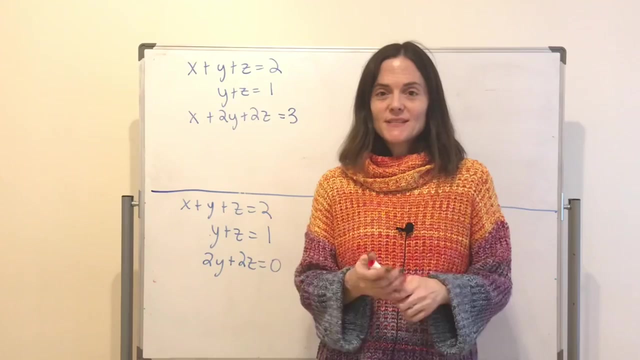 to understand what they mean. So let's look at two more. maybe I will draw a line right here. Well, let's begin as we have in the other two examples. These will be different though The last two examples. we had a unique solution to each linear system. 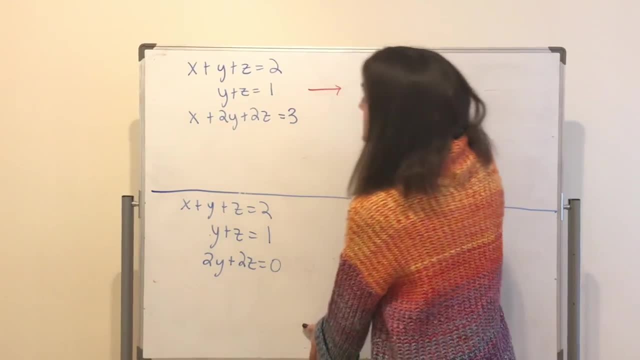 Here let's begin. If we try to understand the linear system, we will have a solution to each linear system. Here let's begin. If we try to understand the linear system, we will have a solution to each linear system. Well, we already have no x in the second equation. 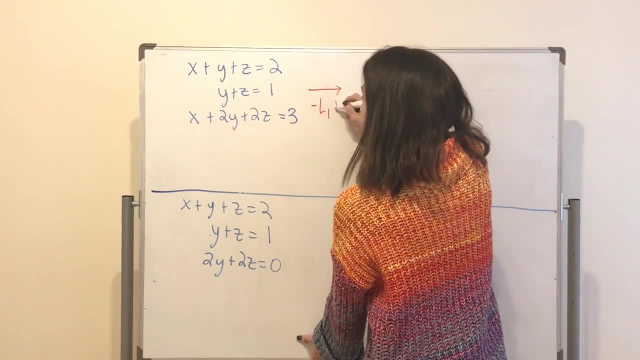 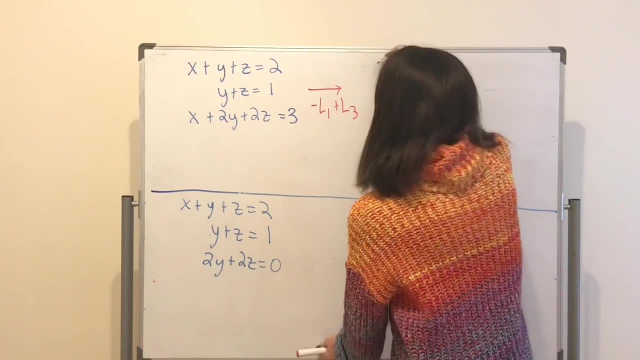 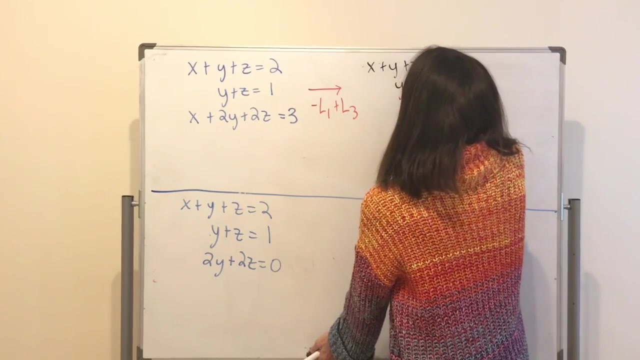 Eliminating the x here. we would take negative L1, add it to L3.. And what do we get if we then write the result: We have x plus y plus z is 2.. We have y plus z is 1.. 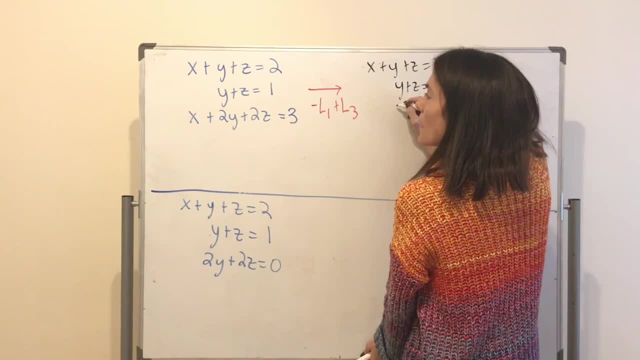 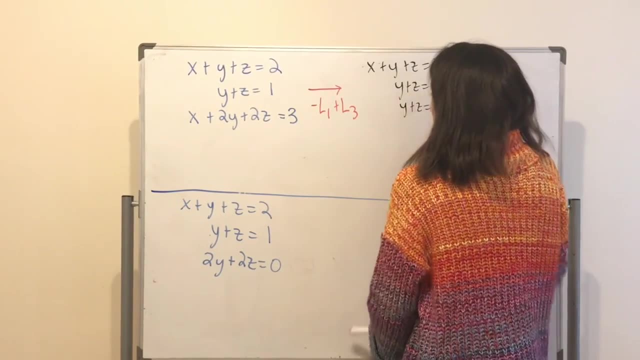 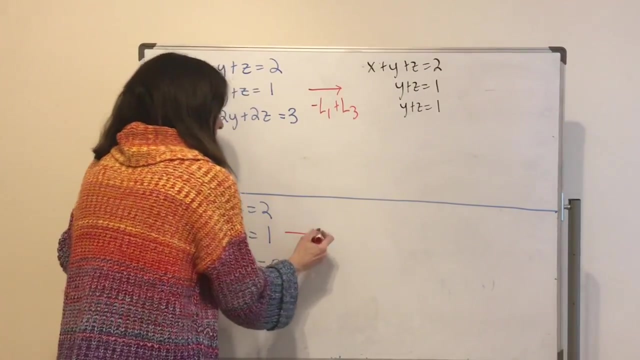 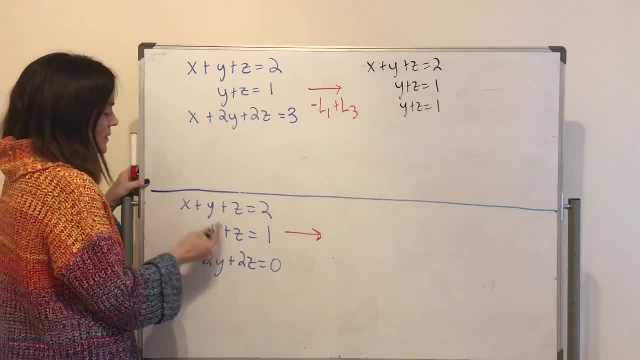 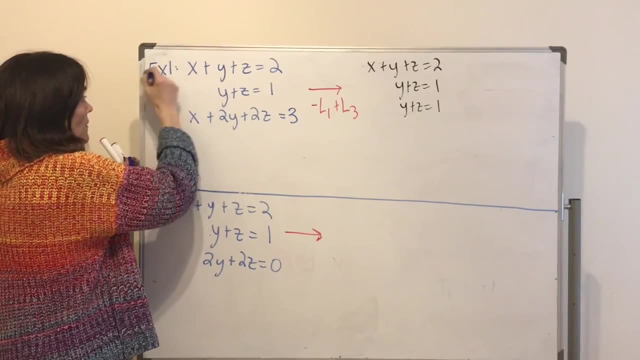 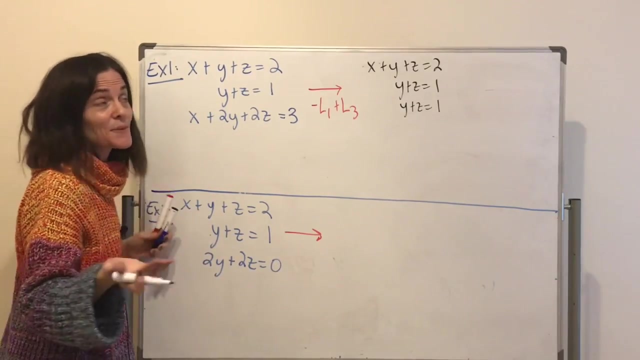 treating these together. well, this example, in a way, is handed to us. this is like example 1 and this is example 2. it's already handed to us where the X is eliminated in the first two equations, so I would just work to eliminate the Y in. 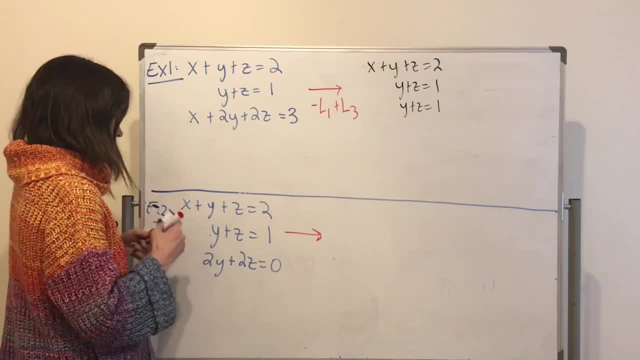 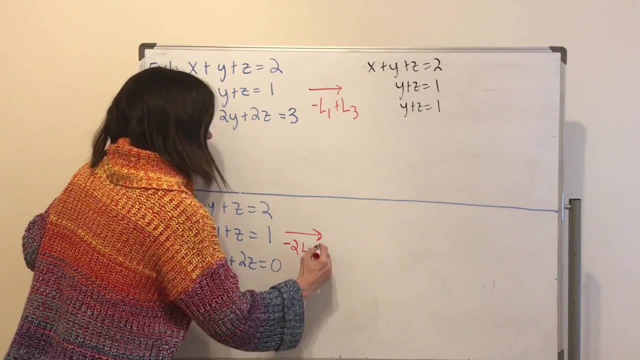 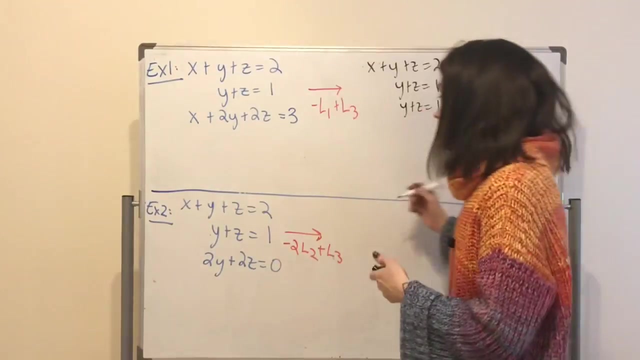 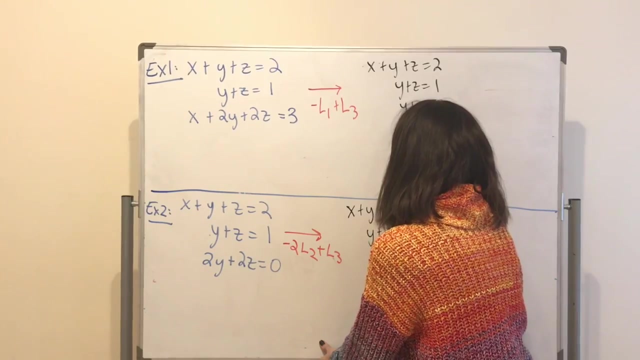 this third equation, which would be here we could just take negative 2, L 2 added to L 3. okay, great, let's write down what result is that we have X plus Y plus Z is 2. we have Y plus Z is 1, but then, if you add: 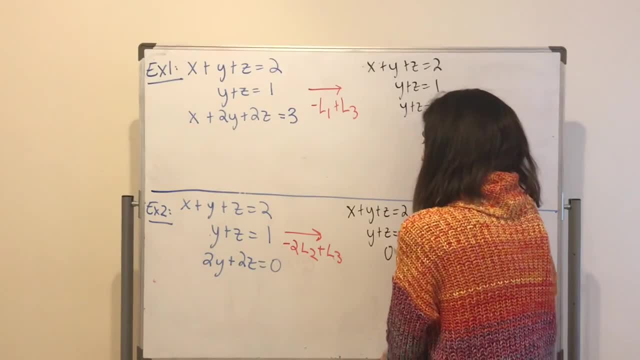 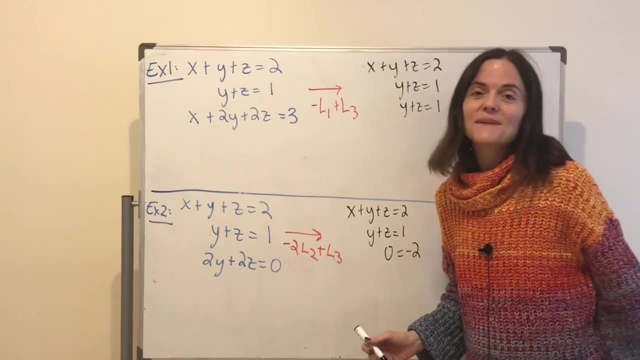 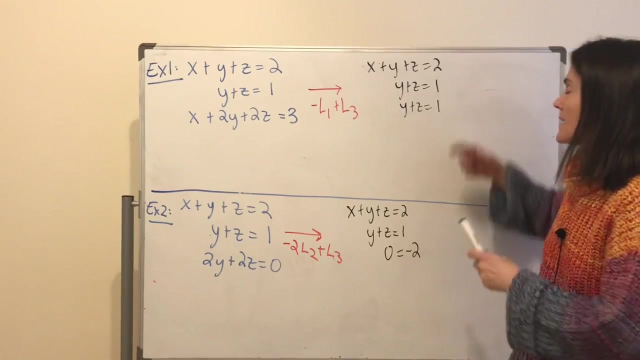 negative 2 times this plus this, we get 0 is negative 2. okay. well, these are both similar to phenomena that we saw with two equations and two unknowns. look here, it's really just two things, and in fact I could take. let's even do another step if we want to, for 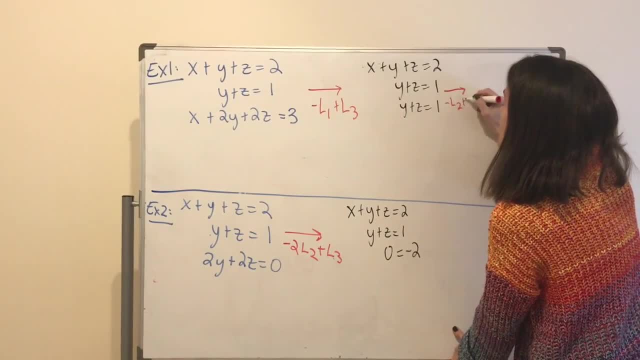 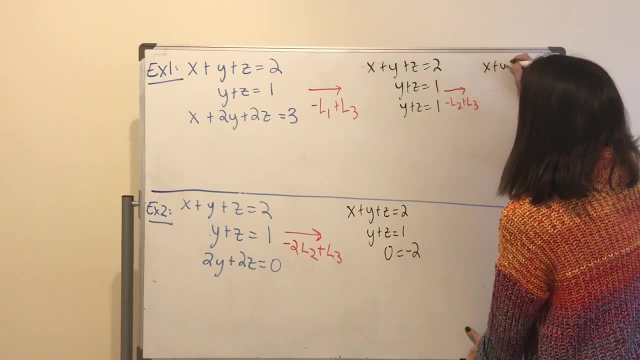 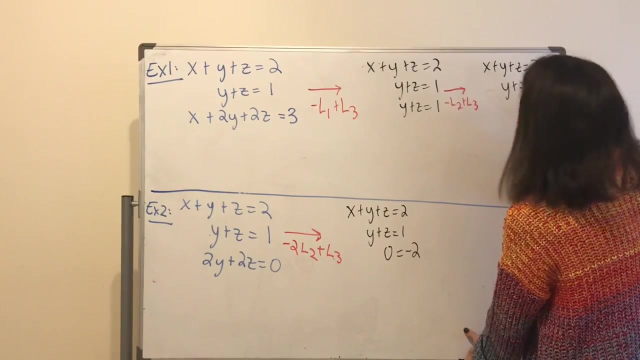 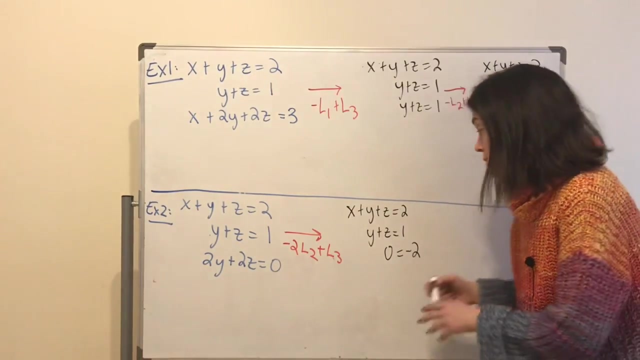 completeness. I could take minus L to add it to L 3, and then we see even more clearly what's happening. we have X plus Y plus Z is 2. we have Y plus Z as 1. then here we have 0 is 0. so now these match up almost the same, except inuses. 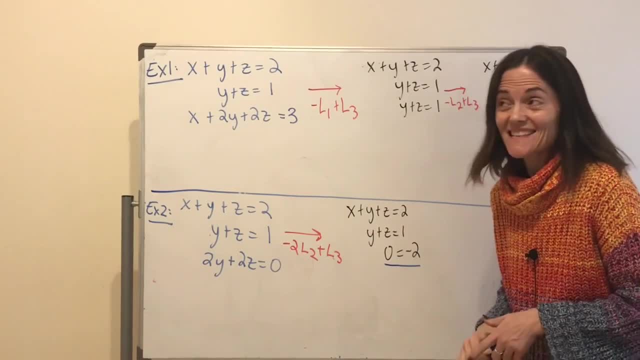 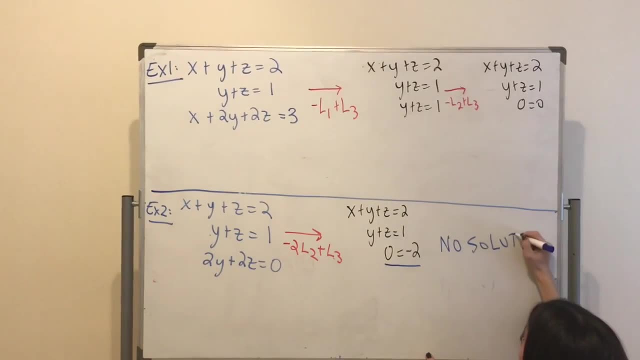 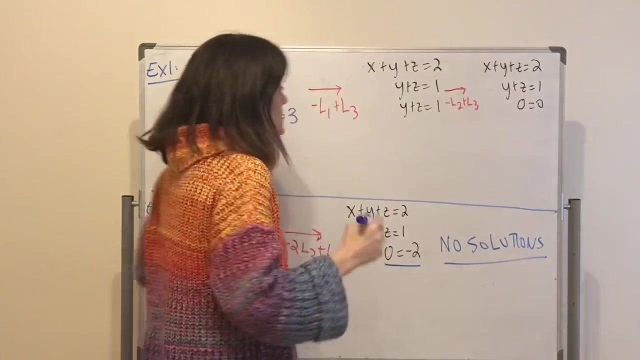 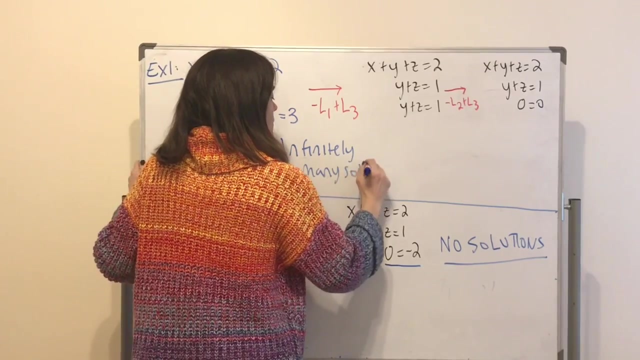 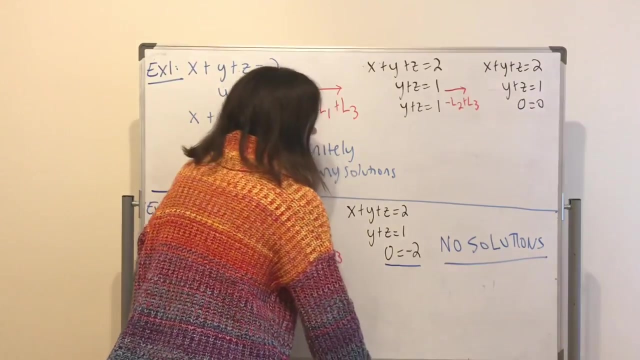 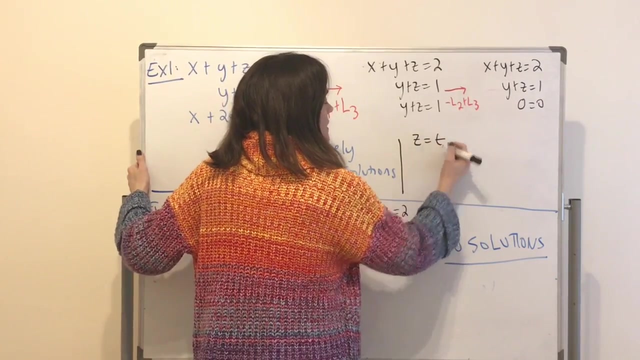 this equation? it's not true. this equation says no solution, so we have no solutions here and up here. well, there's gonna be infinitely many solutions. how could you find some? well, let's just say for a moment, how could we find infinitely many? okay, very nice. let's say that Z is T or T can be any real number, okay, well. 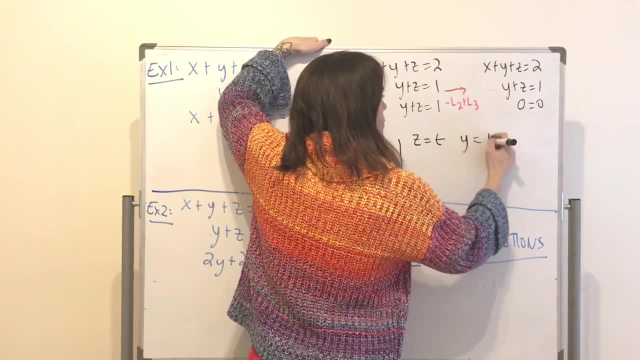 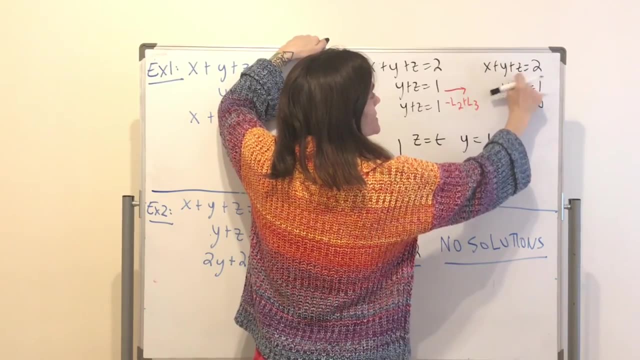 then why solve? Y would be 1 minus T right now. if Y plus Z is 1, that means this: to this sum is 1. so what would be 1 minus T right now? if Y plus Z is 1, that means this: to this sum is 1. so 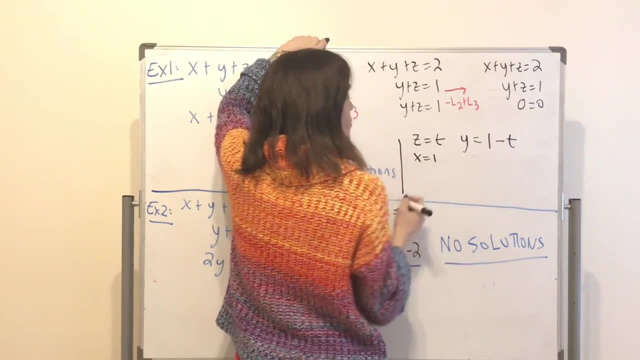 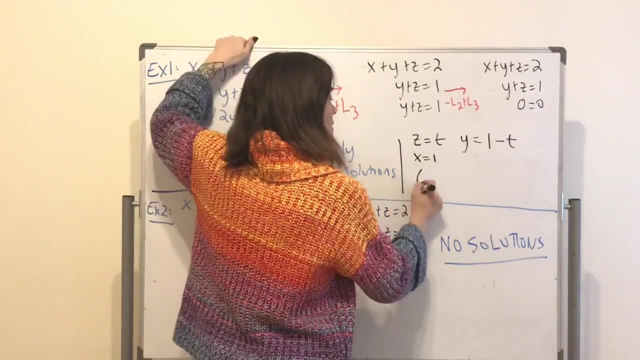 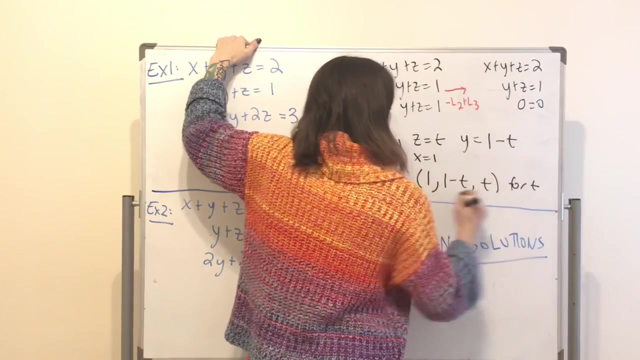 right now. if Y plus Z is 1, that means this: to this sum is 1. so subtract here: X equals 1, no matter what Y and Z are, provided Y plus Z is 1, right. so if you solve both of these, so here 1, 1 minus T. T for T in R. this was our real. 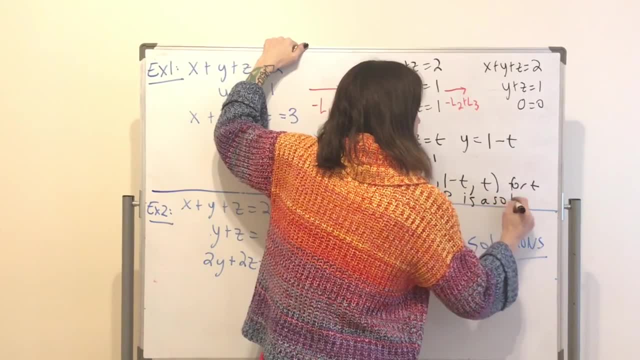 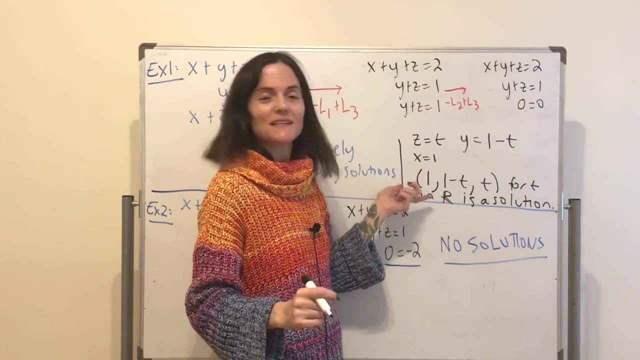 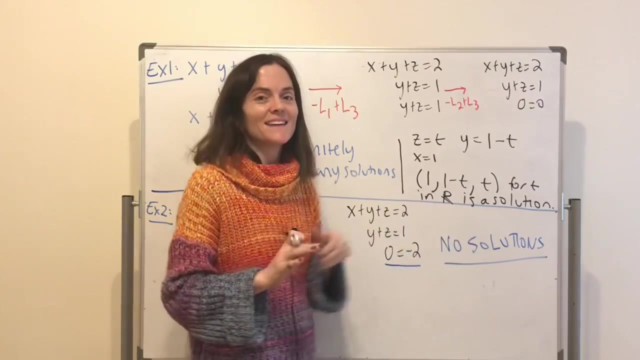 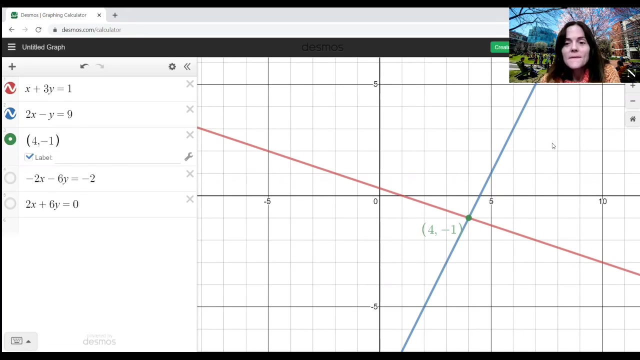 numbers thing is a solution. this is infinitely many. every real number T corresponds to one solution like this. we have infinitely many and this, this will be as we will see in our pictures, this will be a line. well, what I'd like to do is spend a few minutes going over graphically or geometrically, what can 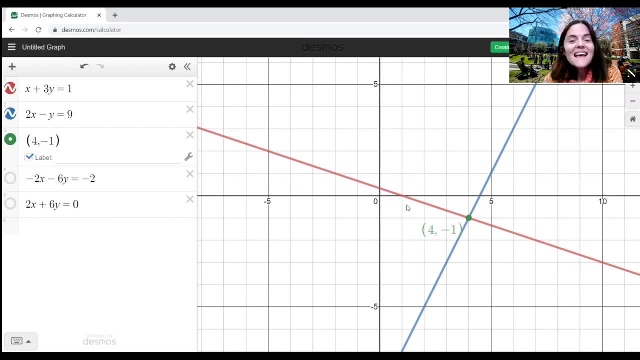 happen with these linear systems, and I will start with the first few examples that we saw, which were just two equations and two unknowns, and the first one we saw was was here: X plus 3y is 1 and 2y, 2x minus Y is 9, and we 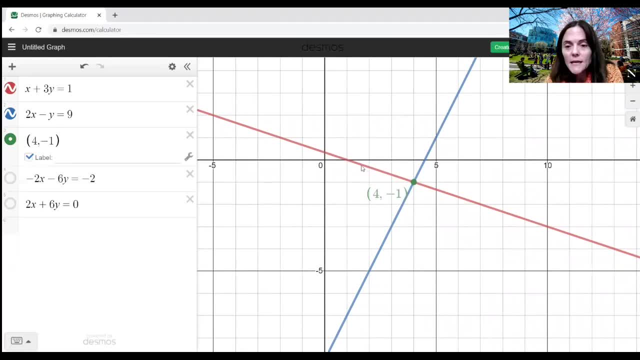 found that there was this unique solution and you can see it here. each one of these linear equations defines a line in the plane and they intersect. well, you can't see my hands because of my background is northeastern. okay, they intersect at this 1 point 4 comma minus 1, which we calculated. this is one way. 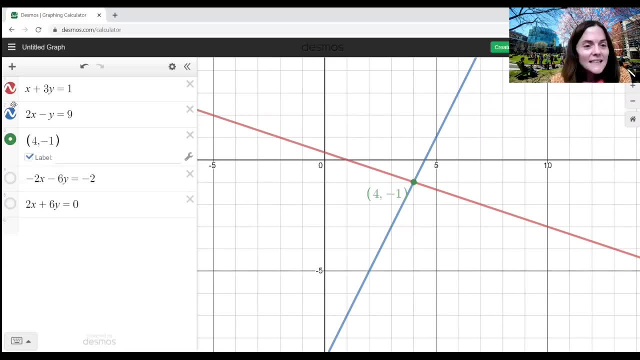 that lines can intersect in the plane. however, now let me take off this. if we take, for example, we have these two: X plus 3y is 1 and minus 2x minus 6y is minus 2. oh, take that label. but you see, here these are the exact same line. we. 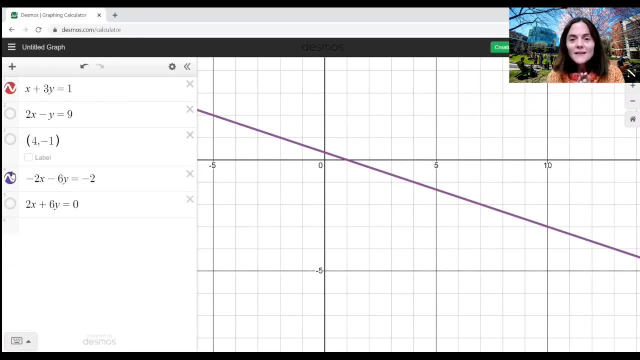 had infinitely many solutions. well, do it again. it's just two overlapping lines. the whole line worth of solutions is our, is our solution set? okay, but then finally we have this third, and you see the problem here. these are two lines in the plane, but they're parallel and they never intersect. these were the two that i had no solutions when 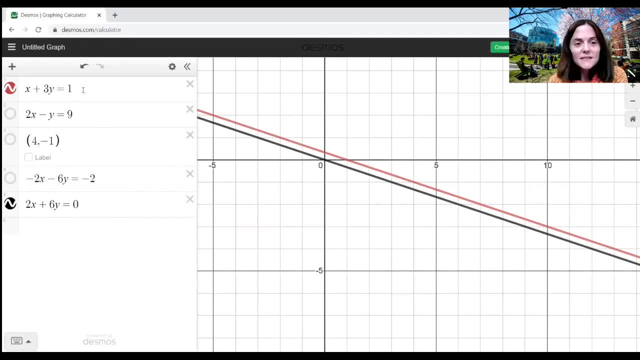 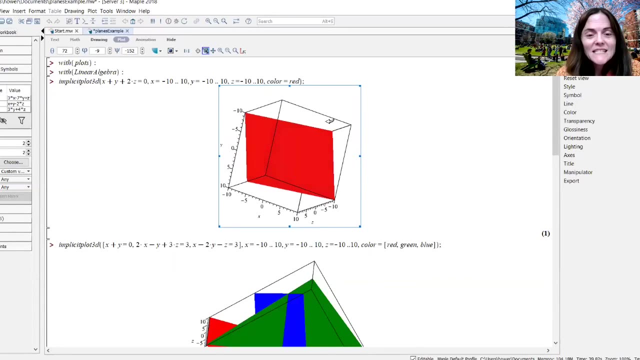 i tried to solve the linear system, which was this: this first equation here and then the third equation below. okay, so this is in in the plane: two equations, two unknowns. we plot lines in the plane. let us start by just looking at, so you see what i have here, the very first line i have just graphed. 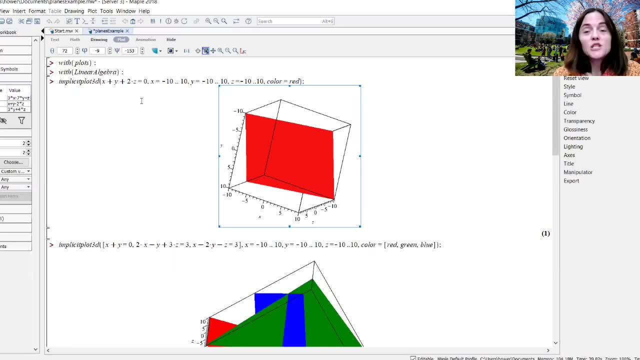 and this wasn't one of the examples we did, but i'm just showing geometrically what is one equation, one linear equation with three variables. so what i have is x plus two y, excuse me, x plus y plus two z equals zero. and i have this graph and it's in red. you see here, this is a plane in r3, okay, so 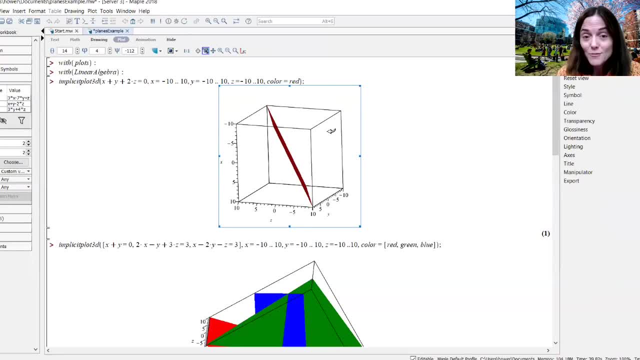 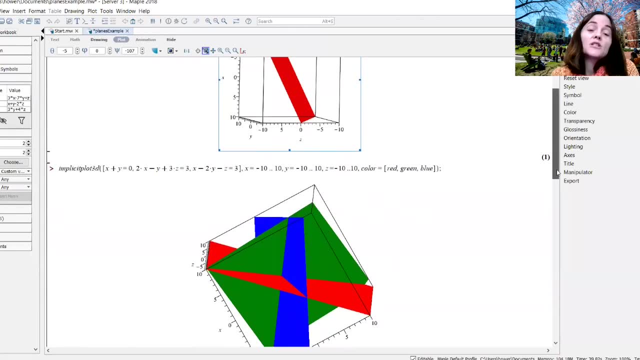 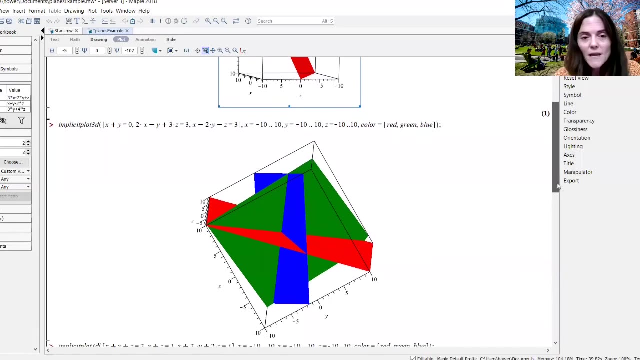 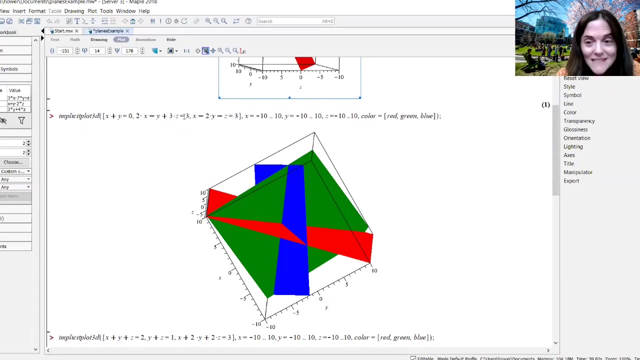 this is general. if you have a linear equation with three unknowns, it's a plane like this. well, now let's start looking at at geometrically the the solutions that we have here. so we have three equations with three unknowns, linear equations. of course, this is the very first one we did: x plus y is zero, two, x minus y plus three, z is three. 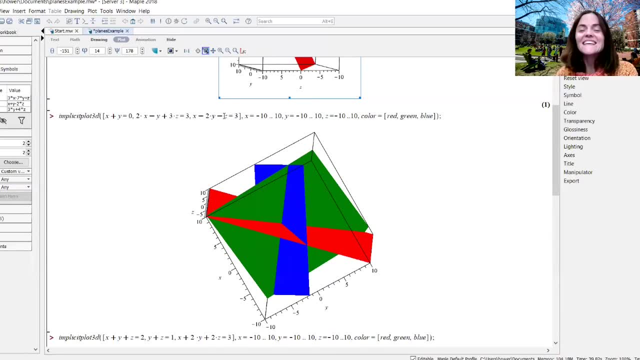 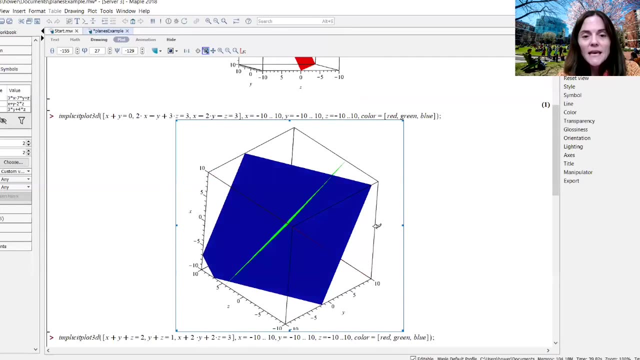 and then x minus two, y minus z is three. okay, we found it had a unique solution. how do you see that geometrically? and it is right here. it's quite beautiful. what do we see? well, well, each plane is colored with a different color. so the solutions to just one linear equation, as i 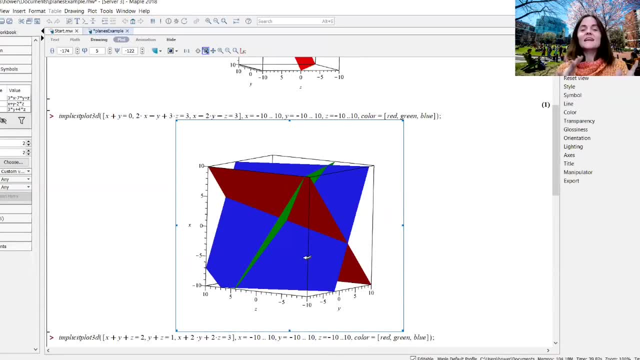 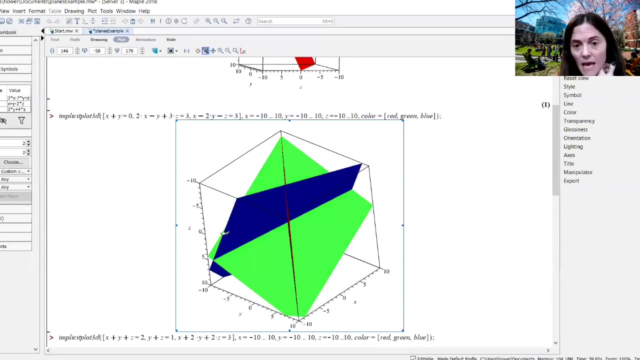 mentioned, it's a plane. each one is a different color and if you are a solution to all three, it's the intersection. just like for for two, we looked at the intersection of two lines, but here, if you take three planes and you intersect them, if you can see in this picture, what you are getting is: 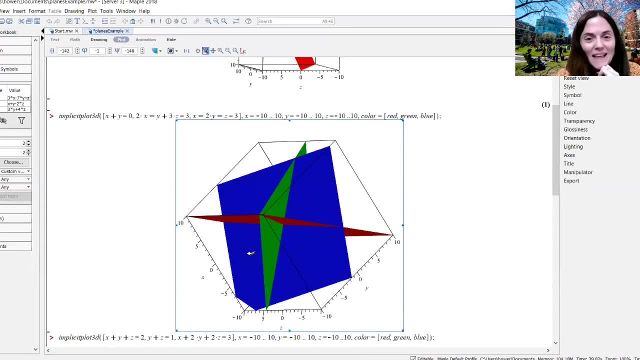 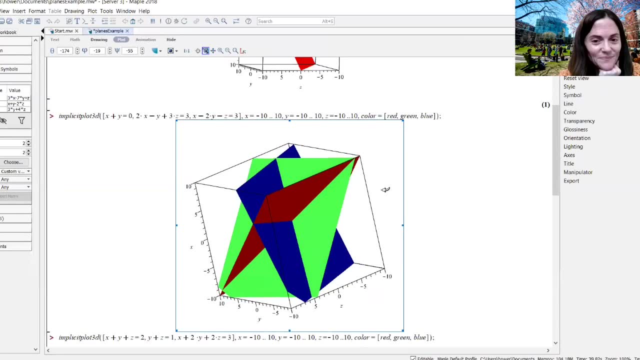 a single point. the intersection of all three planes is a single point. this is when we had a unique solution. this was our very first example. now let's move down. the second example was also a unique solution. i won't look at that. let's look at the third and the fourth in the third. 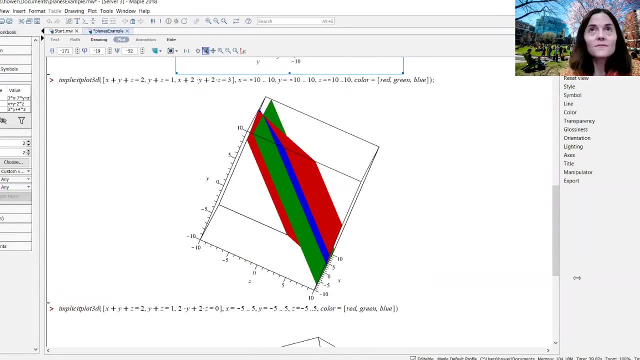 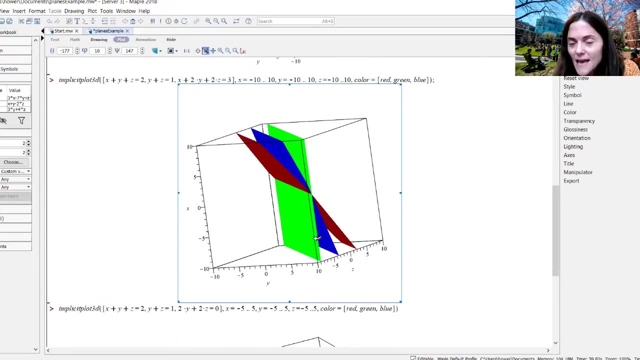 we had a whole line worth of of of solutions. now let me- oh, okay, we can see that again. it pretty well here. do you see this? what's happening is looks kind of like a book that's open with the pages coming down, but you see, these three planes? they. 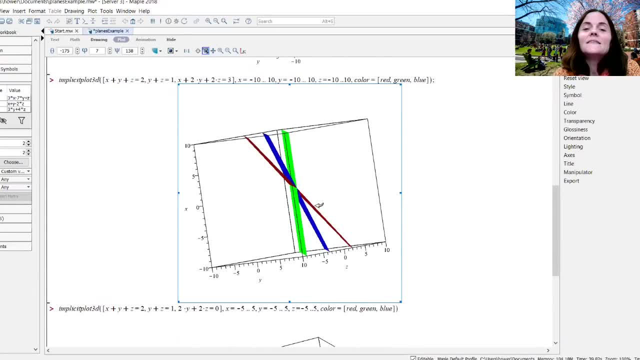 share a line in common. you see it right, it's very pretty. this is one way planes can intersect, so you can- and these are distinct planes. you could also have just two planes that are identical and then a third cutting them, something like this, or you can have all three planes identical. I guess in that case you would. 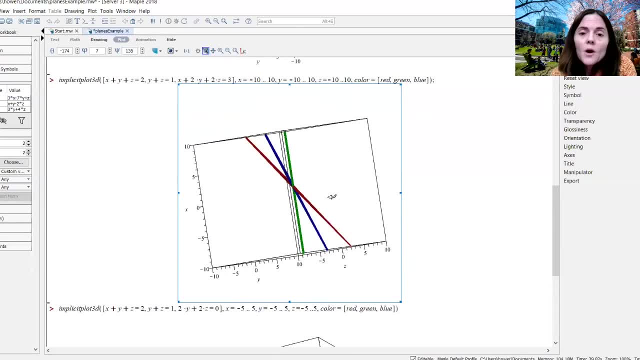 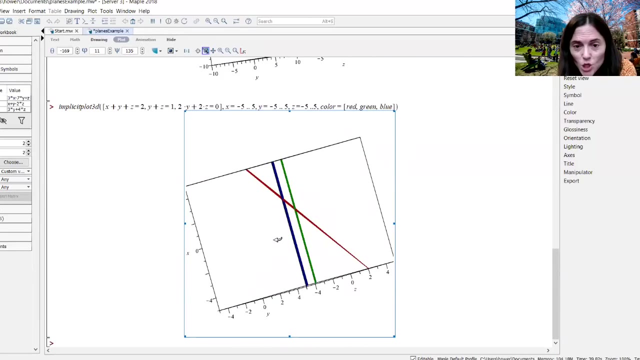 have a whole planes worth of solutions. but here we have three different planes. their intersection is a line as we see in this picture. and then finally, the. we did one where we had no solutions. let me see if I can go to good angle here. oh, something like this: two of the planes in this case are our parallel. 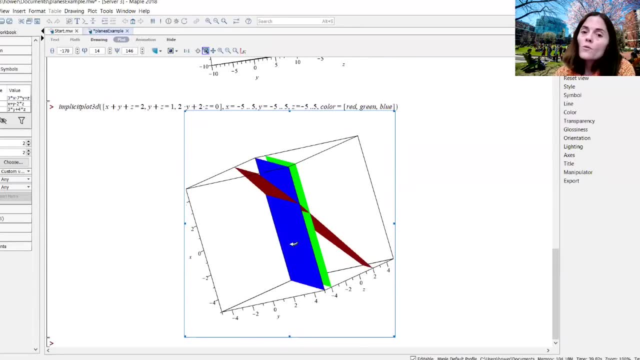 okay, and then this third cuts through them both, but but common to all three, there's no intersection. okay, when we tried to solve, we got like zero was equal to some nonzero number and of course that means we have no solutions. so this is geometrically well. this is another way that planes can't intersect as we. 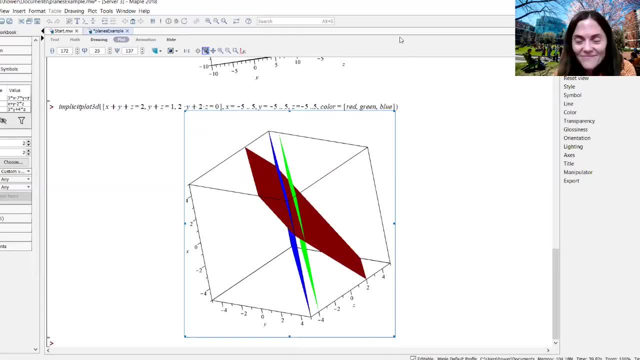 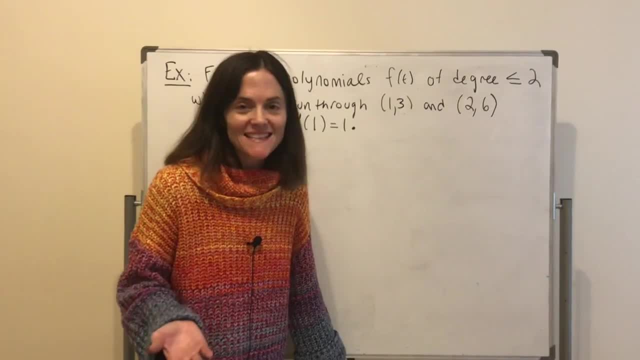 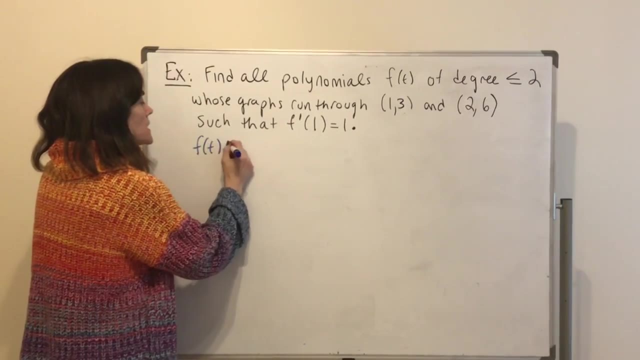 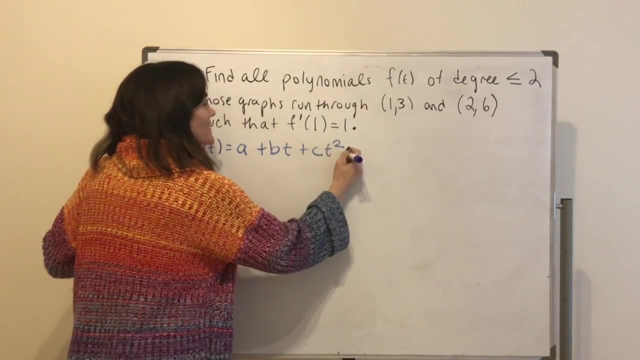 see, looking at this picture, let's close with this example, and it's a little bit different, but it's a nice application of a linear system. we want to find all polynomials. maybe I should write that f of T is of the form a plus B, T plus C, T squared like this, we want to find: well, this is a general. 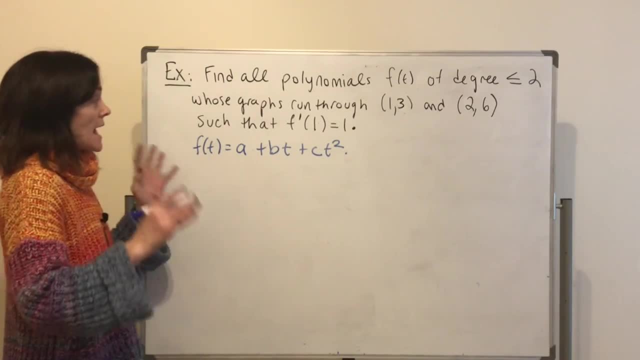 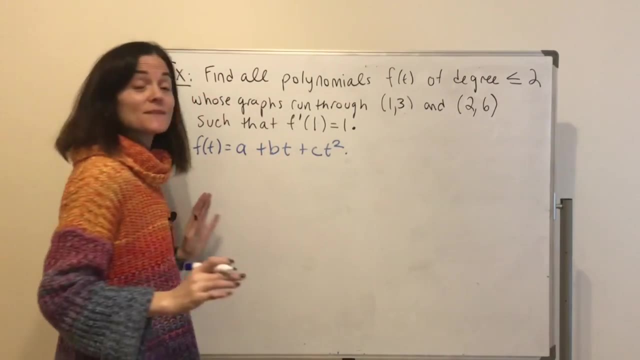 polynomial of degree less than or equal to 2. and then we have this information: the graph needs to go through this. and then we have this information: the graph needs to go through this point, this point, and then we know something about the derivative. well, first of all, what this is going to lead to, I should say we will. 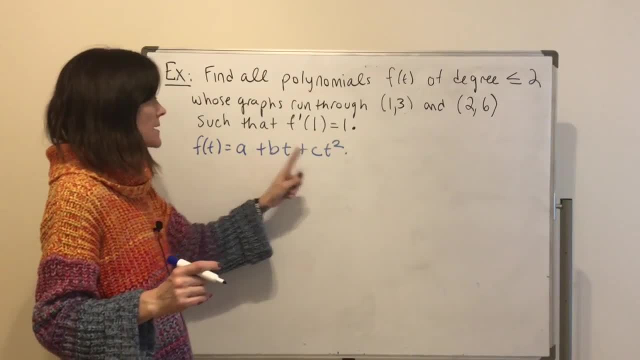 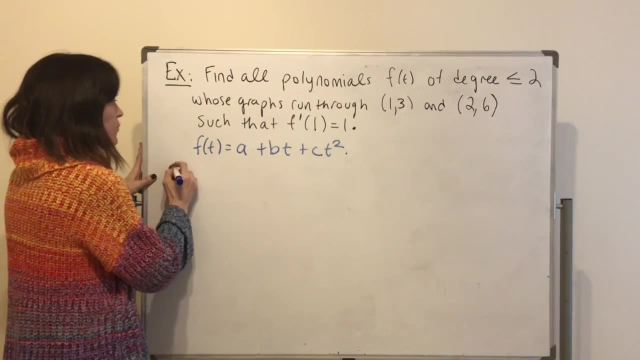 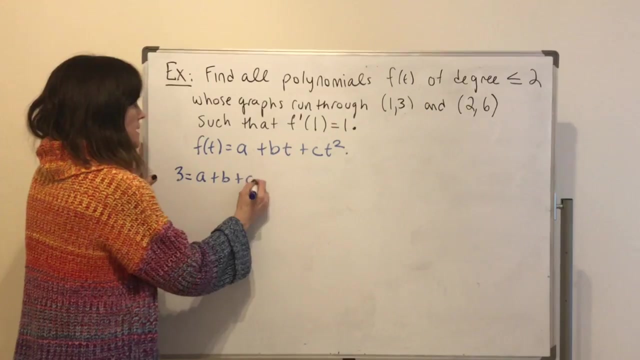 have a linear system involving a, B and C, and then we will solve this linear system. okay, well, what we know is that f of 1 should be 3, so 3 should be a plus B plus C. that's evaluating at 1, and then, right, maybe I should make. 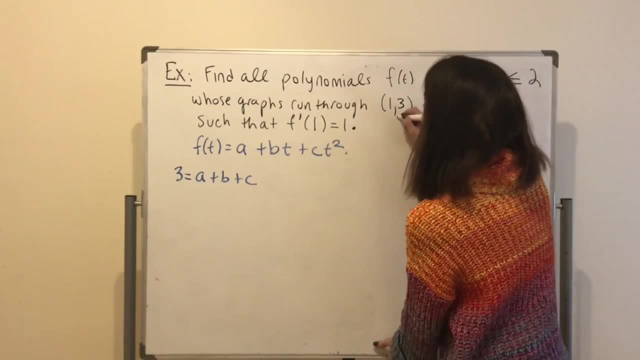 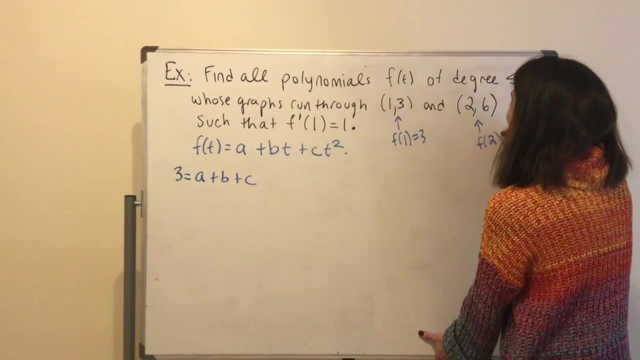 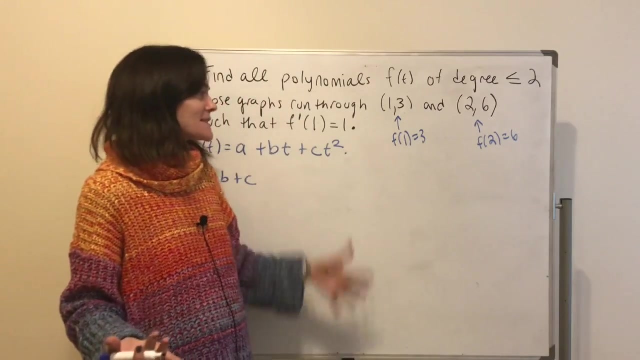 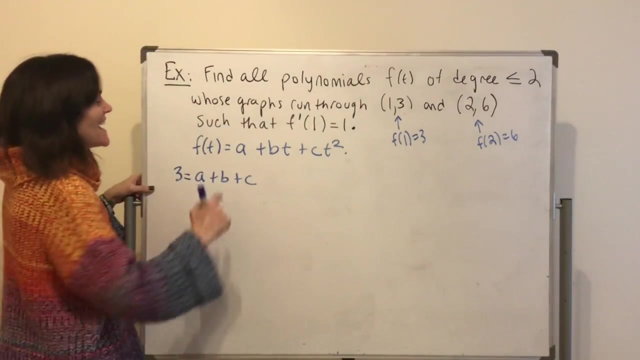 this observation here: this says f of 1 equals 3 and this says f of 2 equals 6. right at the point: 1 comma 3 is on the graph, then f of 1 is 3, like this: or if 2 comma 6 is on the graph, f of 2 is 6. okay, we have that down. and then now let's get. 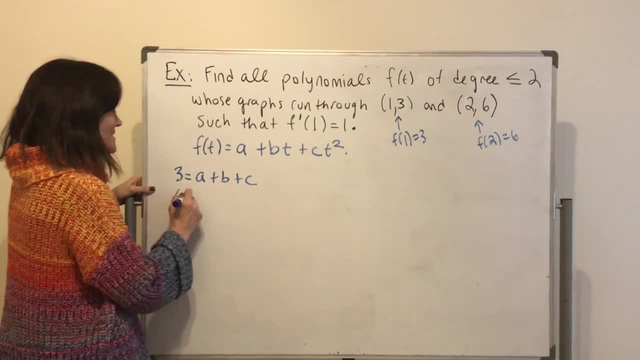 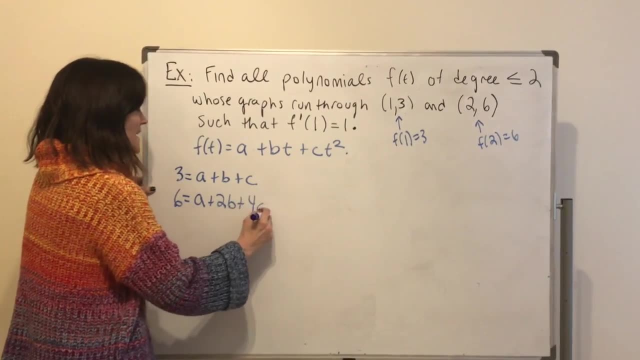 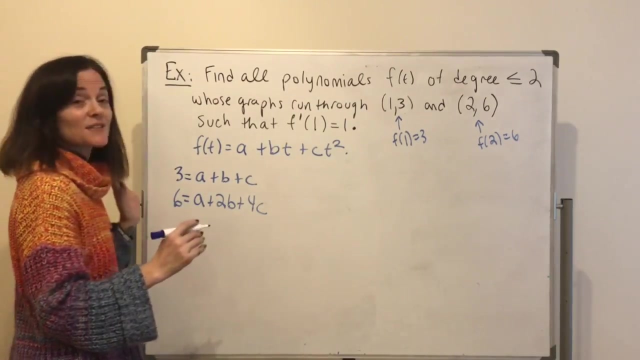 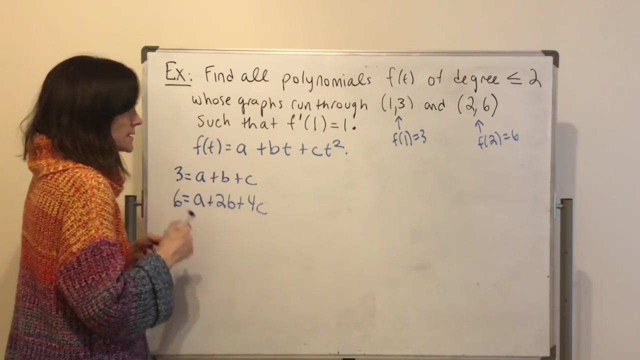 this second equation: f of 2 is 6 says 6 is evaluate at 2 a plus 2 B plus 4 C. so far so good. well, there's this third equation about the derivative. this is the derivative. the derivative at 1 should be 1, so here, maybe I should come over here and take the derivative, okay, so. 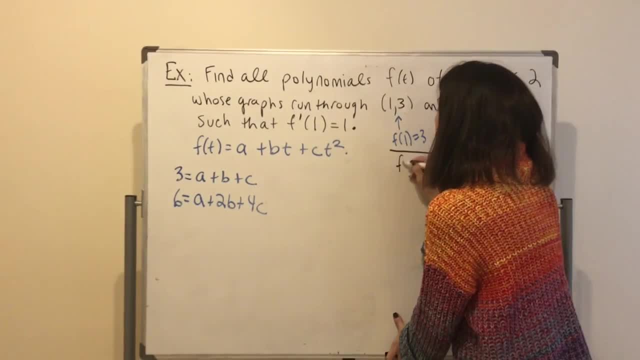 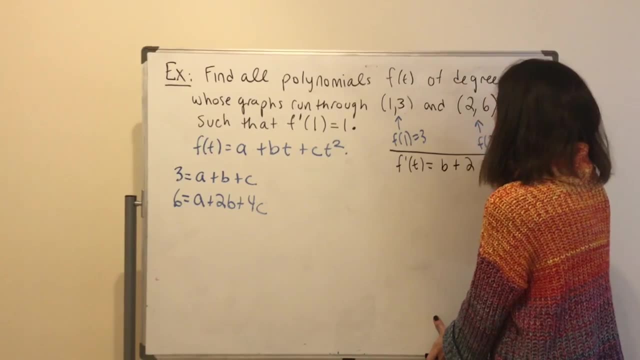 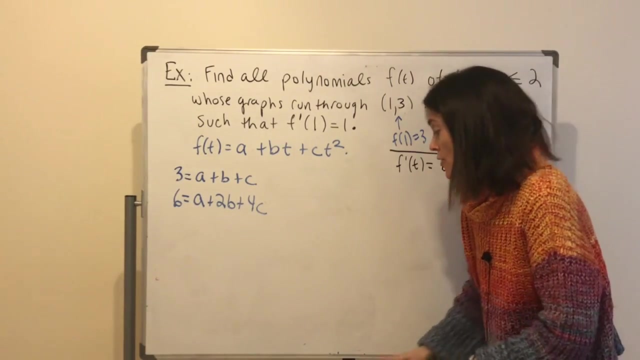 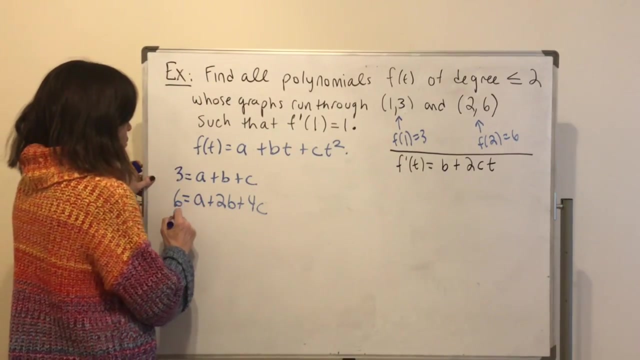 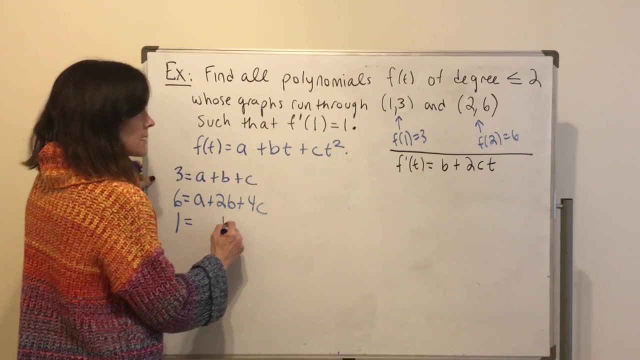 this is my function. then f prime of T. well, this is polynomial. it's B plus 2 C, T. okay, now evaluate this at 1. this is going to give our third equation. evaluate that at 1. we should have f. prime of 1 is 1, so 1 equals. well, it's going to be 0 a, and then we will have B plus 2 C. 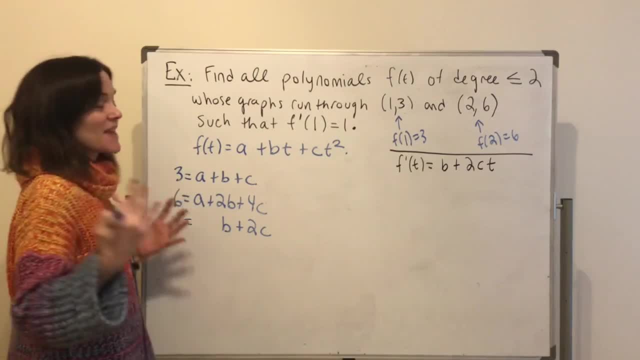 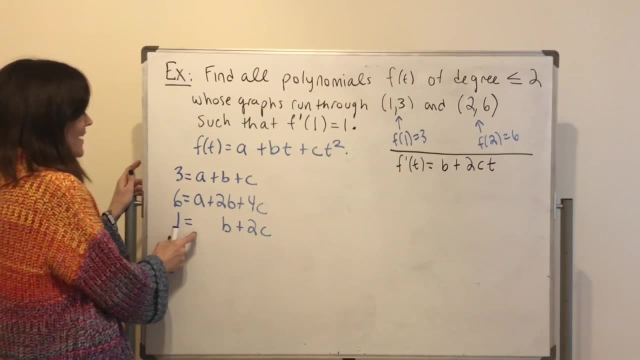 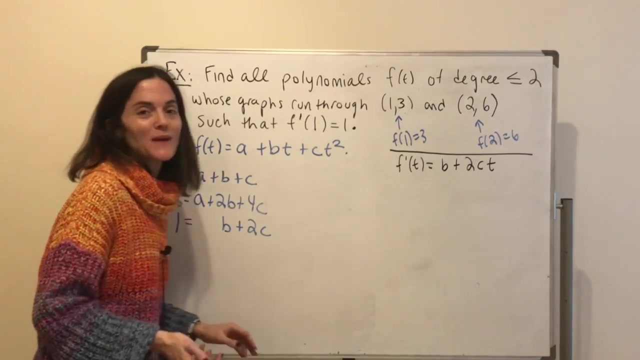 okay. well, the only difference is, instead of having X, Y and Z, I have a, B and C, and then I put the constant parts on the left-hand side versus the right-hand side. this is the only thing that's changed, but it's exactly the same as we. 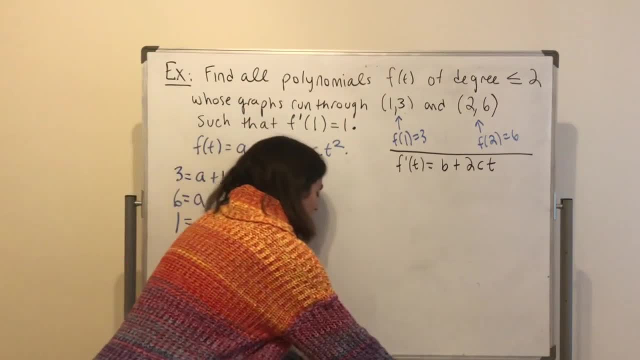 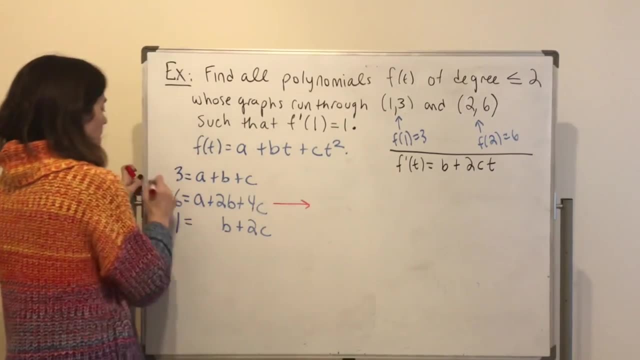 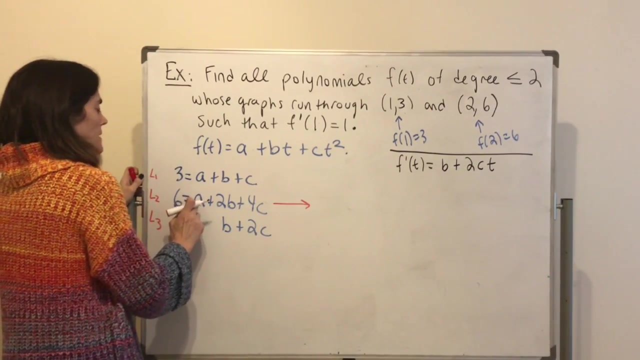 have been working with. okay. so what am I going to do? well, first I want to eliminate the a, so I will take again. this will be line 1, line 2, line 3, line 3. okay, so I'm going to take- let's see minus 1, line 1. add it to line 2. 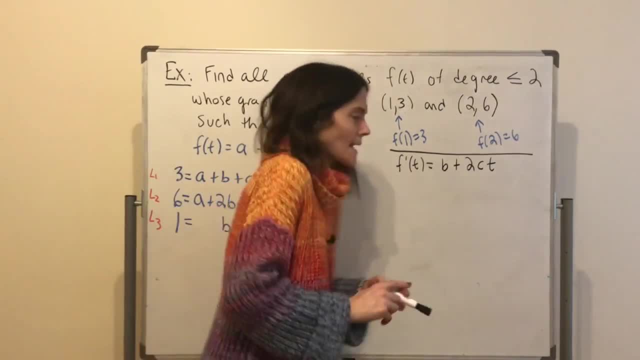 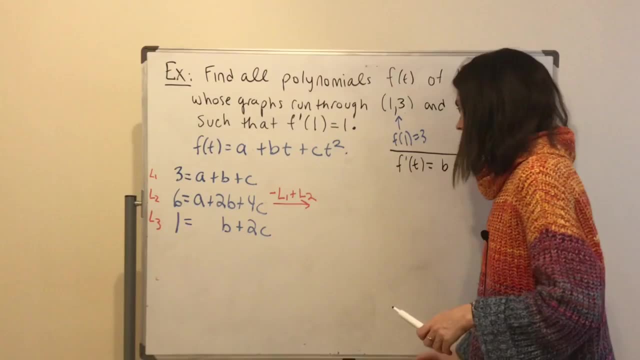 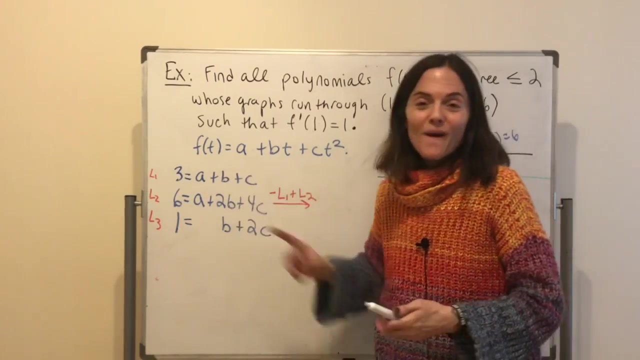 okay, and maybe just, I guess, so that it matches, I'm going to put the three, six and one on the other side of the equal so that it matches exactly what we were doing before. maybe I should, okay, but this was sort of the new part, the setup. so we have, oh, I, 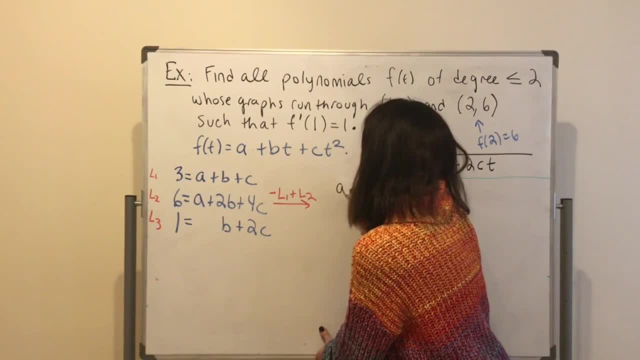 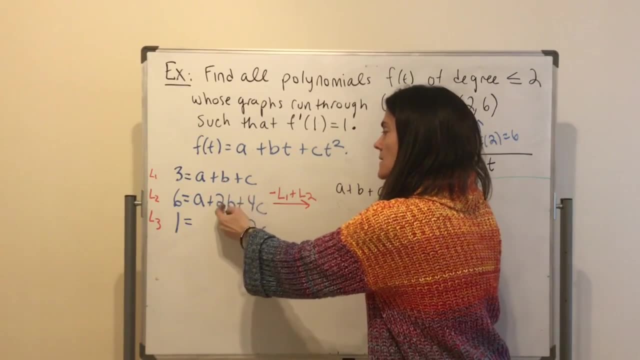 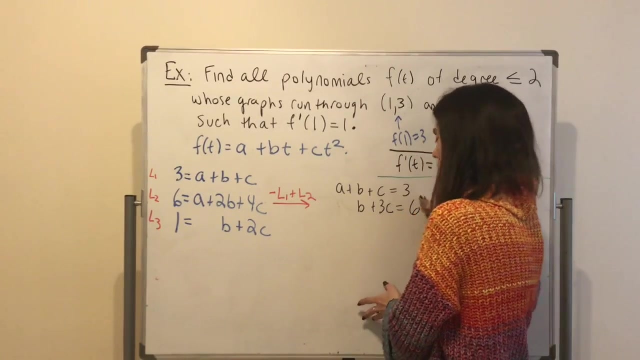 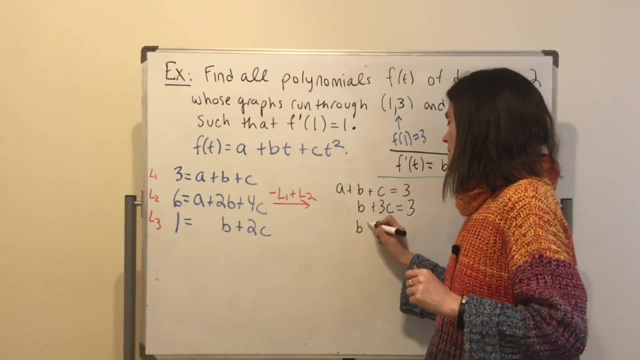 was going to put. on the other side we have a plus B plus C is 3, and then we are going to have: let's see, this minus this B, this minus this plus three, C is oh, six minus three, oh, it's another three. okay, then we just recopy: B plus 2, C is 1. 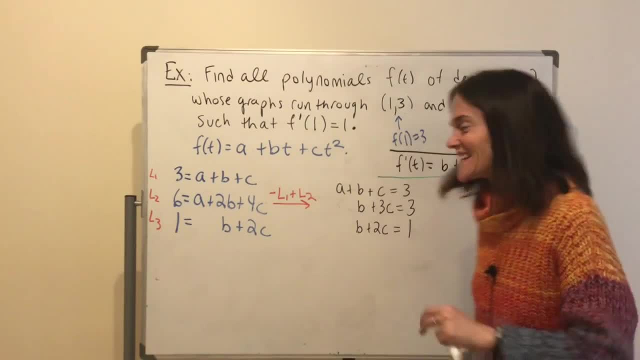 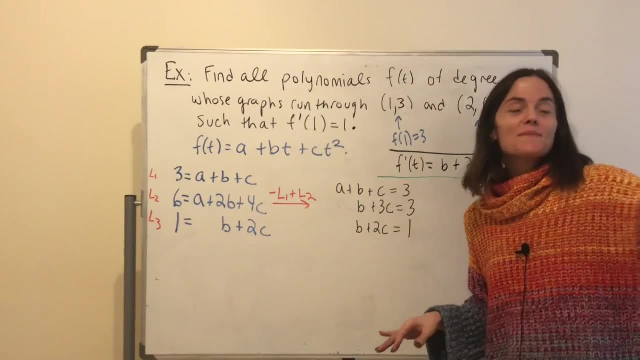 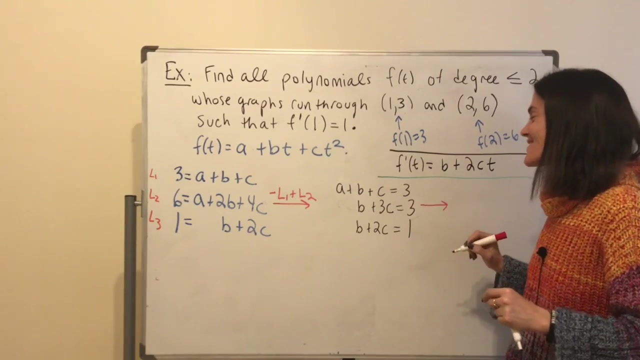 okay, I hope this is making sense. This is the hard part about doing my lectures this way. I can't. hey, is everybody okay? Well, I am in my bedroom right now. There's nobody in here but me. Okay, well, we will make it through the semester. 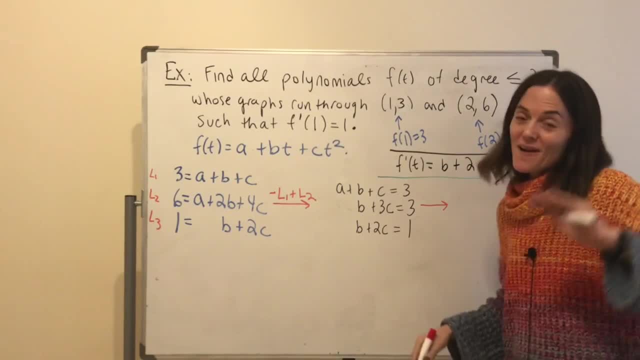 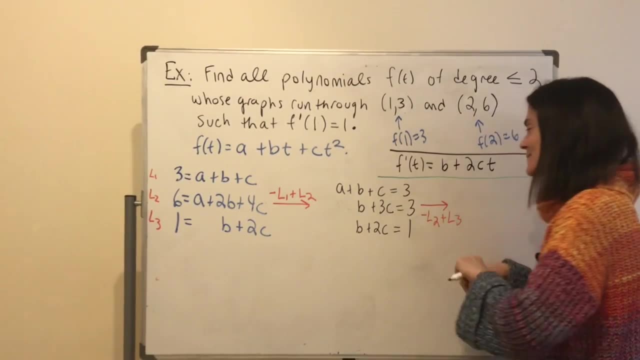 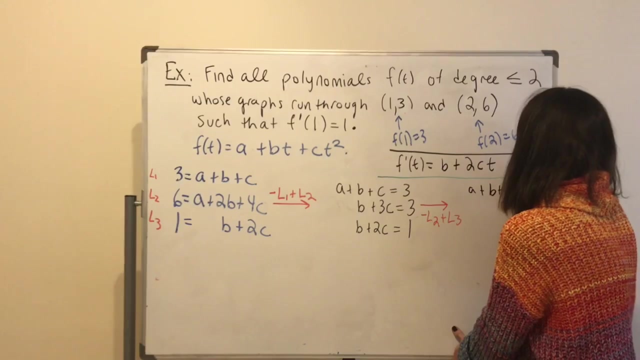 Okay, now we wanna eliminate this B so that we are able to solve for C. This will be: we will take negative line two, add it to line three. Very nice, A plus B plus C is three. Then we have this: remains B plus three, C is three. 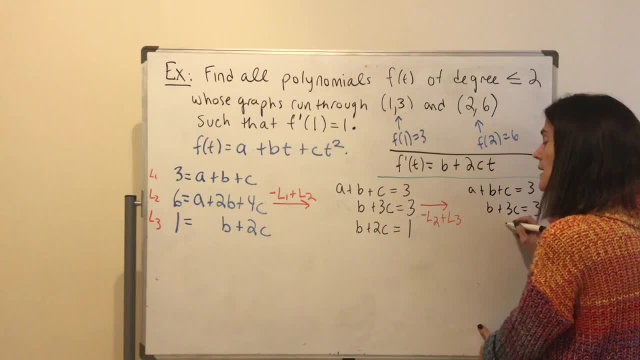 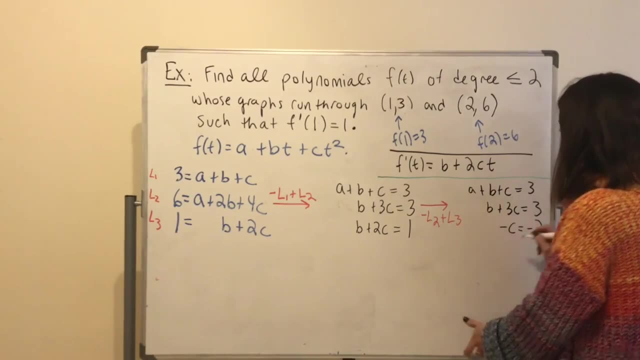 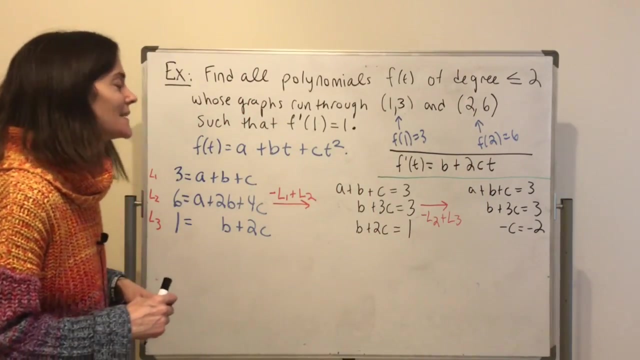 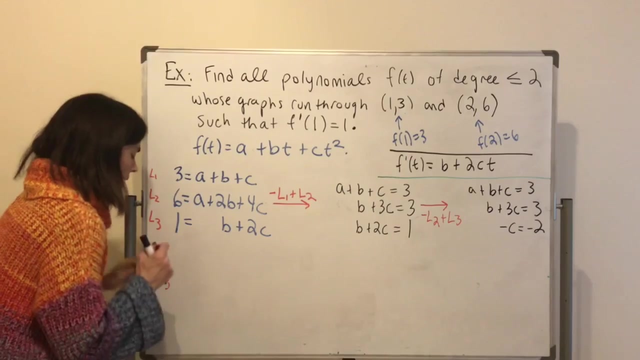 We take negative this. add it to this, which becomes negative C is negative two. Okay, so well, technically, what are we doing next? We're multiplying minus one times line three- Maybe I'll do this little here- Minus line three. 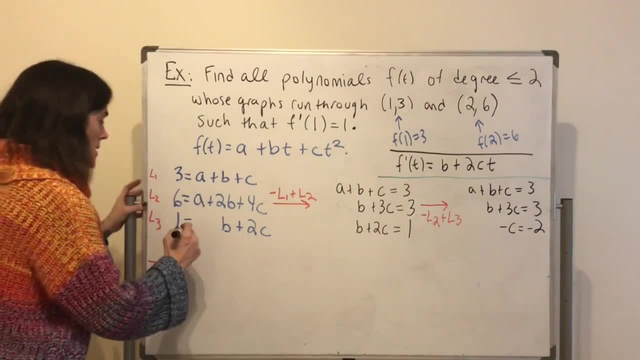 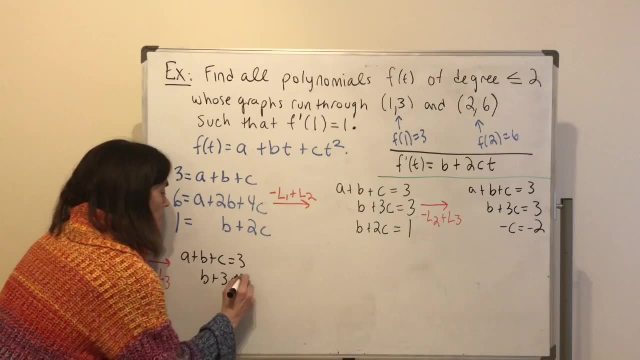 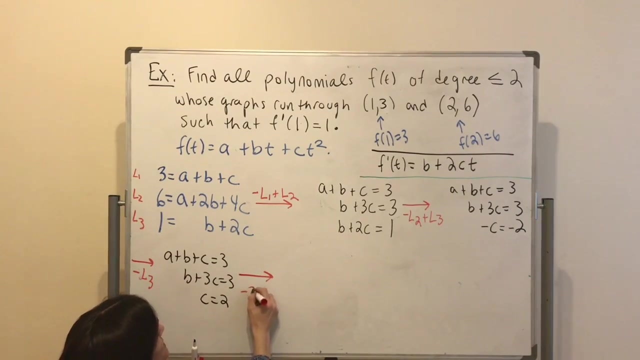 And I'll just recopy it and move directly into the next step. So this would be: A plus B plus C is three, B plus three, C is three, C is two. What am I gonna do? I'm gonna take minus three, line three. 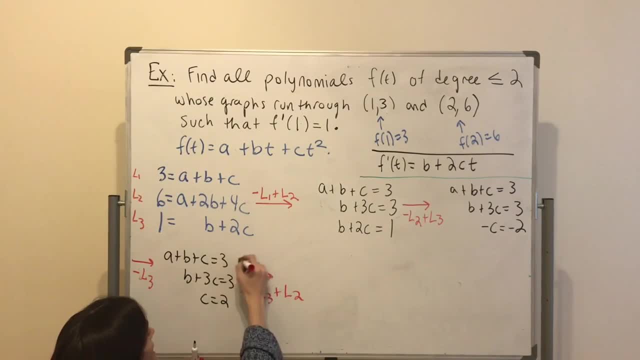 add it to line two. Just take minus three. add it to line two minus line three. add it to line one. We're almost there. So line one becomes A plus B is three minus two, which is one. Line two becomes B. I have minus three. 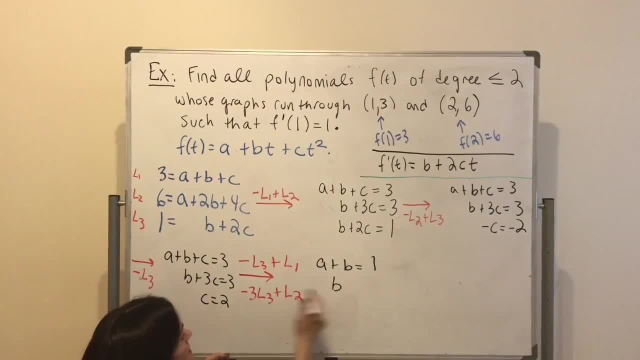 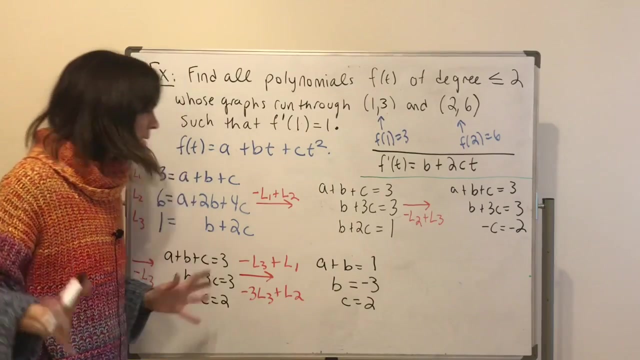 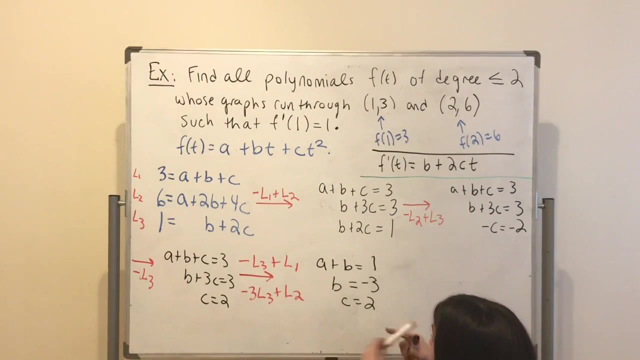 Oh, this is gonna be six. I mean three minus six. this will be negative three, And then this is still: C is two. Okay, so we have: B is minus three, C is minus two And one more step. All we need to do is our final step. 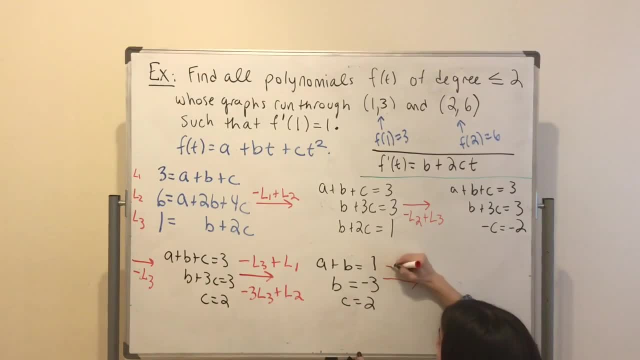 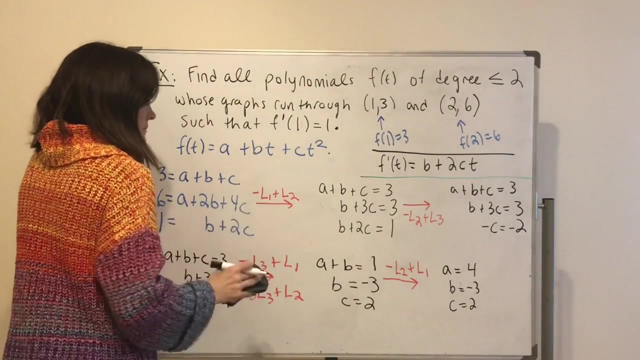 is: just: take negative line two, add it to line one, And then we get: A is Four, B is negative three, C is two. So our polynomial: now we're ready to have our final answer. Maybe I will don't know where to write it. 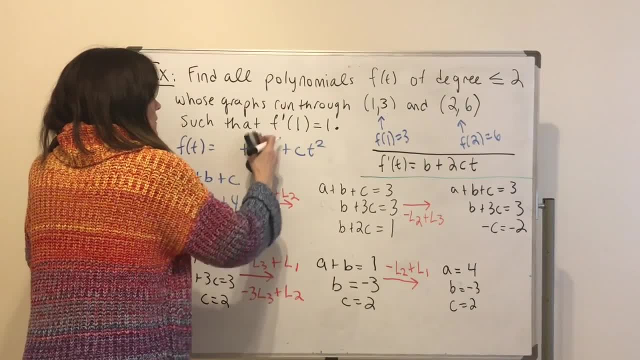 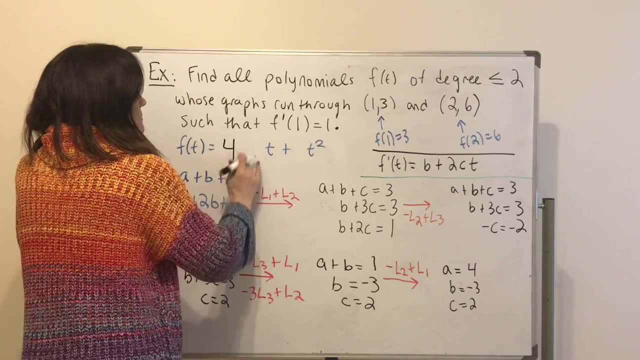 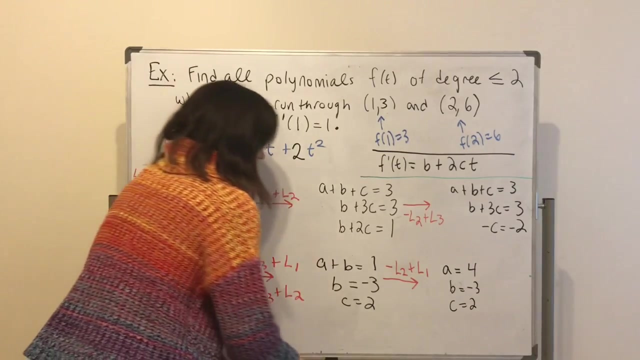 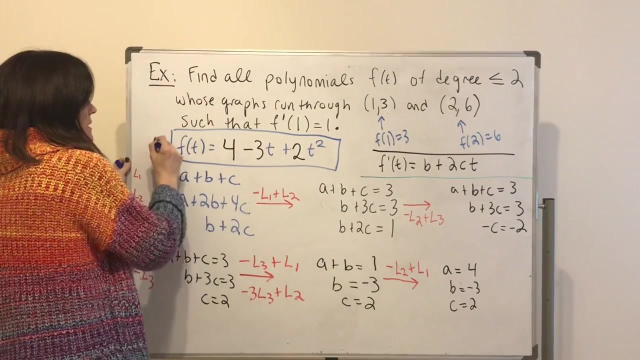 I'll just put it here. Oh, Okay, we saw, A is four, B is minus three, C is two. Find all polynomials. Well, look, there is a unique. The answer is: there is just one And here it is okay. Very nice. 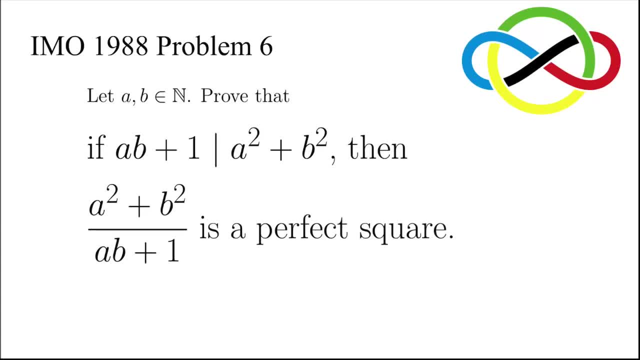 Let's take a look at this very famous problem 6 of the International Mathematical Olympiad 1988.. It says: let a and b be positive integers. prove that if a, b plus 1 divides a squared plus b squared, then a squared plus b squared over a, b plus 1 is a perfect square. Before we move on,